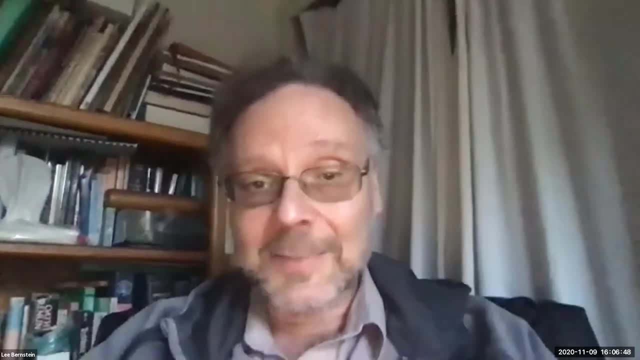 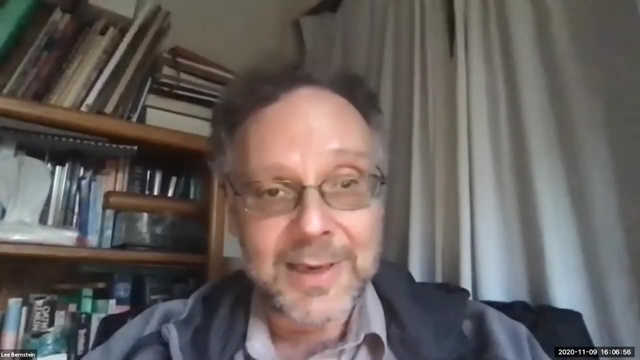 definitely the case for Etienne. So, like many of the best experimentalists, Etienne's career is rooted in practical experience. Starting with an undergraduate background in chemistry, he became involved in isotope production at Itemba Labs in South Africa, becoming the targetry and 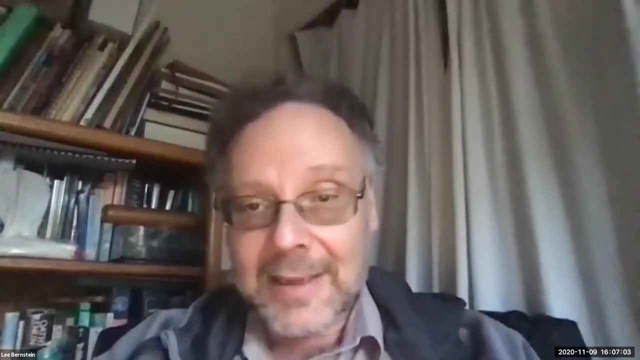 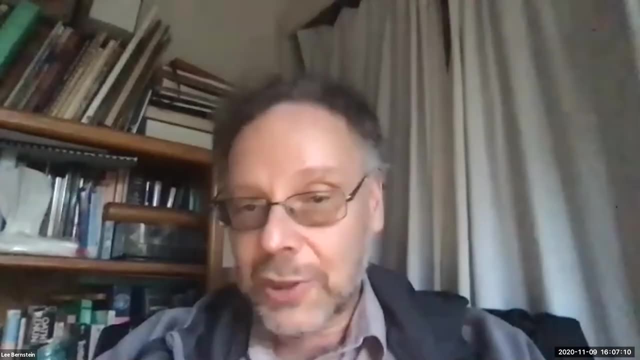 bombardments coordinator for five years. After getting this excellent and practical background in this really multivariate field, Etienne decided to get a PhD, Graduating from Stellenbosch in 2014,, with a dissertation titled Production of Radionuclides with Medium Energy Protons. 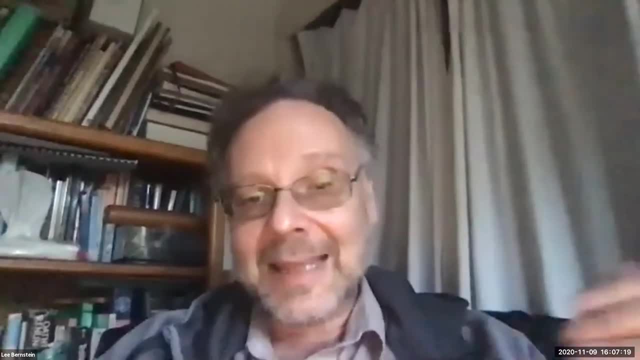 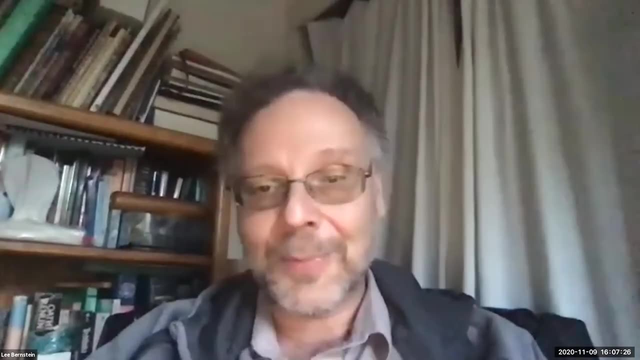 with the emphasis on targetry. So after getting that degree, Etienne crossed the equator and went to PSI in Switzerland for three years, where he gave the CERN isotope production capability a shot in the arm, with a focus on the production of radiolanthanides including terbium-161.. 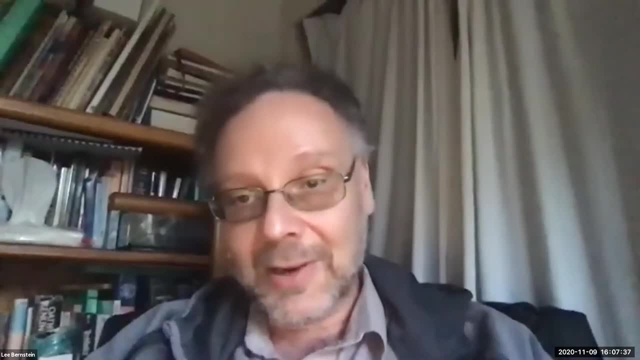 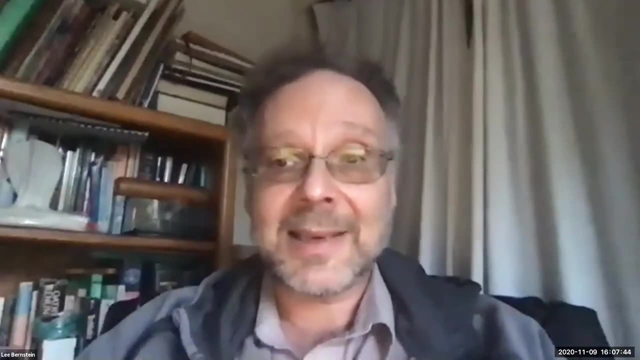 And then, to the great and good fortune of the US isotope production community, Etienne decided to stay north of the equator and move to Los Angeles, where he was a professor at the University of Los Alamos National Lab in 2017, to become a senior scientist and the lead physicist for 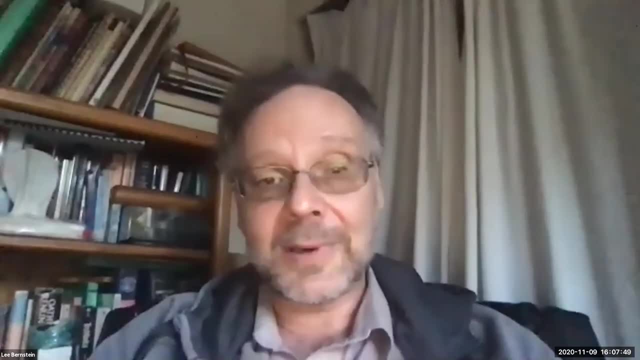 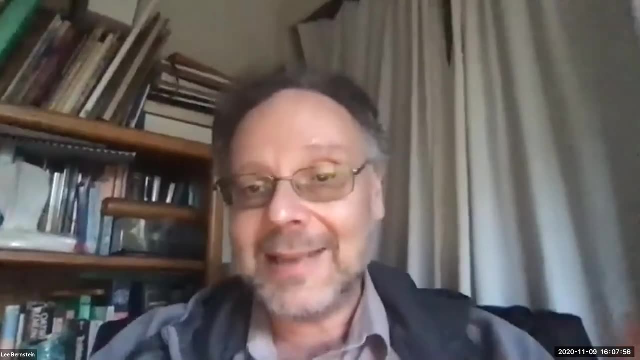 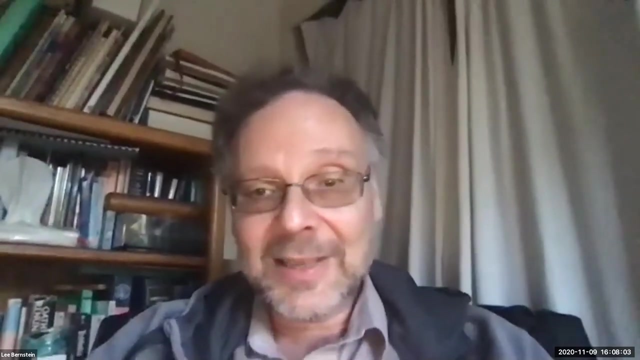 isotope production at the IPF, the isotope production facility at Lance. So I think of it as, to use a military analogy. Etienne was like a senior NCO who went on to become an officer and then finally a general. That's really the best generals you can get. So for the past years, 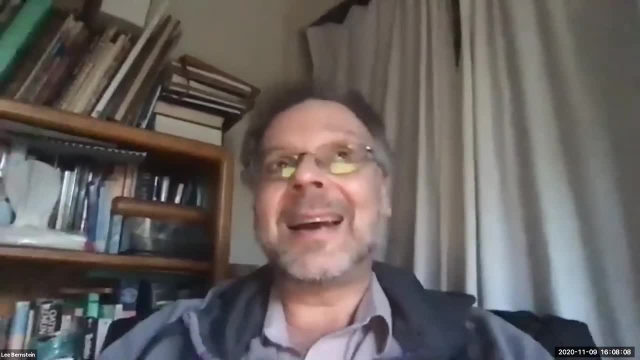 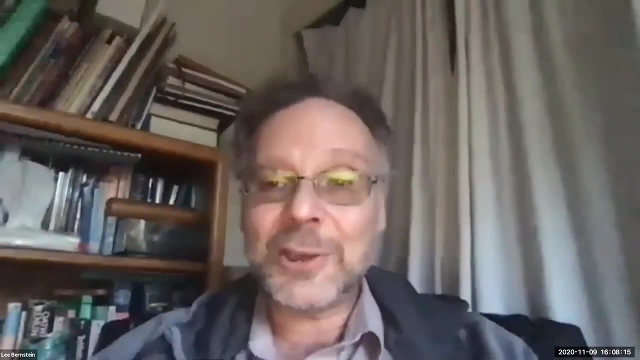 Etienne's been my principal collaborator in something that a term that he came up with, we call it yet-on-the-spot, And he's been doing a lot of research on this and he's been doing a lot of another tri-lab collaboration, Yahtzee. This tri-laboratory effort is between Los Alamos. 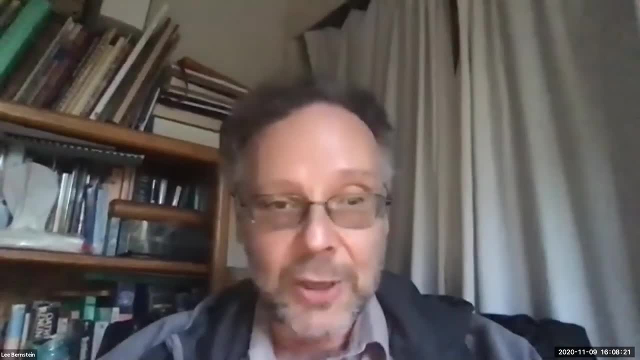 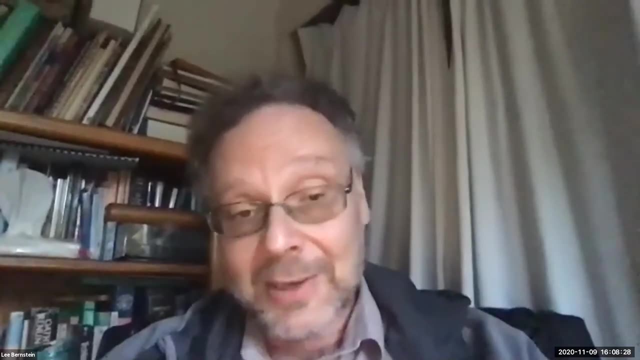 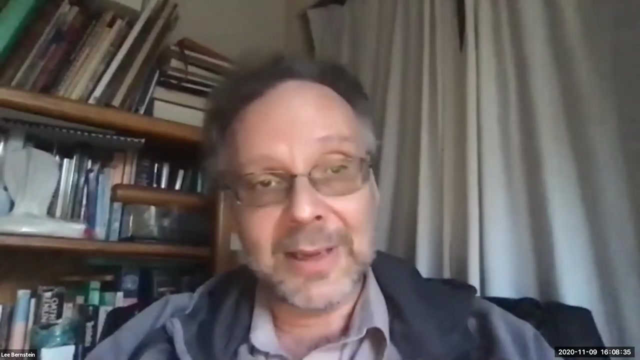 Brookhaven and Berkeley to improve nuclear data for isotope production, And he's helped train several of the GSRs in my group and that really shows that he's as good at mentoring as he is at target design. So please join me today in welcoming my colleague and friend, Dr Etienne Vermeulen. 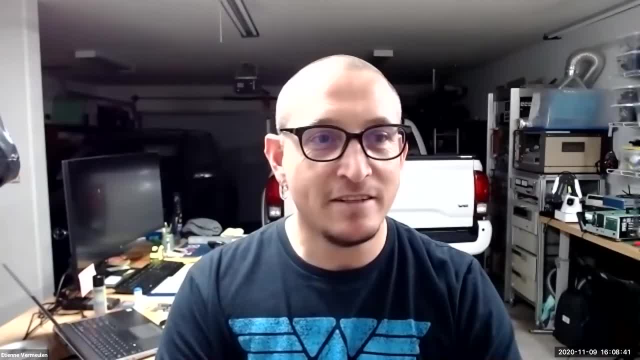 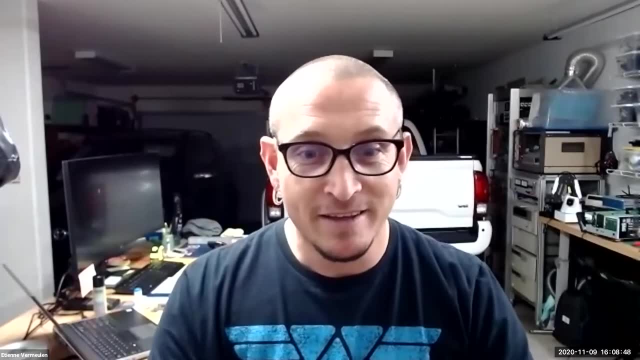 Thank you, Lee, That was a very flattering interaction. And hi everybody from a snowy Los Alamos. So behind that door, behind me, it is actually snowing right now. Winter seems to have come early to Los Alamos, And it's ironic because I 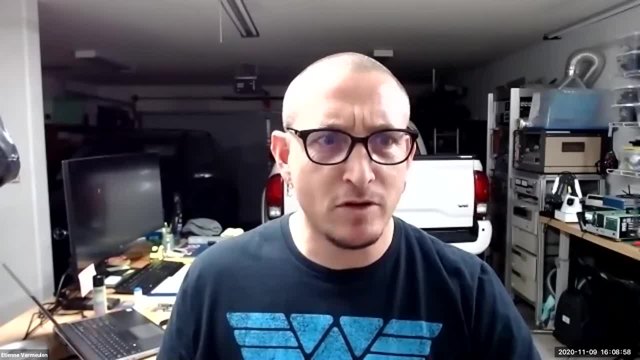 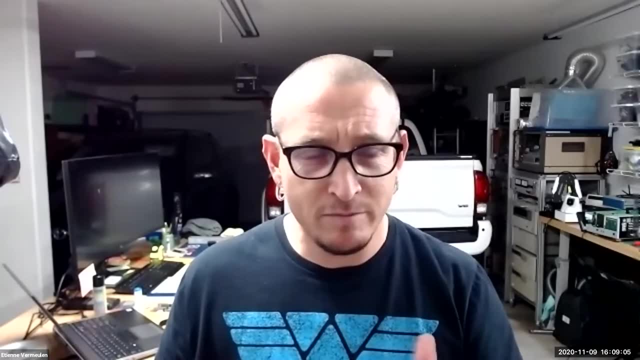 just bought the first Game of Thrones book at the guy's shop because he's got a shop down in Santa Fe Not signed because you know that's expensive. But winter is coming, That's the best I can say about that. 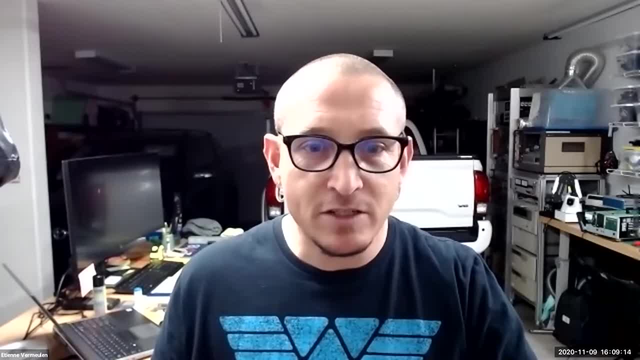 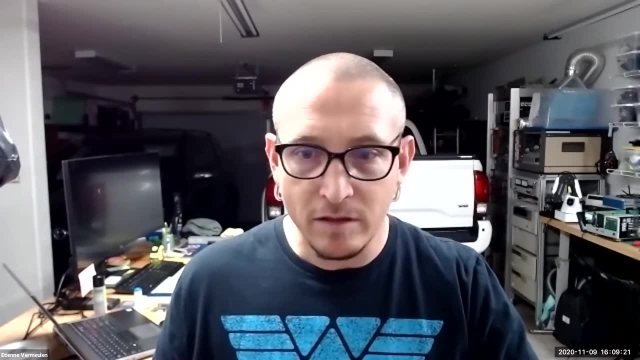 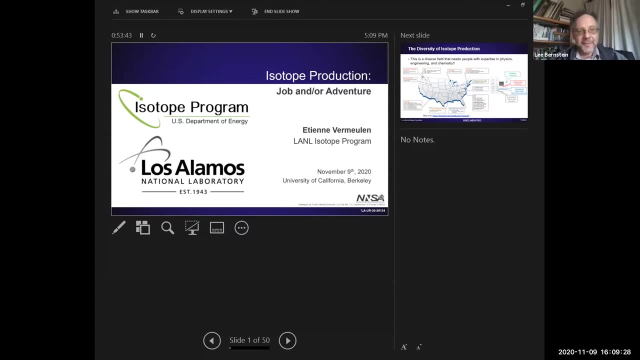 Okay, let me see if I can get my screen share going here And then we'll get started. Okay, Lee, can you confirm You can see my screen? I can confirm You're in. you are in presenter mode, So if you want to do slideshow, 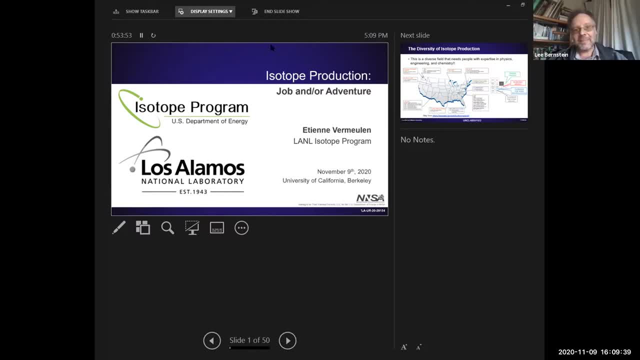 I don't know if you could do display settings. Perhaps there's a way to change it. Yeah, there's a way to do that. How's that? No, still presenter mode. I mean, it's visible, but it's presenter mode. 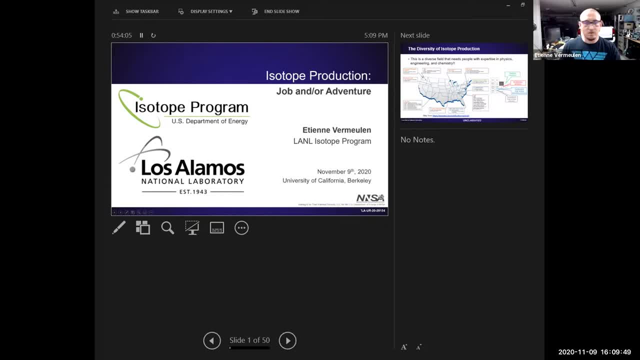 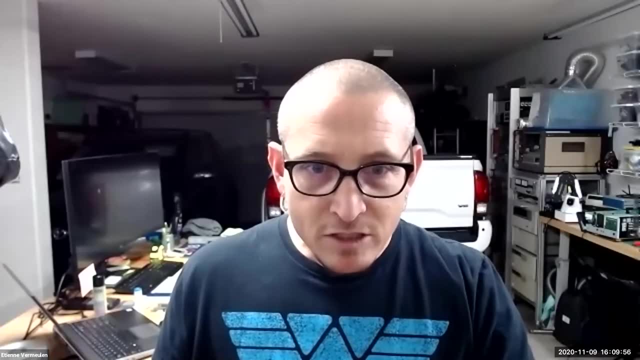 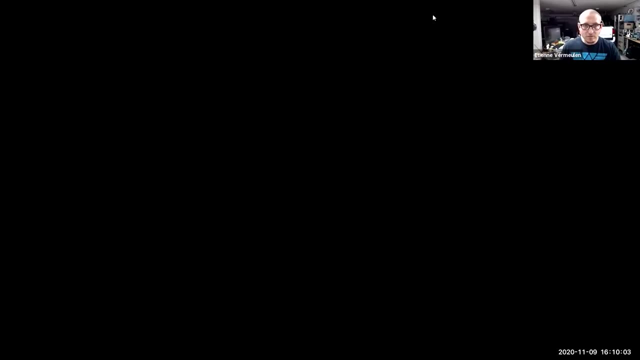 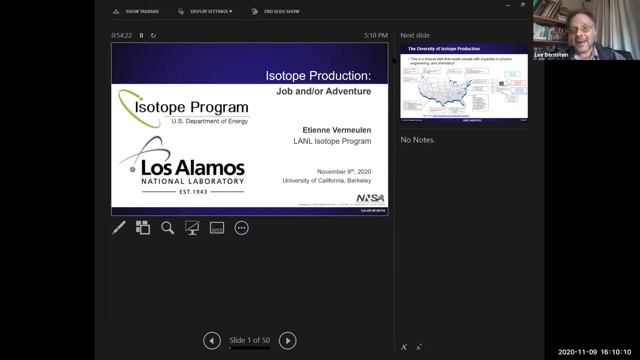 No, How? Presenter mode still? No, he's not doing that. Okay, But I've got technical difficulties. It may mean I'm not sharing the right screen. Let's see. How about this guy Still? Still presenter mode? I mean it's. I think it's okay. But 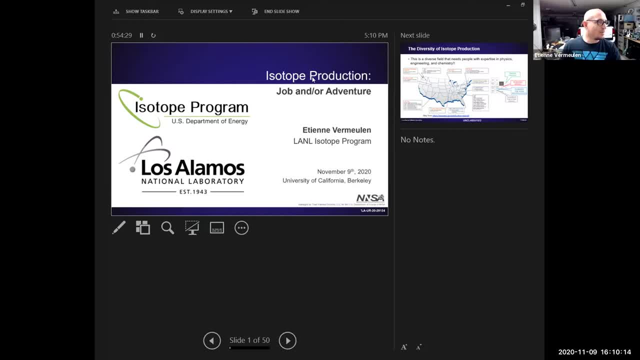 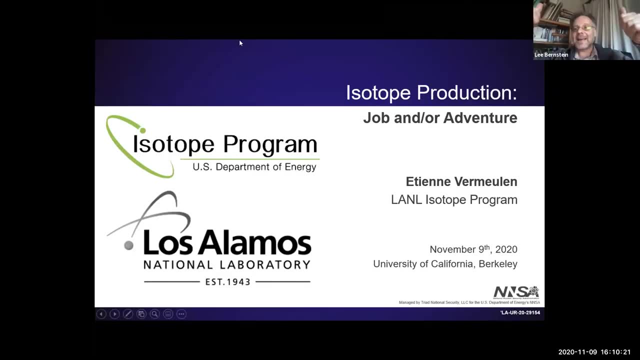 There's anything you want to add. I don't want you guys to see all my your interesting notes. Interesting notes, Etienne. I think there's a swap screen somewhere. There you go, You're good, That's it. Okay, I have two screens. That's why I get confused. 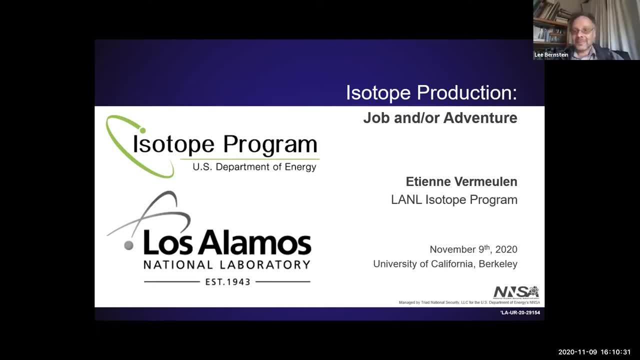 Alright, that's fine. Okay, Well, so I titled this job and or adventure, but but it's pretty much just adventure. I've done this now on four different continents and it is pretty much an adventure. It's a stressful adventure at some. 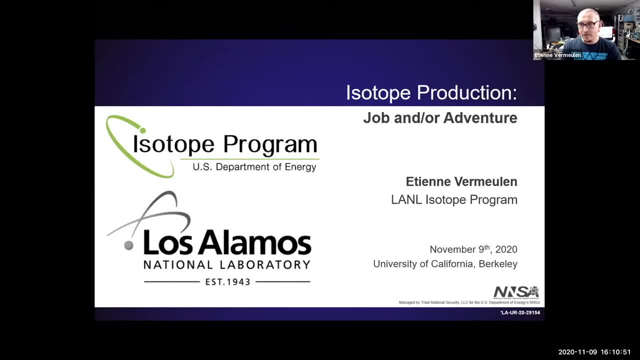 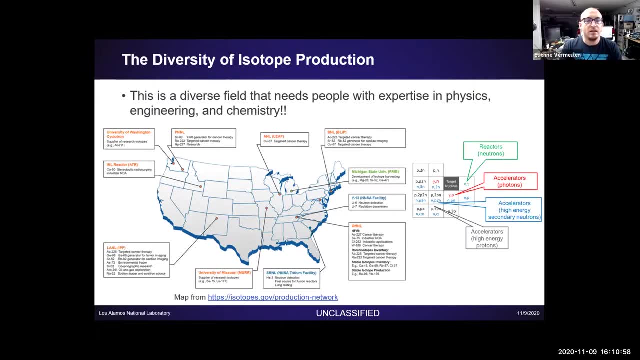 point, but still an adventure. So I just want to start with how diverse isotope production is in the United States. These are all the laboratories and some of the universities that are currently in the DOE. isotope programs fold, So all of these facilities either create 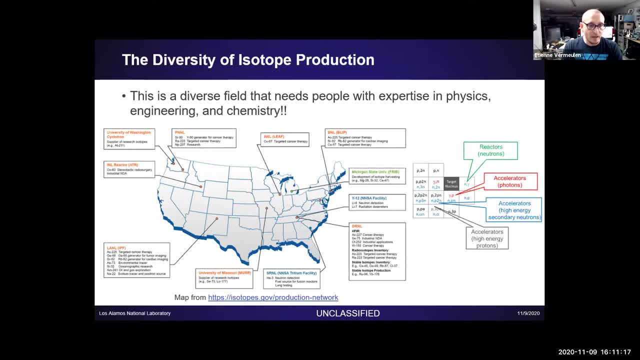 or use isotopes, and if you look through the list, it's pretty much everything in the nucleotide chart that you can think of is made in the US and is used in the US. We use reactors, accelerators of electrons, of protons and even some heavy ions, specifically alpha particles, and then sometimes lithium-7 and 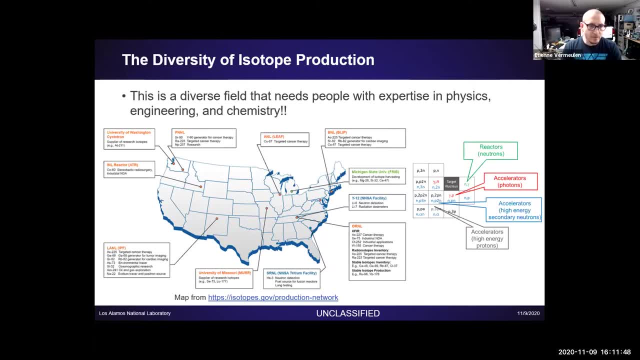 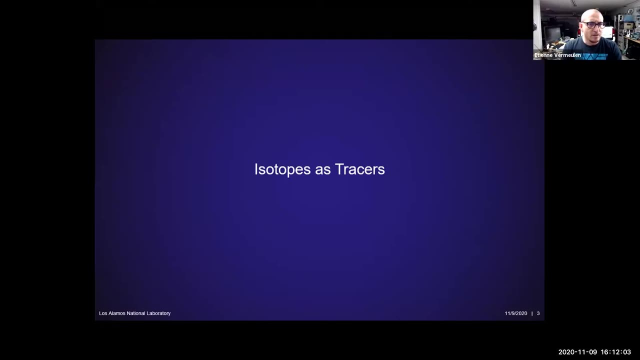 I'll talk about that a bit later- and then the stuff that I do, which is protons. so Lee will get a good laugh when I tell you I'm mostly a proton guy and neutrons come as a bonus, but mostly what I work on is proton accelerators. so the first thing I want to sort of touch on 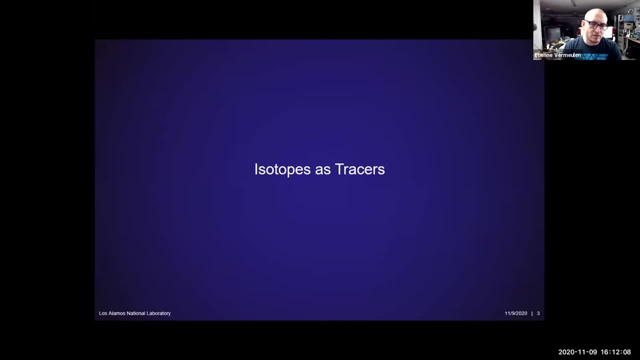 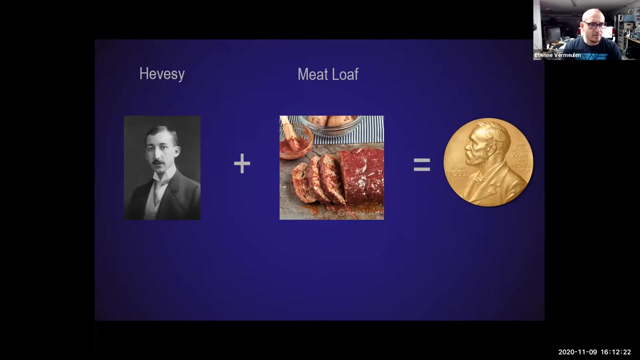 is the use of isotopes as tracers, because also what I do for the most part is make medical tracers and it's quite an interesting story where it started. so George Heversy got the Nobel Prize for inventing isotopes as tracers and the way he did this he was. 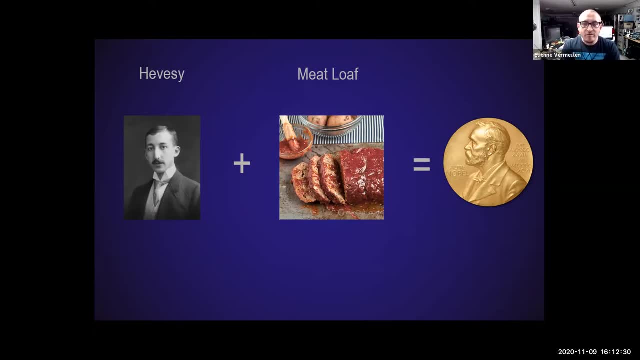 working at Munich at the time and he was convinced that his landlady was re-using the previous week's food in the Sunday meatloaf. so he got some radioactive material from his lab and surreptitiously spiked the meat, probably on wednesday, and on sunday used the detector. 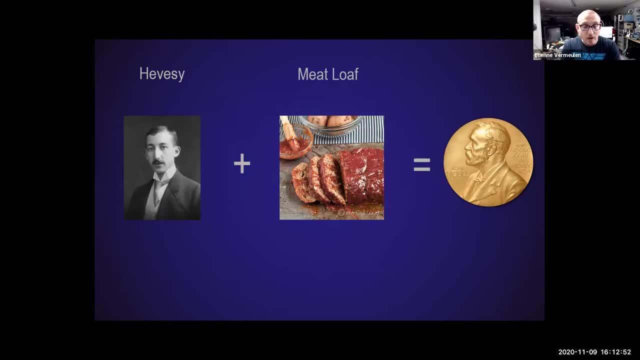 that he built himself to prove that this lady was actually spiking the food or was actually re-using the meat. ladies that are working all over the world. the world has another amazing approach and we have this one of 250 actual results that are actually putting food in in sunday's meatloaf. and he got the nobel prize in chemistry, i think, for inventing um the. 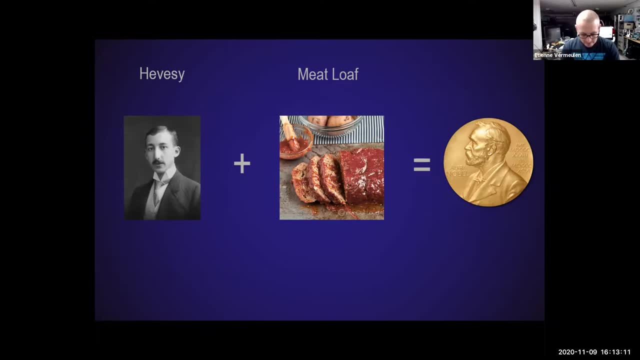 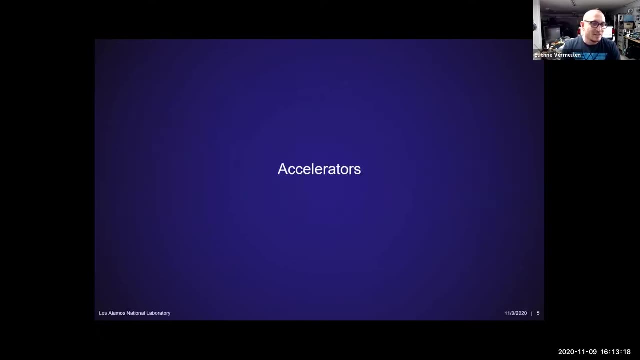 tracers. so that's sort of where it started, and, uh, it's a pretty good start. if you're going on an adventure, you can't do it on an empty stomach, right? so, as i said, um accelerators make up most of what i do, and mostly proton accelerators. 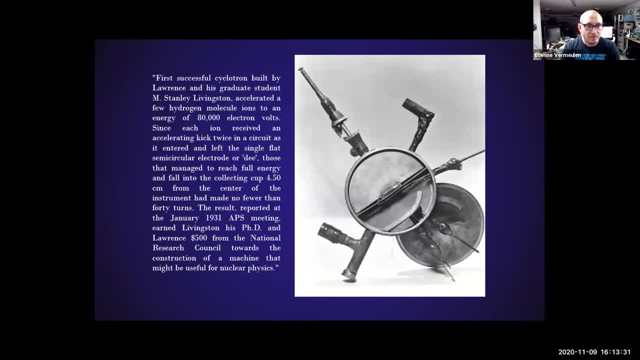 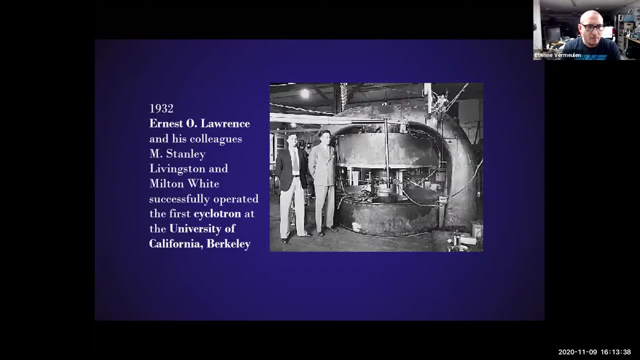 now- you guys probably know this by now. this is the first cyclotron that was invented at in berkeley and by these two guys. a lot of people think that the guy on the left probably did most of the work and the guy on the right probably did most of the work, and the guy on the right 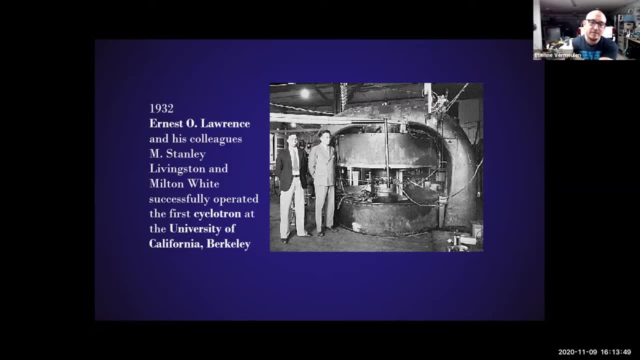 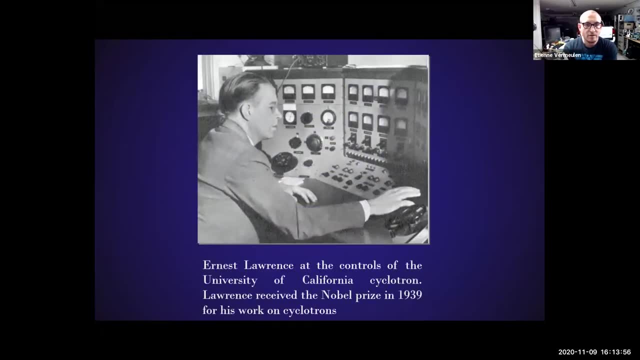 did most of the work and the guy on the right got the, got the nobel prize, um, but that's the, the magnet for the first cyclotron. that was probably just down the road from you guys. and of course, here's lawrence at the control booth, um, and i. 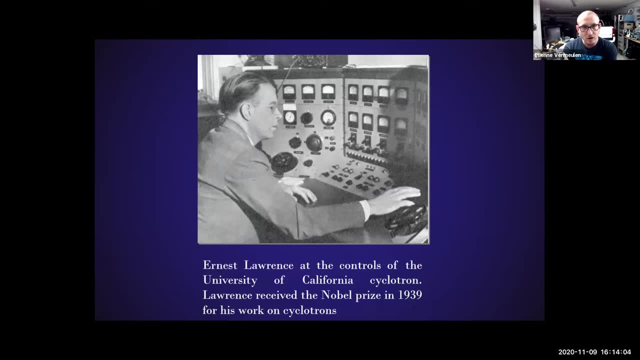 think the wonderful story about this is this control column was close to the cyclotron, um- and yes, he got the nobel prize for the cyclotron work- but also that control station was plugged into the same outlet as the cyclotron and and at night when they went home they turned it off and they 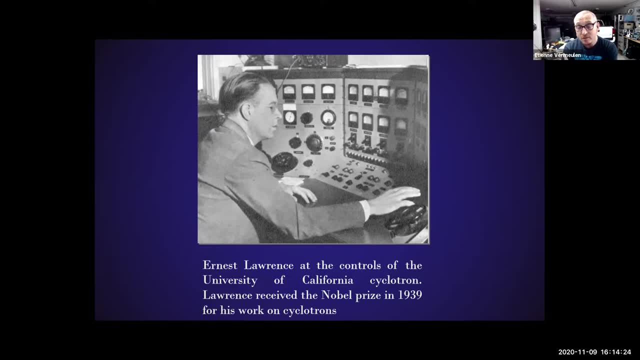 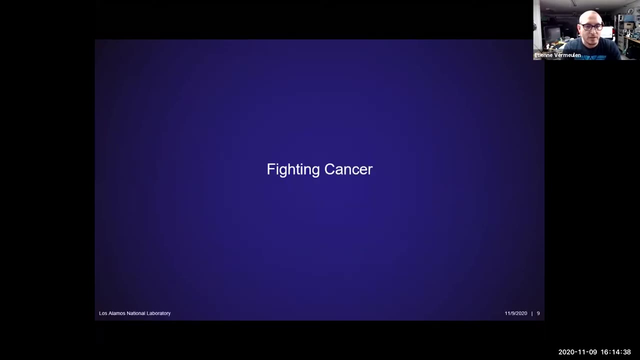 unplugged it, so they did not discover the isotopes that they made in that cyclotron. consequently, somebody else got the nobel prize for that, but you can argue that the first isotopes were also made at at berkeley, um. so why do we do this? and one of the major reasons we make isotopes is to fight. cancer. now, the isotopes are made to fight cancer and the isotopes are made to fight cancer and so to treat cancer. you have a bunch of opportunity or a bunch of ways to do it. the first way is surgery, of course, and you want to be removing the cancer with some sharp instrument. now, i'm by no. 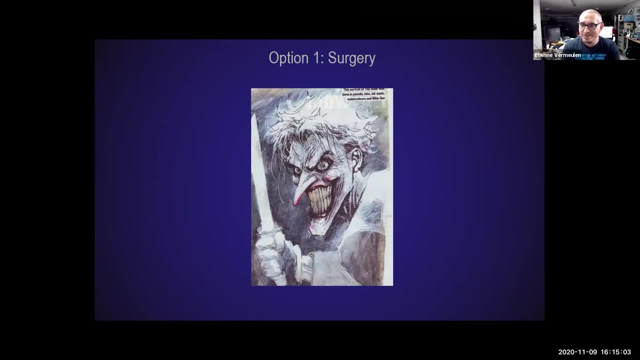 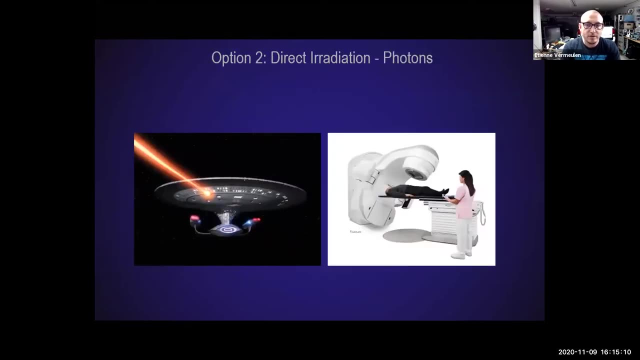 mean saying that all surgeons look like that, but the ones i've dealt with sometimes have made me feel like that. option two is direct irradiation with photons. so what you have is an electron accelerator which impinges the nobel prize for the cyclotron and the isotopes are made to fight. 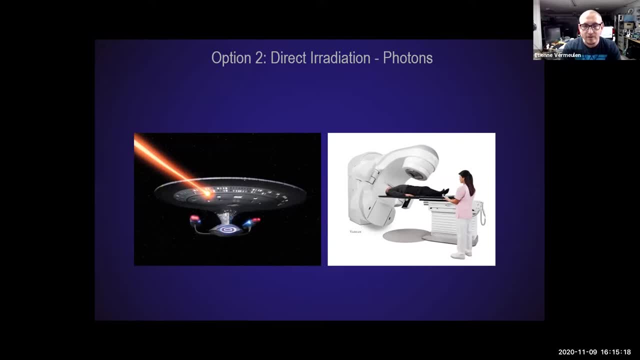 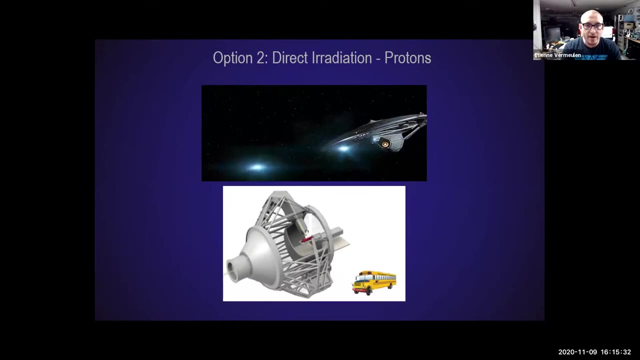 cancer. so the isotopes are made to fight cancer and the isotopes are made to fight cancer and the very strong x-rays that come from there can be used to treat cancer. so if you're into star trek, that's sort of like the, the photon cannons, um on the enterprise. another way to do it is directly. 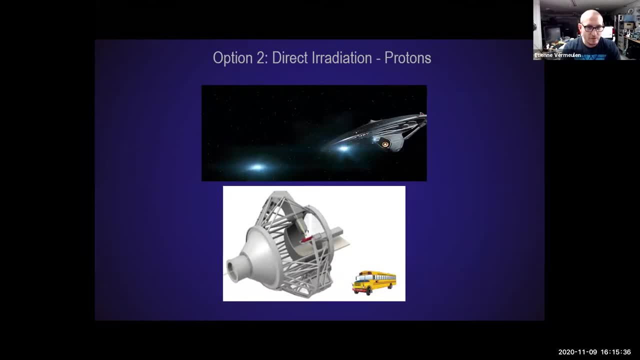 with particles, so protons, and if you have those photon torpedoes, that's probably more like the protons from the enterprise and that gets shot directly into the patient. the reason we can do that is because when protons stop, they drop all of their energy in a very short period, short space, and that's called the brag. 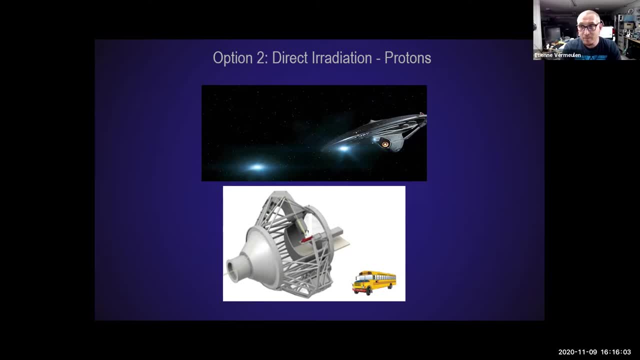 peak, if you haven't learned that yet, and i do fair warning, i do not have any formalism in this talk. this is supposed to be not a lecture. i'll leave that to lee to do that to you. but, um, what you see at the bottom here is actually one of the proton gantries, and i think this one is. 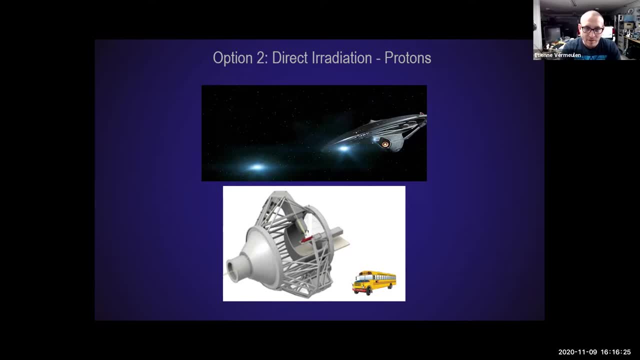 at psi and it's huge because you need these massive magnets to turn the protons around, so you cannot build this everywhere. um, it's very specialized centers where you get proton therapy and, while it's really good, it also makes damage around the area because it's still got to go. 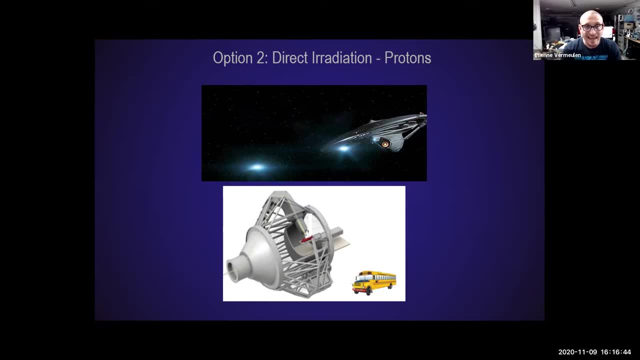 through the body to get to where the cancer is, and so you can't build this everywhere. it's very specialized centers where you get proton therapy, and while you can target you know um sub five millimeter tumors, it really is of the order of four to five millimeters that you can effectively treat. so if you want to get smaller, you've got to. 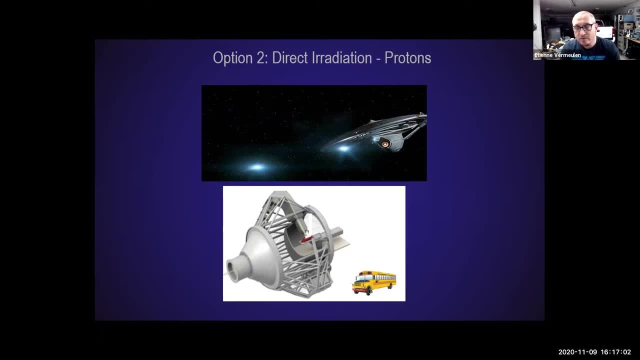 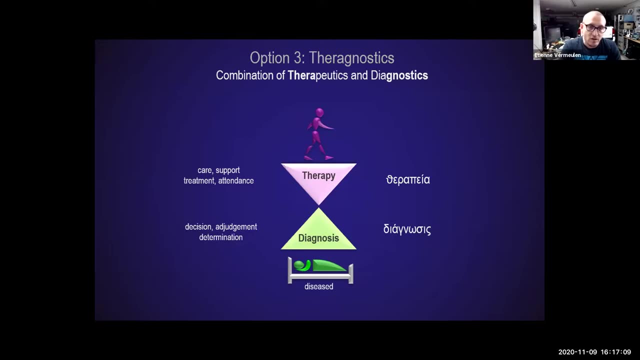 think a little bit more out of the box, and that's where one of the things we do comes in. so we do a thing, what we call theragnostics, and it's a combination of therapeutics and diagnostics, so the radioactive isotopes that we make can be injected into the brain and the brain can be. 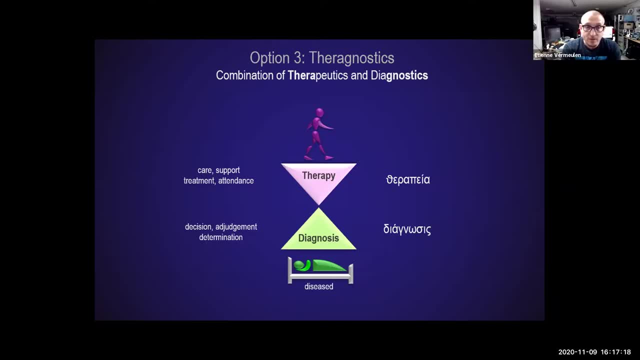 injected into a person, you can scan that person with a detector and you can detect the rate, the radiation coming from these isotopes. if you choose them in the correct way, they can either just be there for imaging or if they have particle emissions that stop in a very short distance. 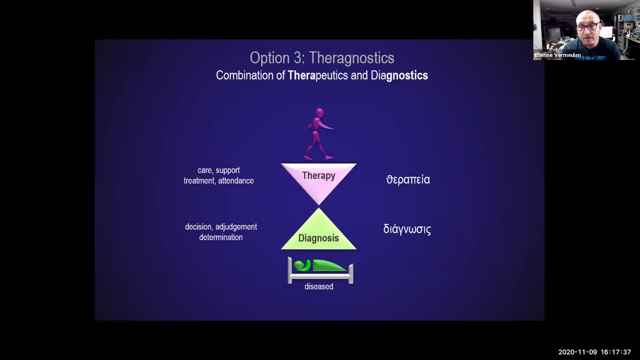 you can actually do therapy as well, and we'll talk about therapy isotopes throughout the the lecture. um, again, like i said, we're sort of following my journey and we'll touch on what every little bit of that does as we go along. a very interesting thing. 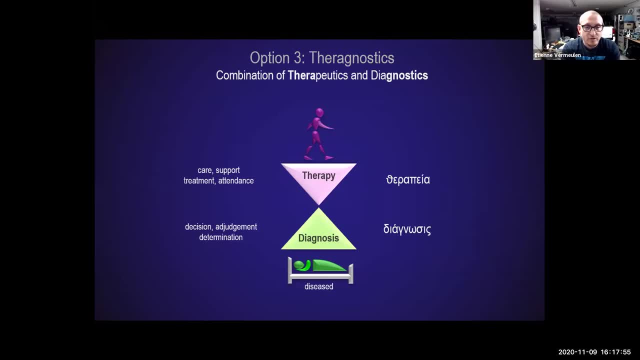 if you look at the, the greek words for therapy and diagnosis, it turns out that you have to say theragnostics. so you will. you will hear people say theragnostics, you will hear people say diabetics and every other combination of that. but if you study ancient languages, 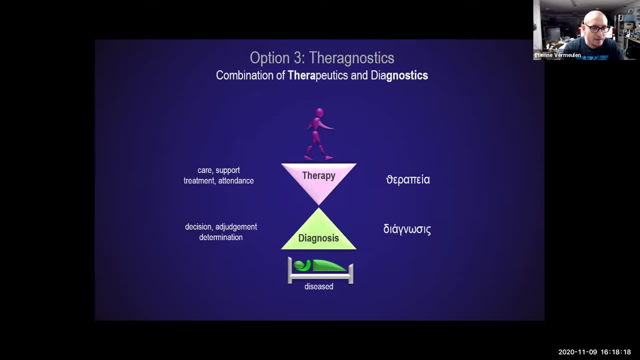 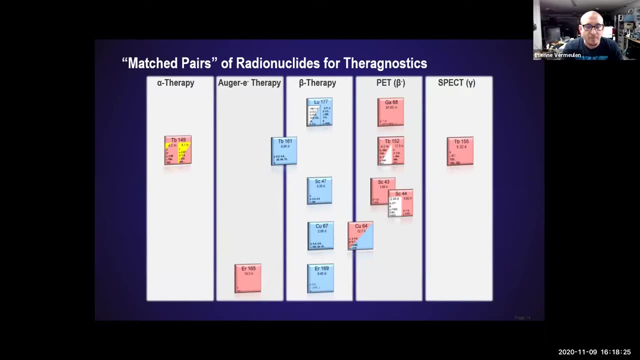 you will learn there are various different avenues for the development of theragnostics, um, but you also will learn that the development of theragnostics really involves many different ways, which is also the way that we teach at uni of work, so i'm going to jump right into that. 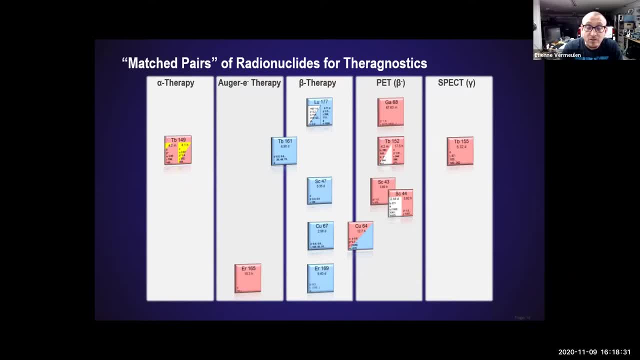 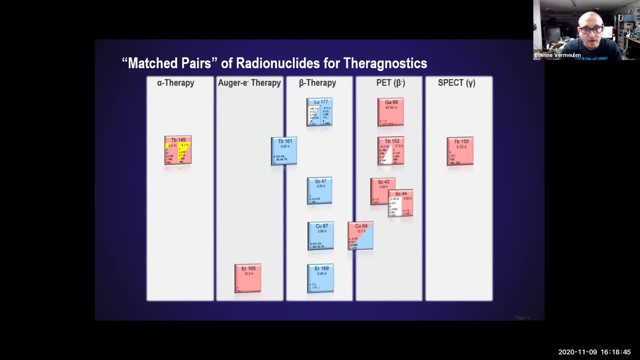 isotopes. that um give us this idea of theragnostics, um. so if you're familiar with the calls for a, ones are typically positron emitters or electron capture, and then those yellow ones are alpha emitters. and remember i said, if your particles stop in a short enough space, you can do a lot of. 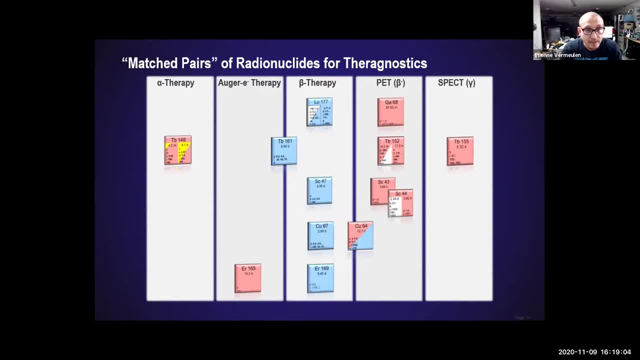 local damage, and that's something that you want when you're trying to treat cancer, especially very, very small tumors. so these blue guys are typically made in nuclear reactors. they have electrons that they emit and lutetium 177 at the top. there is by far the biggest electron therapy isotope, and 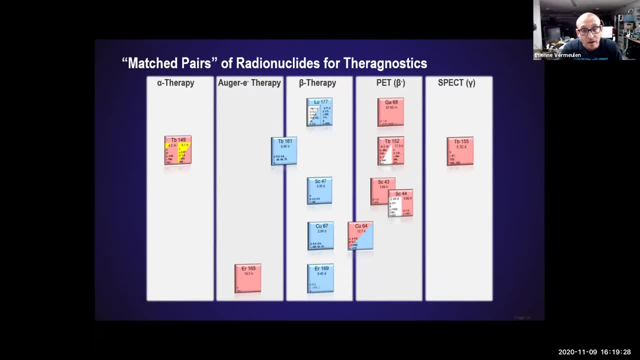 we'll come across that a little bit later in the talk as well. on the right hand side, those pink ones are your positron emitters, the the big one that isn't there is fluorine 18, which is probably by far the most used right now in pet scans. 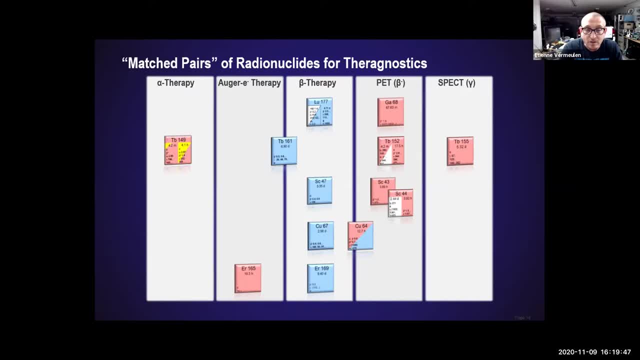 what's nice about pet is because it's emitting positrons. you can use the nullation when a positron meets an electron and it gives out two gamma rays 180 degrees apart. if you can detect those two and you can take the difference in the time they take to get to the detector, you can actually pinpoint. 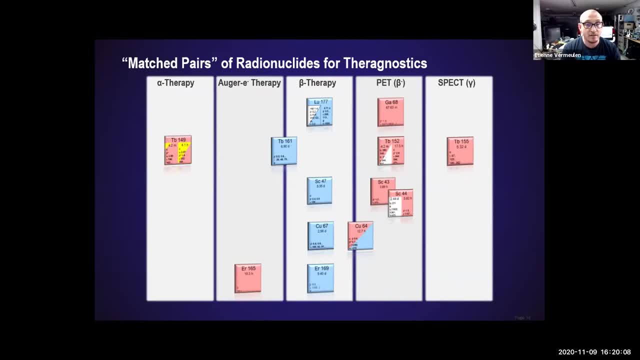 where the cancer is. you can make a three-dimensional image. this is pretty important. if you combine that with computer tomography, then you can say exactly in the box, exactly in the body, where it is now if you're doing external therapy. this is pretty important because you want to know exactly what you're hitting with with your external beam. 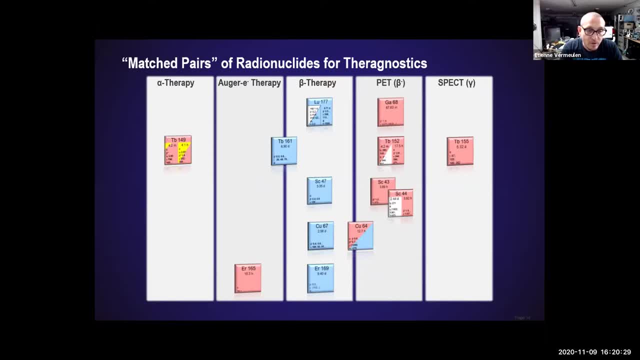 and then on the left hand side, there's terbium 149, and that's a pretty interesting isotope because it emits alpha particles. now, remember i said these, these particles have to stop in a very short space and we talk about. let me give you a few examples here. it's a near energy transfer, and if you have an electron being emitted, 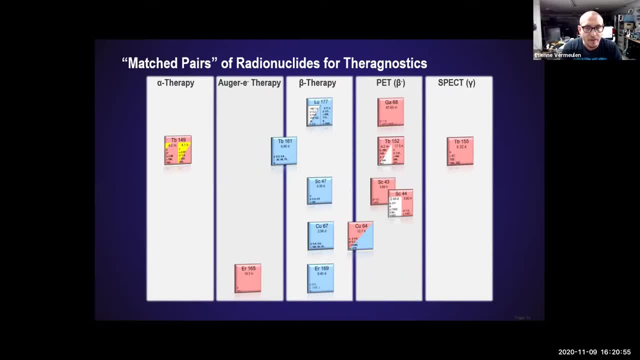 at quite a high energy. it's going to travel a couple of millimeters in the body. if you have a positron, it's going to be a bit closer and if you have an alpha particle- you can imagine- it's much easier to stop because it's such a large particle and because it stops. 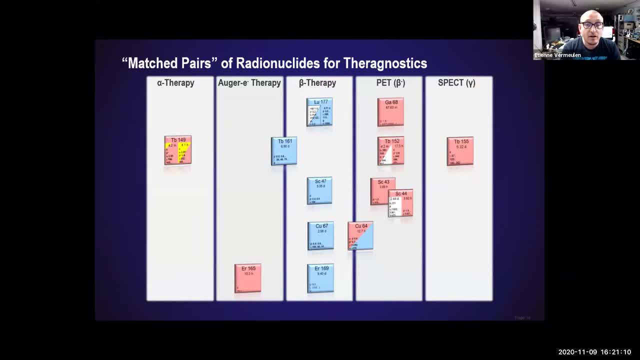 so quickly it does all the damage right there, where it is. so if you can target it properly, it will damage where you want it to. So I think that's enough of that for now. Just remember match pairs of radionuclides so we can image. 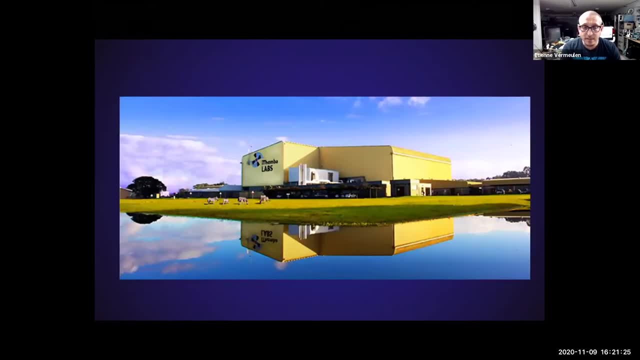 them and we can do therapy with them. So let's see where I started. I started in this wonderful place And there's animals. you see out, there are zebras And they're annoying because you have to chase them away from your car in the 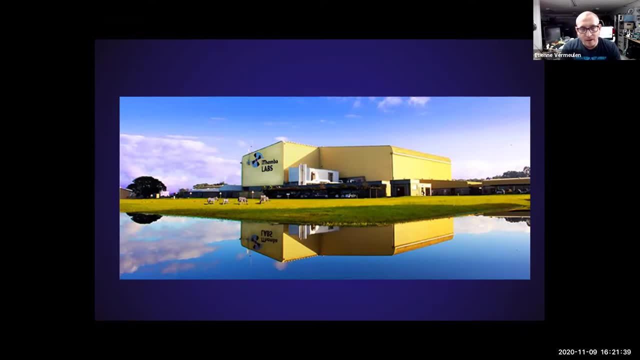 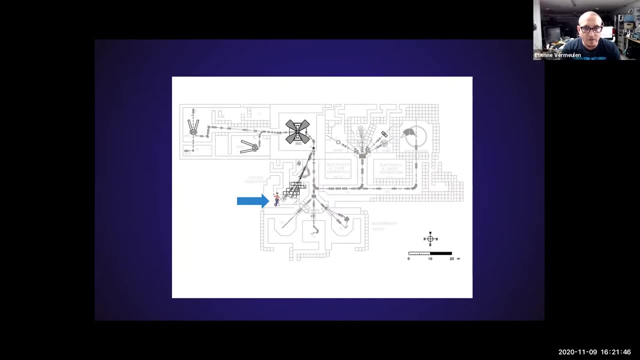 afternoon when you leave. But it, Tema labs, is accelerator facility built around a separated sector, cyclotron. So still staying with Lawrence's concept but taking it to a way bigger level. That little cross in the center and I don't know how to do the pointer. Let's see if I can do that. 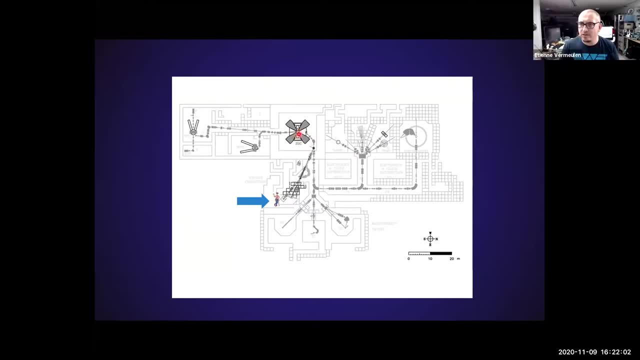 If it's PowerPoint, you can use Command L. Yeah, there you go, Can you? can you see my pointer? Excellent, Yes, So so this is the separated sector cyclotron. It's fed by two injectors cyclotron, One specifically for protons And then there's one for heavy. 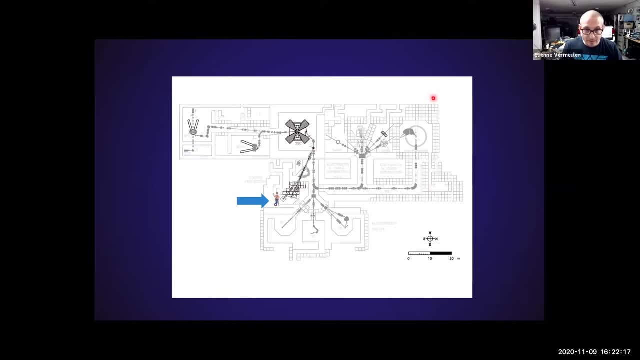 ions as well, Because on this side of this reactor facility they do all kinds of interesting physics. There's a magnetic spectrometer- This is Aphrodite, I don't know if you've told the guys about this. So this is a gamma array. There's a neutron. 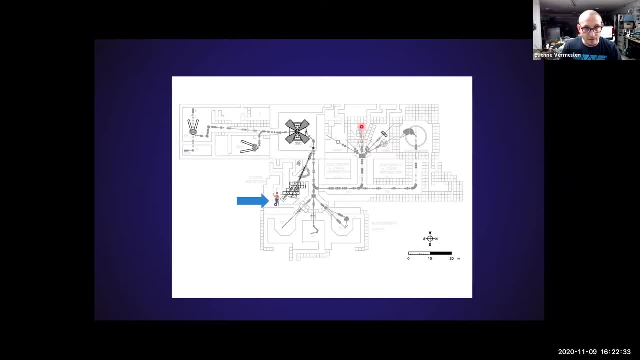 volt over here. So there's a lithium target and you can do neutron experiments, And then there's a scattering chamber over there where you can do proton, PP, Prime proton scattering experiments. But we didn't care much about that. This is where we were, So this is the isotope. 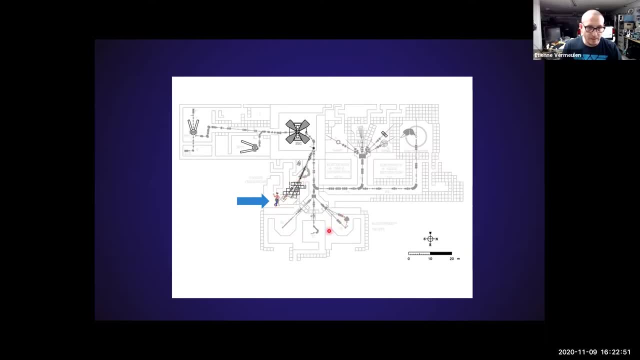 production section. Over here is a couple of proton therapy volts, So we did proton therapy as well, But this is sort of so. so that's me, Waldo, And you'll. you'll meet us. You'll meet me again in different places. Here we had three lines coming. 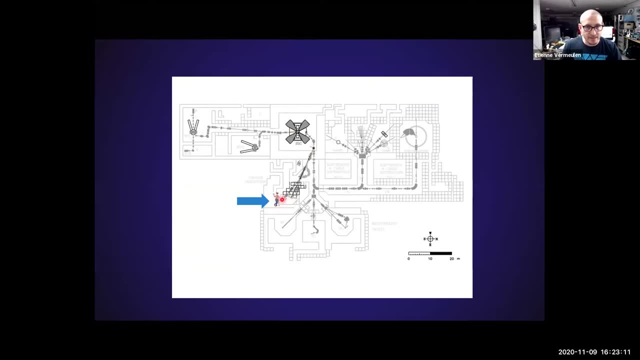 straight off of the cyclotron With protons at 66 MeV. The reason we use 66 MeV? because it was really good for neutron therapy as well. So we sort of we could do isotope production in between patients. But there's 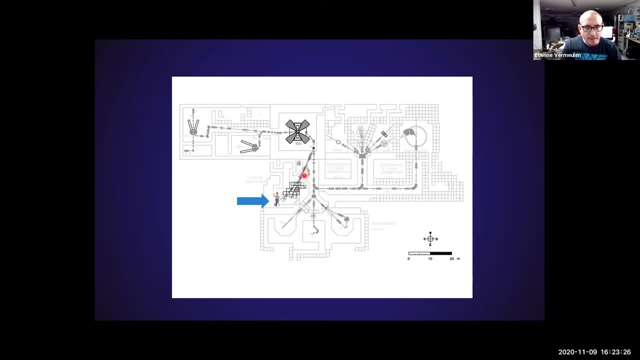 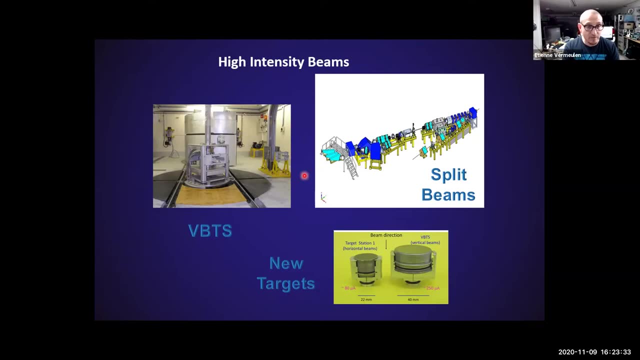 another piece here. that's really interesting. So what we did is we actually bent the beam down. So at some point we split the beam- because you can split a proton beam- And then part of the beam went down into the basement and part of it went straight into. 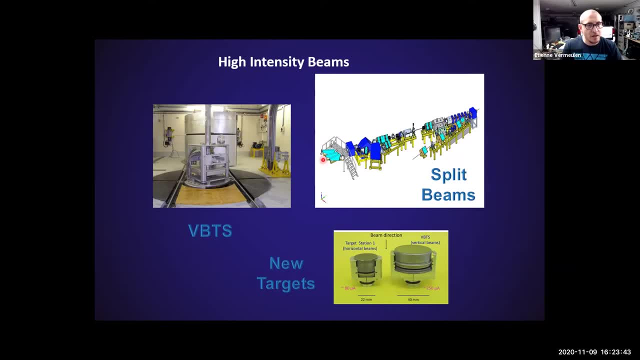 into those three lines that I showed you. On the left here, this is the vertical station, So a beam pipe coming down And that's a target holder over there And the targets would sit down here And then we had a train that would take the target. 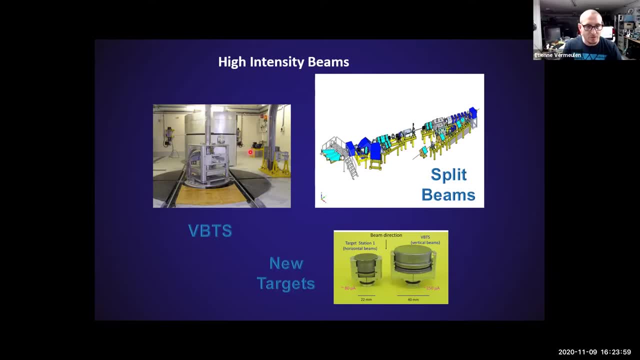 to the, to the hot cell complex to do chemistry. Targets typically look like hockey pucks or smaller, And they're filled with the materials that we want to transmute. So what are isotope production people? Well, we're alchemists. 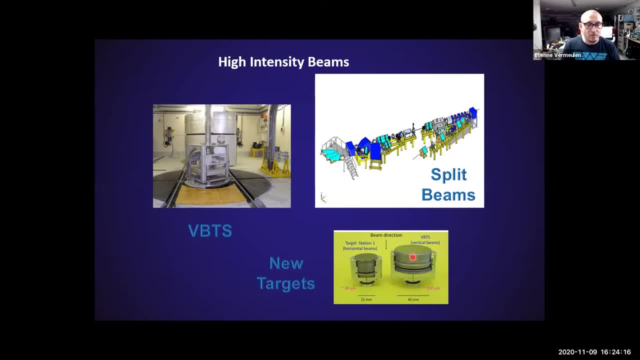 we really are alchemists. we transmute one metal or one material into another by shooting it with particles. That's absolutely what we do. So if you become an isotope production person, you can legitimately call yourself an alchemist, Because of the energies of what we have here. 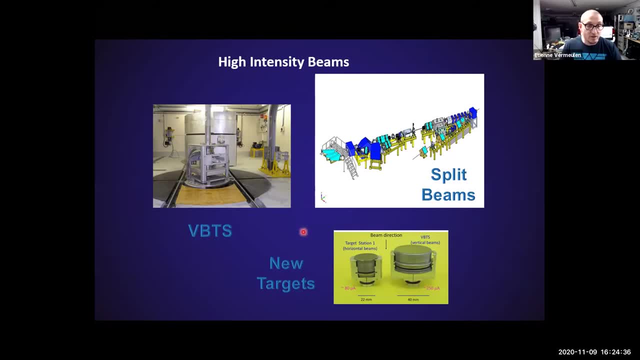 we also have to shield these things very well, because there's such a lot of radiation coming off that it will destroy everything around it. So what you see at the back, there is about 15 tons of shielding, And that shield moves and moves. 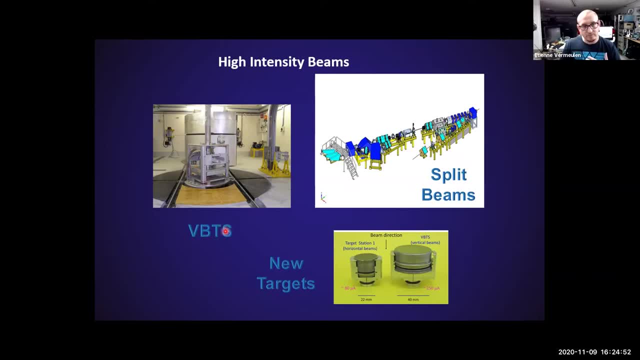 around this bombardment station. There's one on our side, looking from this side as well- And the way you do this is you have a core of very pure iron, specifically low in manganese, because you don't want it to get too radioactive, because you 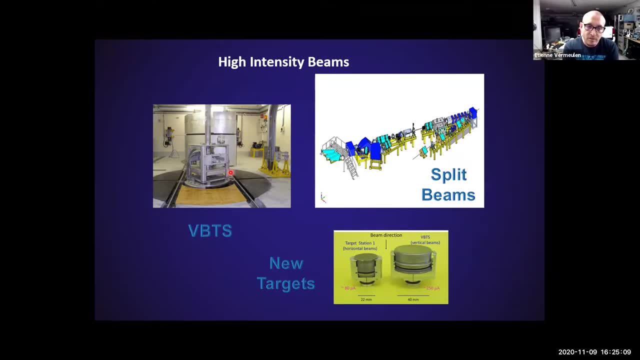 have to work in there. So what you do is you send all these protons coming out of these reactions. so you shoot the proton in, you kick a bunch of neutrons out. it's going to slow those neutrons down just enough so that when it hits the next layer, which typically in a 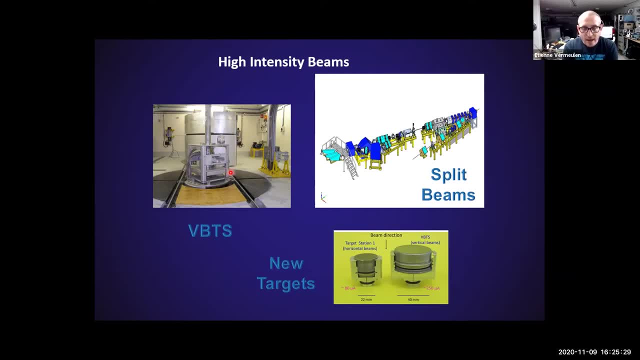 poor man's shield is candle wax and boron carbide. So boron has got a really high cross section for neutrons capture cross section. but it has to be slow neutrons. if they're too fast the boron is just simply not going to care, it's just going to go straight past. 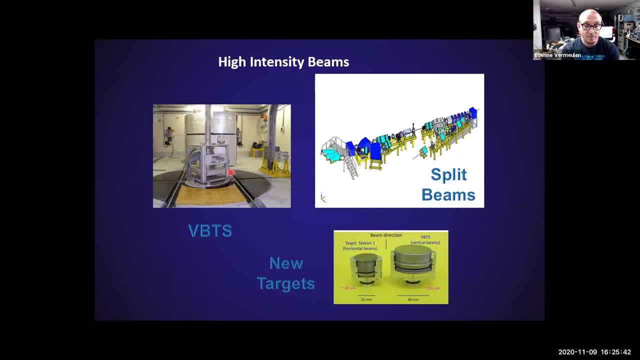 past it. So you use the hydrogen atoms in the cattle wax to bump the neutrons around and slow them down enough so the boron can start capturing them. The problem is that when boron captures a neutron, you get a- what is it? Lea, 1.5 MeV gamma, I forget, But you get a hard gamma that comes out. 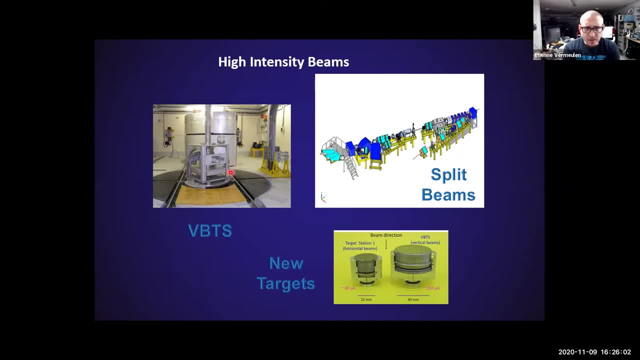 of that, So there's another layer of lead around that as well. That's twofold So it stops the prompt gammas that come from that boron capture. But it also helps you when you have to work around there so that you don't get too irradiated from this very hot center section over here. 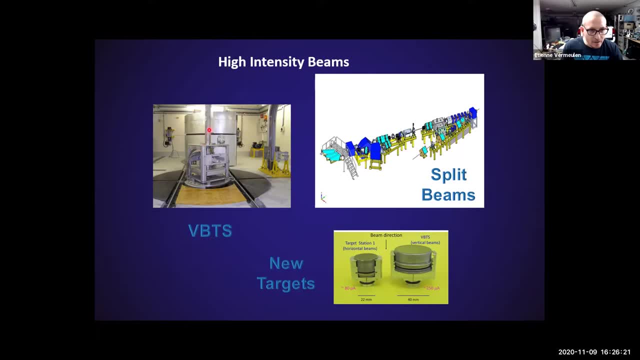 This is a really interesting arrangement. So these black things down here are actually tanks, And in those tanks are solutions of ammonium pentaborate, because it was just easier when you worked on the boron capture, So you don't have to work around there. So you don't have to. 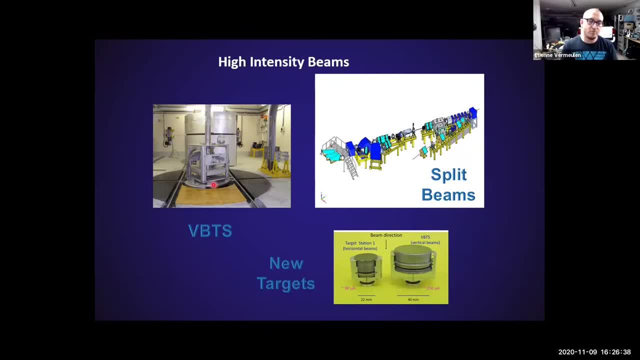 work in the floor to have a liquid in there, So another way to get boron around your target. So, as you can already see, we're talking about chemistry, We're talking about engineering, We're talking about physics, And they all mix together to make sure that we can do. 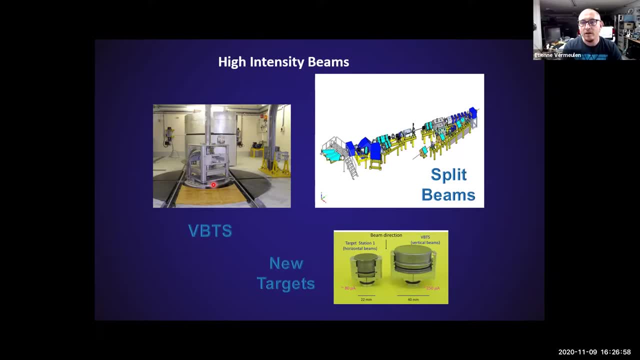 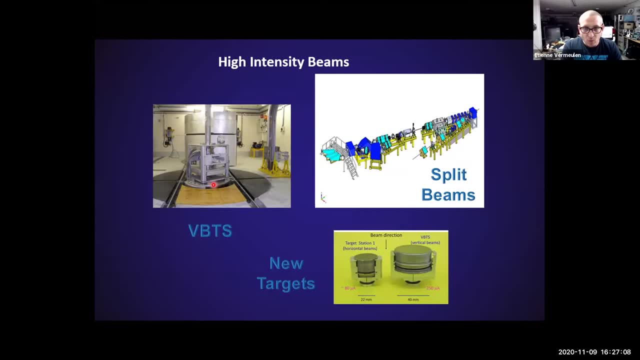 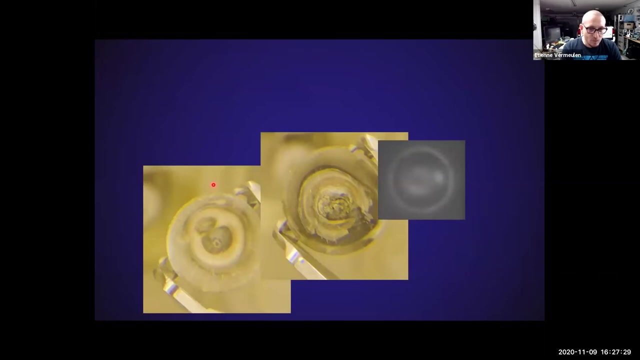 So this is work at the bleeding edge of technology, And things don't always go right. Actually, more often than not, they go quite wrong, And if you look at this target at the bottom right here, when it goes wrong, it goes wrong spectacularly, And this is an interesting thing. 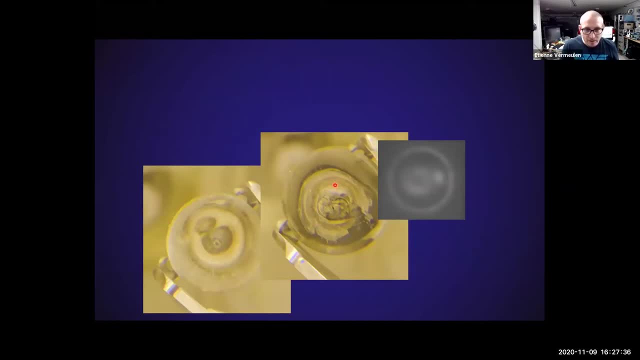 So this is the beam spot on this target. This target is about an inch and a half in diameter And what's happened is the beam has actually collapsed. So typically, when we have these large targets, we will raster the beam in a circle just to spread the heat out, But this guy collapsed And you have to figure these things. 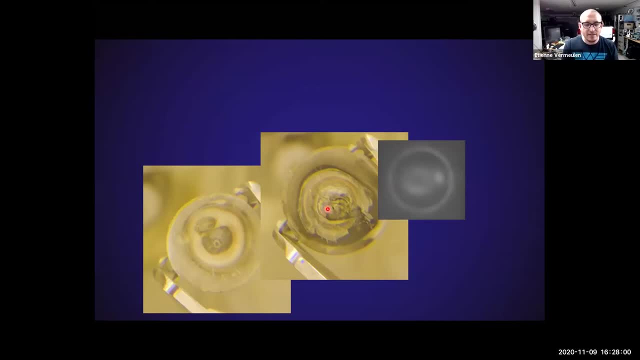 out like plane crash investigations, Because once it's happened it looks terrible like that. So you have to kind of dig into the hole. So what do you have here? course, it went south pretty quickly. now. radiochromic film is really interesting. it's not just a little. 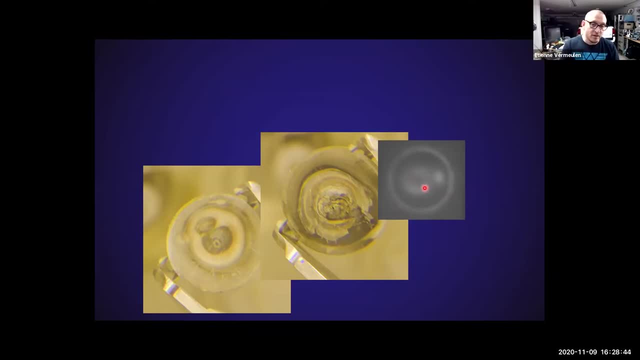 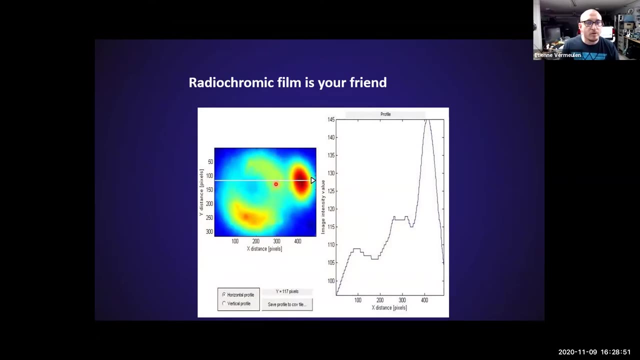 x-ray like that. in here is a lot of information. so if you go and scan that and you analyze it, what you see is this, and this tells you a lot more about what happened. you can see, this is the most radioactive spot, so this is where the beam went when it became one spot. and if you analyze 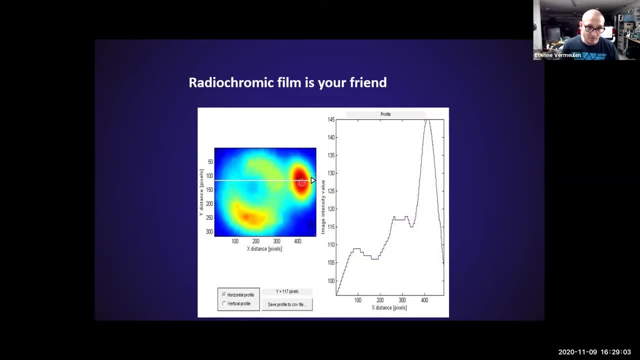 across it, you can see it's really radioactive, so so we could say that the beam actually stopped there and drilled into the target. so how can we learn how to make these targets better? because it's all about keeping that material inside of the encapsulation and one of the things we can do. 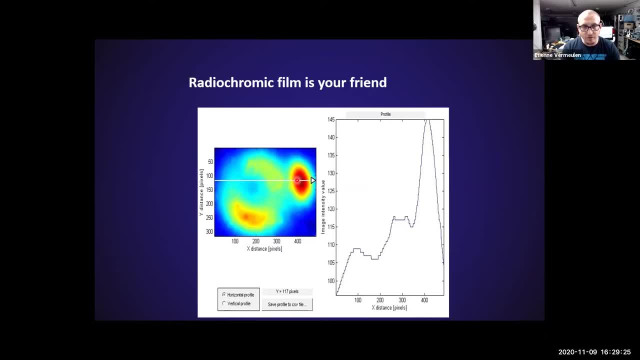 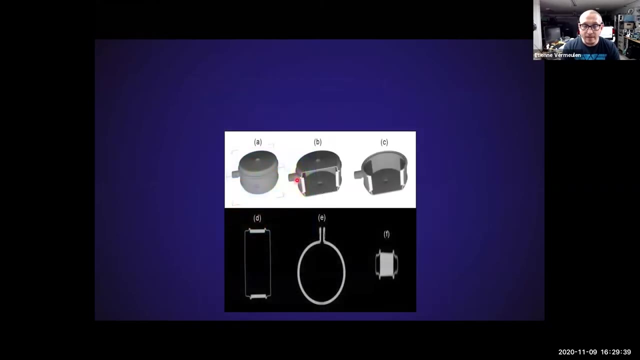 that's pretty interesting is radiography. now, if you use simple x-rays, these stainless steel targets are too thick to penetrate and all you see is just a dark spot. so one of the things we can do is we can leverage neutrons. you can create a neutron radiograph. so in this case, we were actually 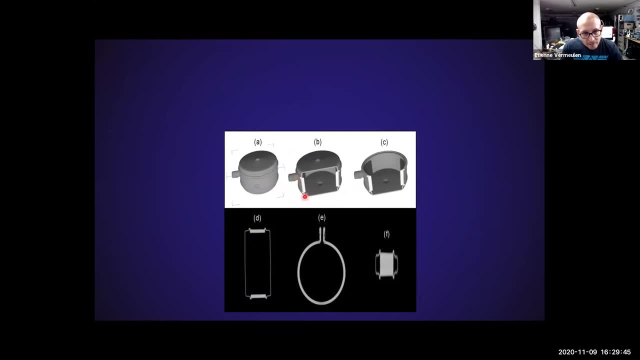 looking at the welds, and if you look there and there, those welds were of a concern and so, using neutron radiography, we could actually do cut throughs of this material. if you look carefully, you can even see the threads of the swage lock fitting over there. so it's, it's actually. 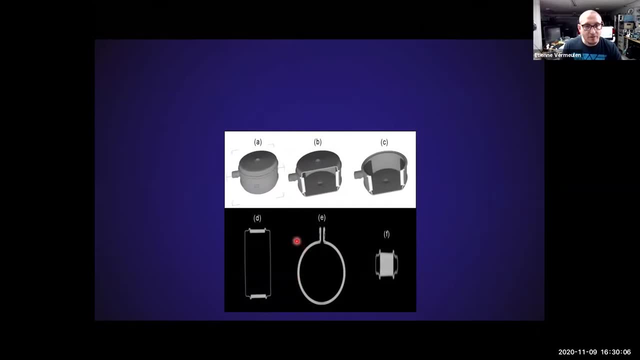 pretty fine measurements that you can do and through doing this, you could say, okay, well, these welds are strong enough and they probably won't, and yet they do break when we put proton beams on them. so one of the most important things I learned working at this accelerator: 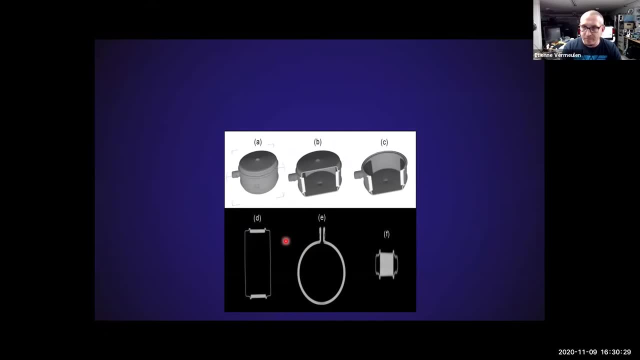 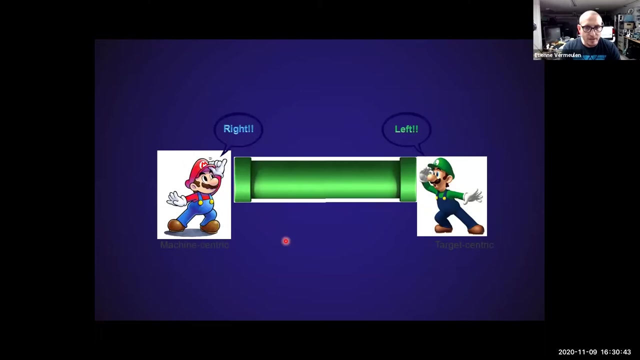 facility is when you're at the end of a beam line and somebody's shooting protons at you, you need to know where the beam's going, because the guy looking from the other side has a right and a and it's always balanced between target centric and machine centric. so if you've got beam coming, 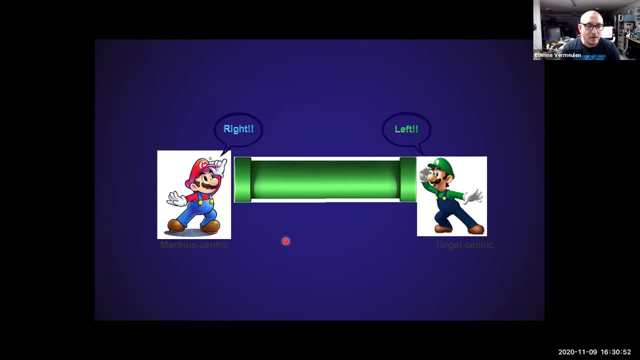 at you. you always have to think from the operator's point of view that if you say the beam's got to go left, he's got to go right, and if you say that one's got to go left, then the other one doesn't to steer it to your right. uh, so hopefully luigi and mario will stay in your mind next time you. 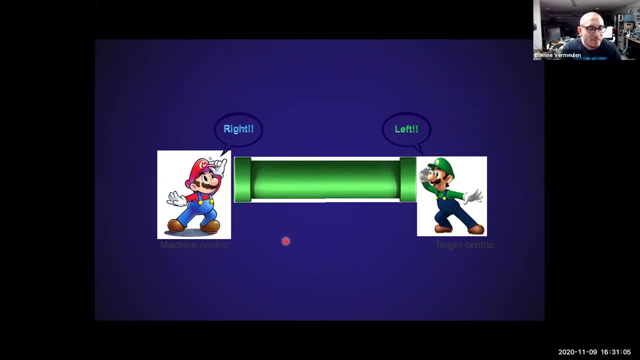 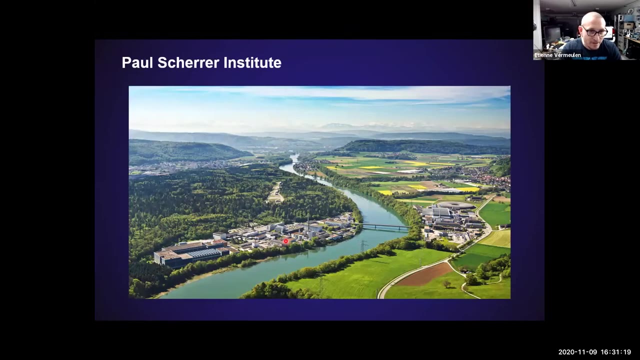 you ask for beam at the at the berkeley cyclotron. okay, so so from south africa. after a number of years, as lee said, um, i went to switzerland and i went to the largest research institute in switzerland, which is not cern but is the paul sherry institute, because cern is its own little. 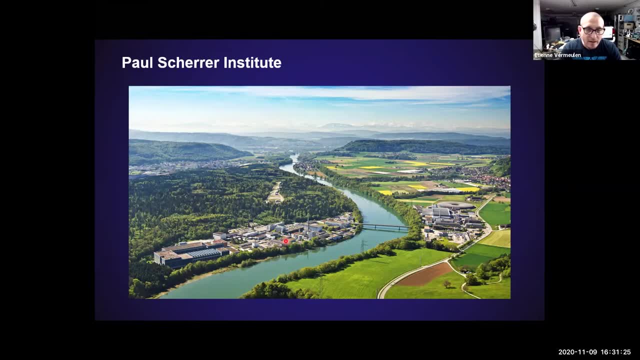 country. it straddles the border between, uh, france and and switzerland, and we'll get to that, but first we'll have a look at psi, and psi is a fascinating place. um, it's built on both sides of the ara river and this river runs through the length of switzerland. at the back there you can. 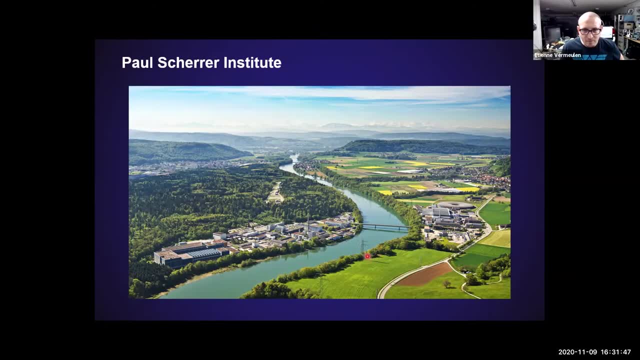 see the beautiful swiss alps, so it's a really picturesque place. on the right hand side there's the cyclotron complex and we'll have a look at that shortly. this is the swiss light source, so that's a electron accelerator. there used to be some reactor facilities on this side of the river and in the 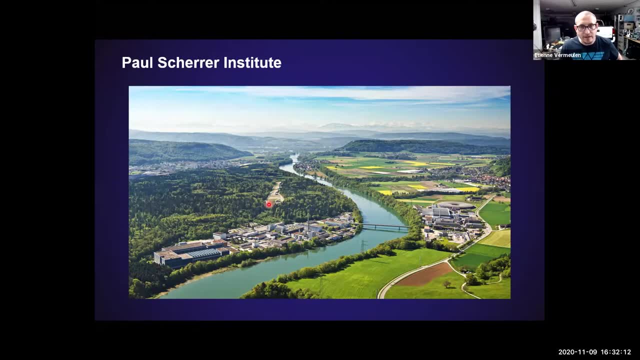 forest here. this is called swiss fell, which is the swiss free electron laser, which is one of the most powerful free electron lasers in the world and is going to do some amazing research when it's going and and running. and the other interesting thing about this facility is this building down here. 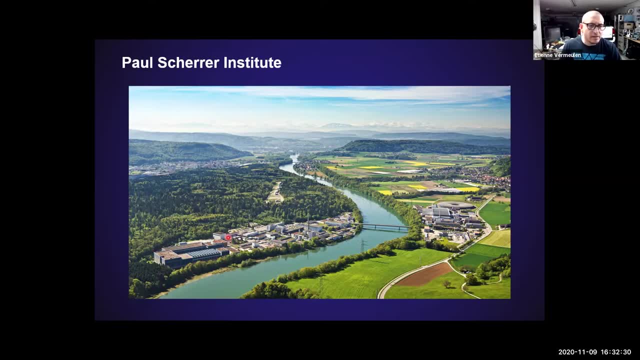 contains all of switzerland's nuclear waste. they cannot decide where to bury the waste, so in the meantime they're just storing it at psi, and if you're ever at this facility you can go there and ask them to have a look. there's a little window at the top of the building where you can look down. 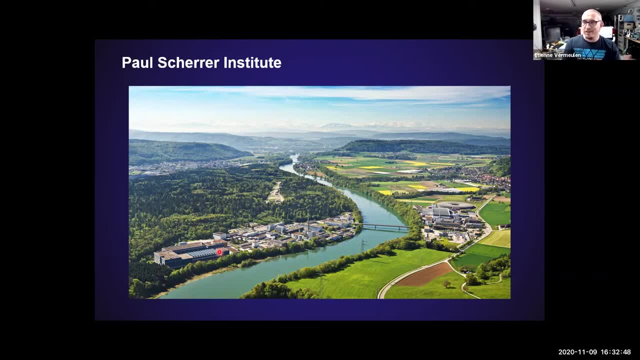 and see all of switzerland's nuclear waste, for anybody who's interested in that type of thing. but mostly that's the basic thing we've got and we've got a little room for that in the lower part of the slide screen. so how do we do that? so we'll go in just a second and i'll just tell you a little bit. 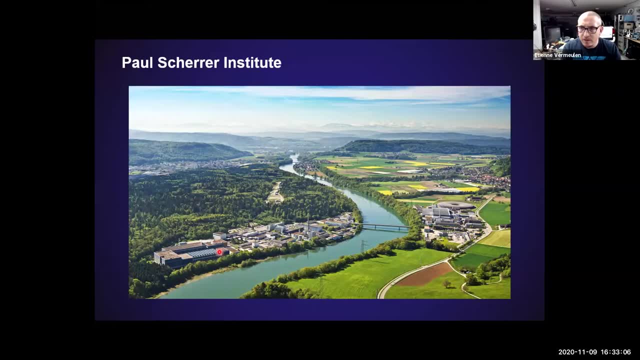 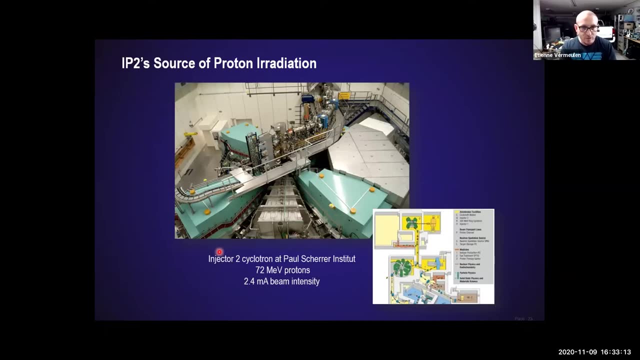 what we are doing here is we have a really good selection of prototypes, so a very good selection of prototypes in the next slide and, of course, we have this so-calledPCAN webinar, and they're- these are just some quick swatches of some of the ones that are really we've got. this is our 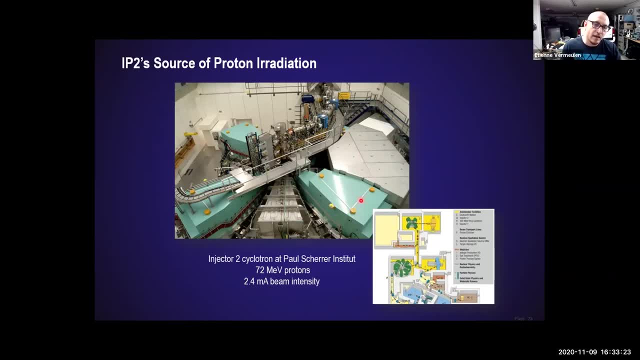 this is a wonderful cyclotron. the cyclotron and these magnets are about 500 tons a piece, so they're pretty huge. this cyclotron can be operated by one person, so all of these pieces drive out on rail, so one person can take the cyclotron apart and do some maintenance on it, if you look in the right. 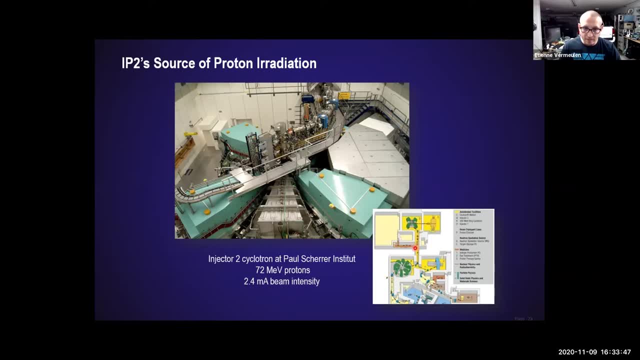 hand corner here. that's the cyclotron, and then the beam there goes to the ring cyclotron, which is the most powerful cyclotron in the world. now people at triumph will say: but they have the biggest one. psi says this is the most powerful one. it takes protons up to 800 mev and then from 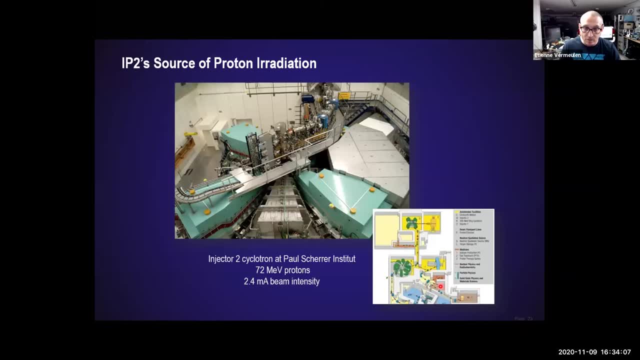 there it goes on to sync you, which is a spallation neutron source, and it's also one of the the most powerful spallation neutron sources in the world, as well as the there muon research facilities. so they do a lot of muon work. 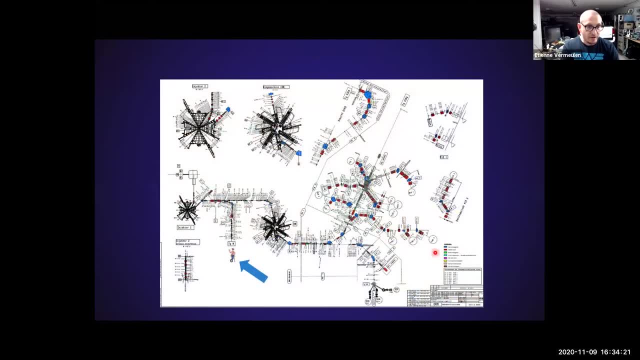 so, if you can find waldo using the handy arrow, this is where we did some isotope production and interestingly enough, again it's a beam that's split. so there's two milliamps of beam going to this cyclotron and we were taking about 40 microamps and slicing it off of the beam so that 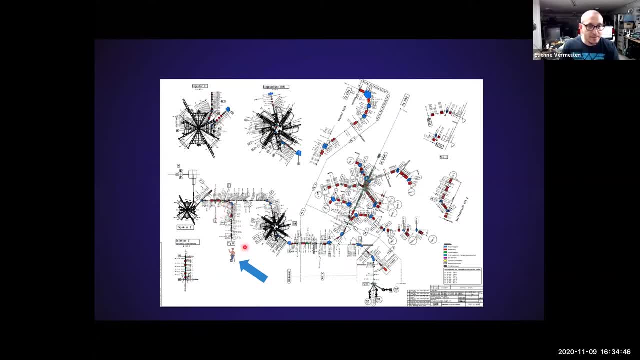 that's actually quite a bit more complicated, because we can't really see the beam coming off it. it looks like a film you just go across and it's directly in the shape of a nickel, so that's why it looks like it's. that's how we're doing it. and then this one, the other type, is, uh, the mega beam and the the. 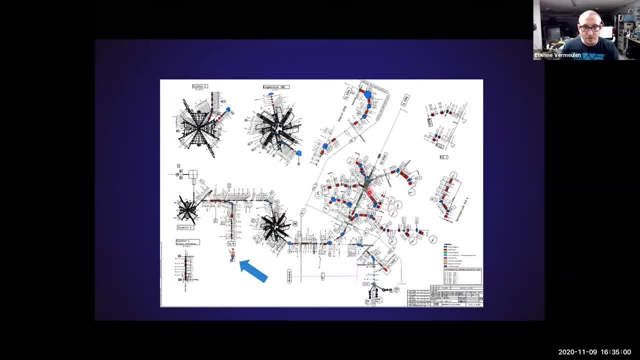 one that's a little bit easier than the other type is the muon, and this is a kind of a multi-uniform beam which is really big and it can take up to 150 tons and one of the most powerful of those in the world. it can take up to 20 tons and that's one of the biggest ones in the world. So how do we do this? If you want to do reactions at lower energies, the only way to do is to degrade it, And at PSI we degraded the 72 MeV neutron beam down to 30 MeV sometimes, sometimes even down to 16 for this specific one. 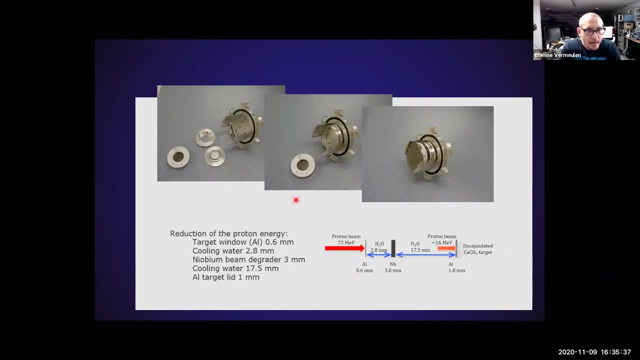 This was for the production of scandium-44.. And usually you have a degrading piece and that's a piece of niobium that will degrade the beam, and then you have a target behind there And these were typically smaller enriched material targets. 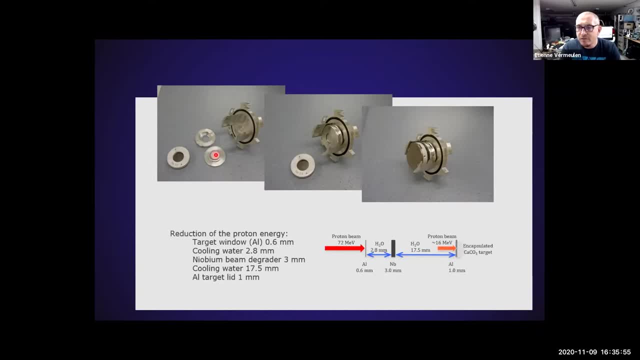 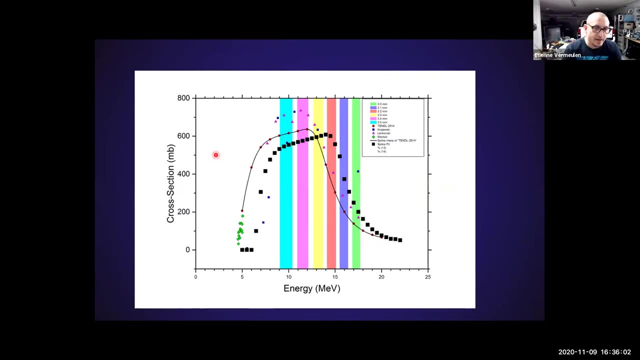 And I'll talk a little bit about that shortly. But first let's have a look and see how do we determine the energy that we're going to do these irradiations at? And this is pretty important to think about, because protons have a stopping power. 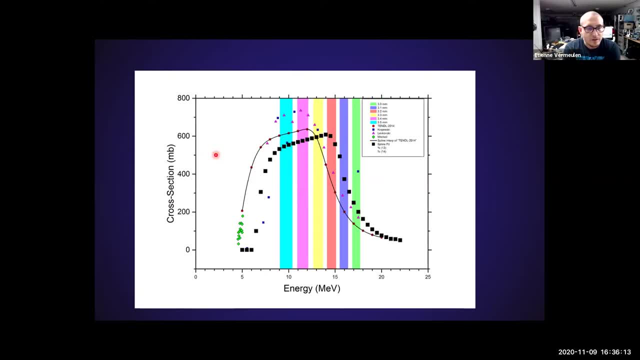 and that stopping power is a function of the energy of the proton. So the faster the protons go, the easier it is for them to move through material. As they slow down, it becomes more and more difficult, And this is because of the power. 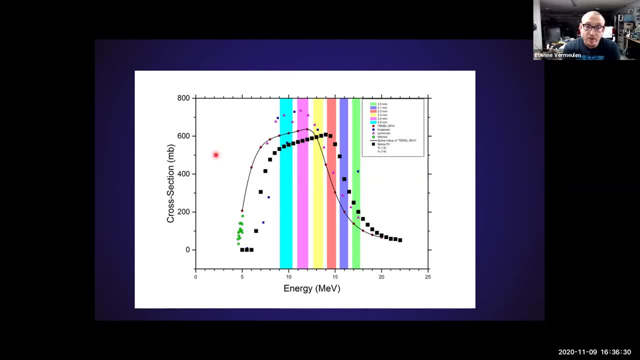 the electrons have over them. So you can imagine running into a crowd of people. At the beginning you can get past three or four layers of people because you're going really fast, But as you slow down, more of them can grab at you. 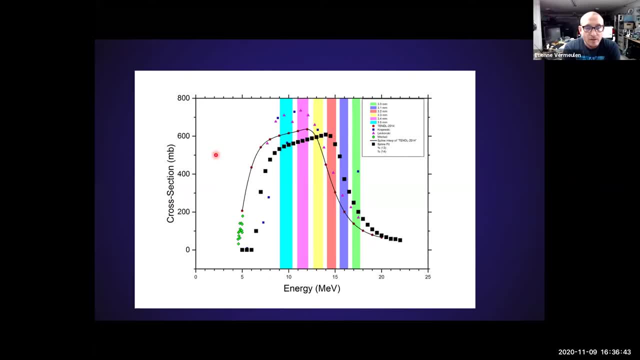 and you slow down much quicker. As a consequence, the energy window of these protons and the amount of energy they lose becomes bigger and bigger the more you go down in energy. So what you see here is a typical cross-section that we measure using foils. 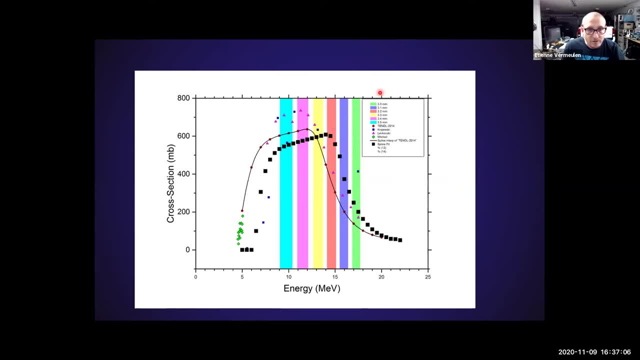 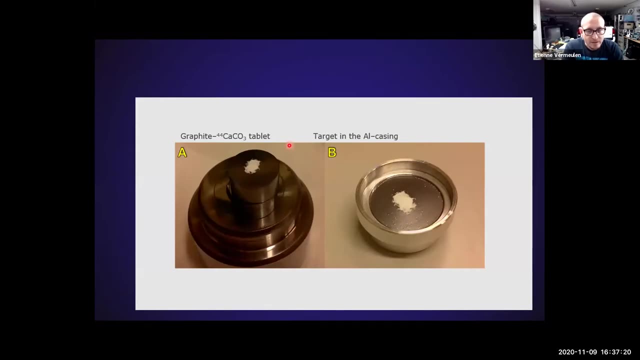 And these colors are the different thicknesses of degraders that we use, And you can see how the energy window gets bigger and bigger As we go down. So how did we make targets for these guys? This is pretty interesting. This is calcium-44,. 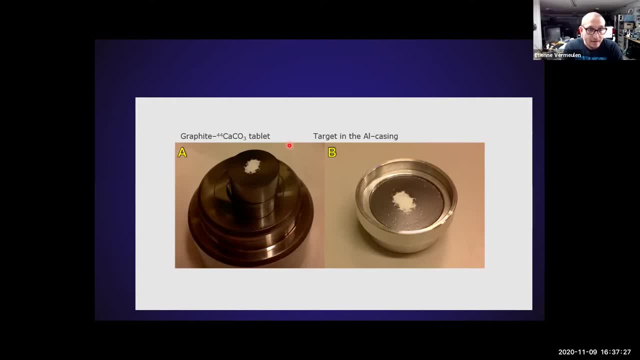 which is a very expensive material, And remember I told you that some of our targets look like hockey pucks. Now, a hockey puck of this material would probably cost about a million dollars. This is about $1,000 worth of material, And if you have to do this every day, 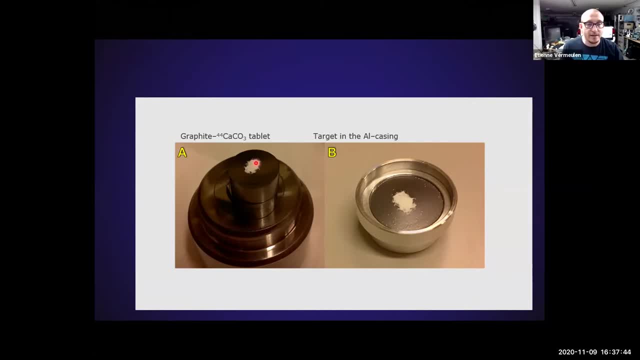 because it's pretty short-lived, the cost quickly mounts up. This, however, is not a really good way to make a target. So what this is is graphite powder And you add some of the calcium powder on top and you press it and it becomes a solid disk. 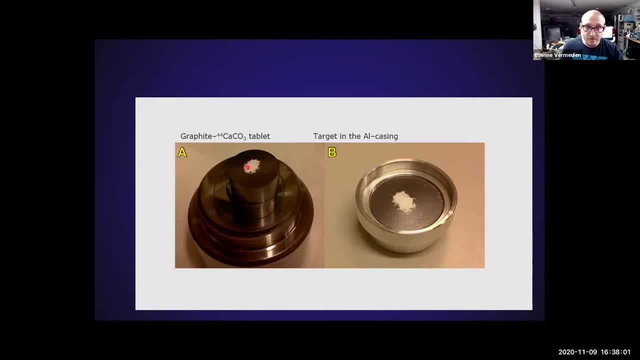 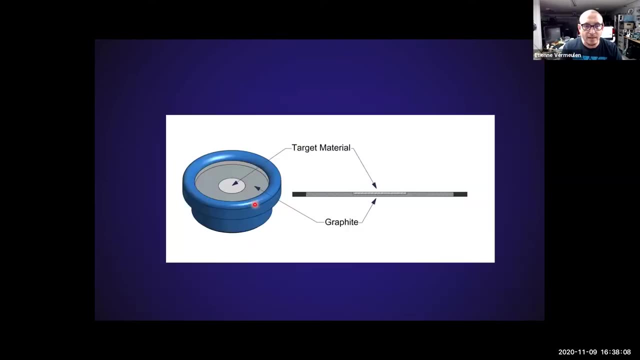 But you have no control over the thickness of this target or the shape of it. That's why it looks so strange. So we messed around with it a little bit and we came up with a different target design. that was a pressed target. So that's about it. 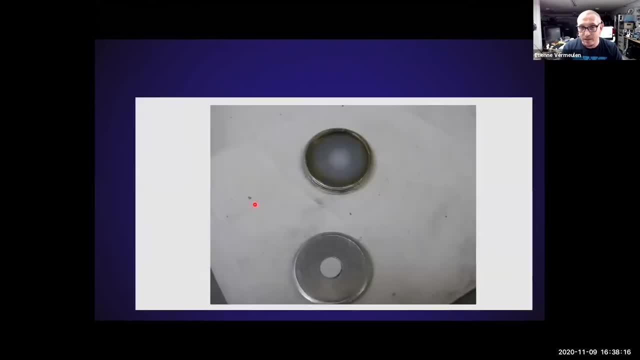 It's about a $1,000 target right there. This is what it looks like in real life, And with that little pellet we can make enough material to treat probably 10 patients per day. So that's it. That's a pretty good way to go. 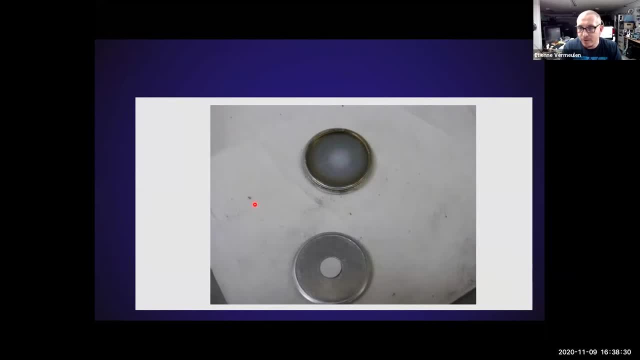 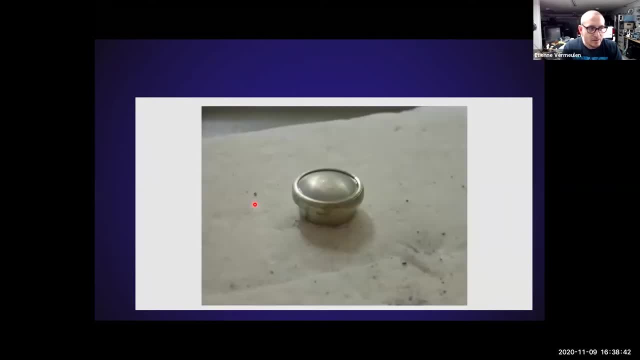 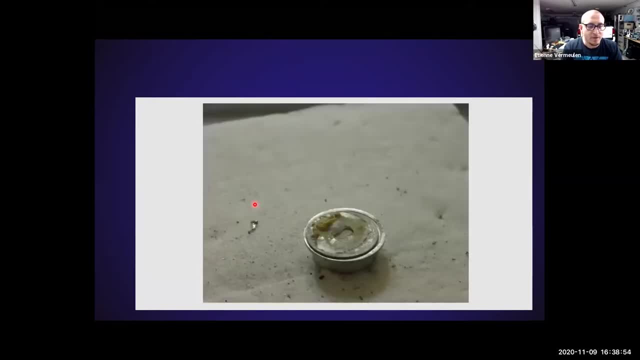 And then when you cut it open, oops, this happens, oops, this happens, And this is pretty interesting. So when you use salts and you irradiate them, of course the protons put a lot of heat into your targets. 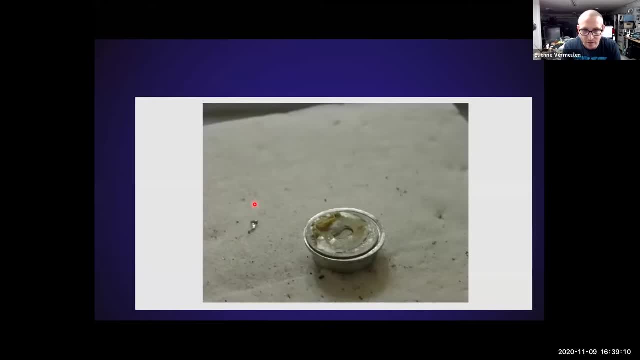 And if your salt is wet? And if your salt is wet, you're going to turn that water into steam. You're going to turn that water into steam And this is going to create a bulge, And this was not the case here. 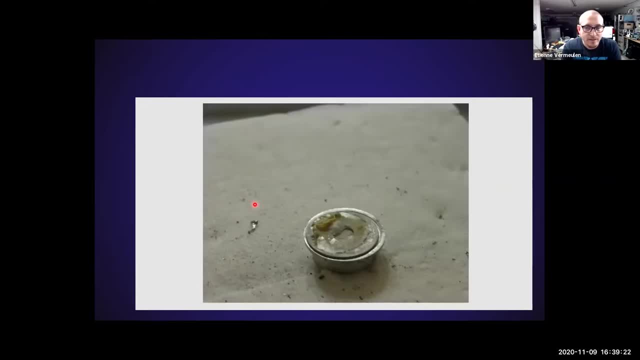 We actually did dry it very well. So why did this happen? Well, there's another problem, and it's something if you're ever going to make targets to remember is that a lot of materials absorb CO2 from the air, And that's what happened in this case. 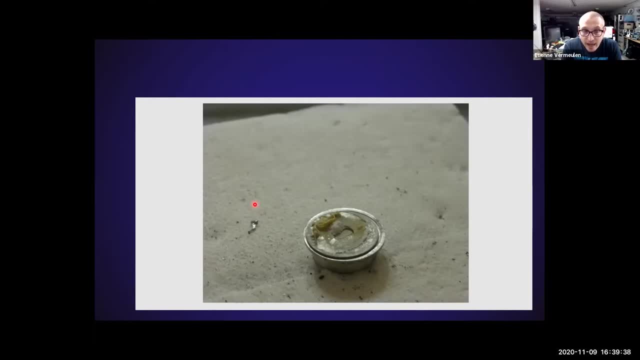 This stuff absorbs CO2 and if you get it hot enough, it will start releasing the CO2 as CO2 gas. and if you get it hot enough, it will start releasing the CO2 gas. So I think that's enough of broken targets right now. 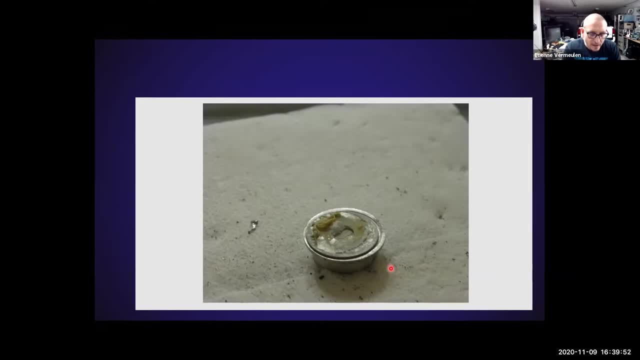 of broken targets right now. The other place I managed to make targets- if we take the adventure a little further- was CERN, And this was through a collaboration we had between PSI and CERN. we had between PSI and CERN, And CERN is not an obvious place. 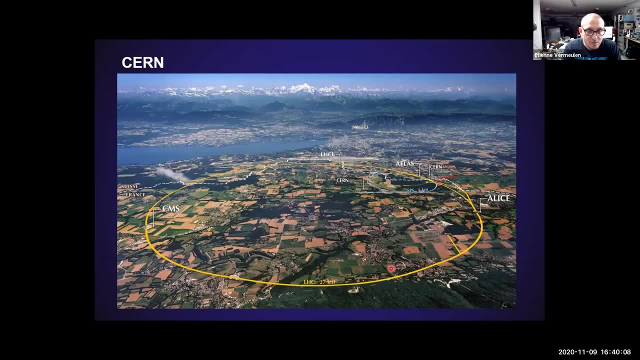 to make isotopes. It's pretty huge. So you can see that's the size of the accelerator. It's 27 kilometers in circumference. It's 27 kilometers in circumference. This is Geneva over here And that's Lake Geneva there. 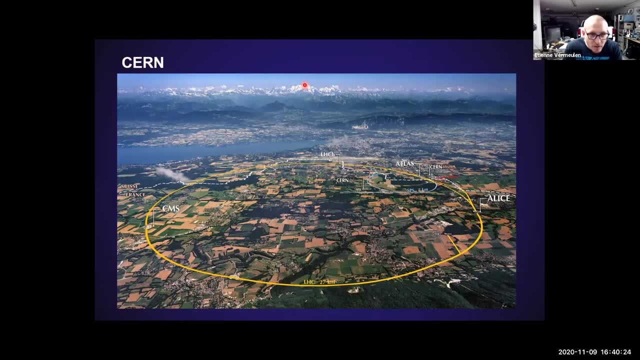 That's the French Alps And that's Mont Blanc over there. And every time you go to CERN, people will say to you: on a clear day you can see Mont Blanc. And it's never a clear day, so I've never seen Mont Blanc. 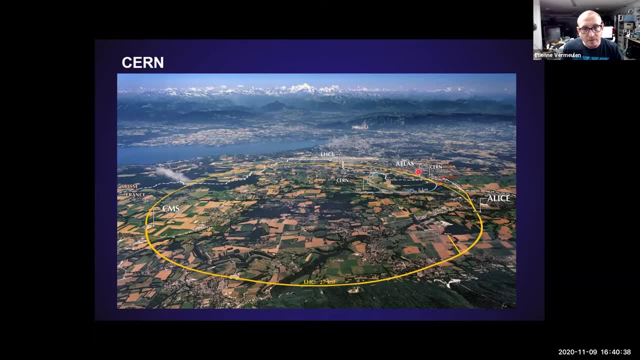 other than this picture, But if you look a little bit closer, there are smaller accelerators here that feed into the big LHC, And one of them is the proton synchrotron. is the proton synchrotron, And that's this accelerator over here. 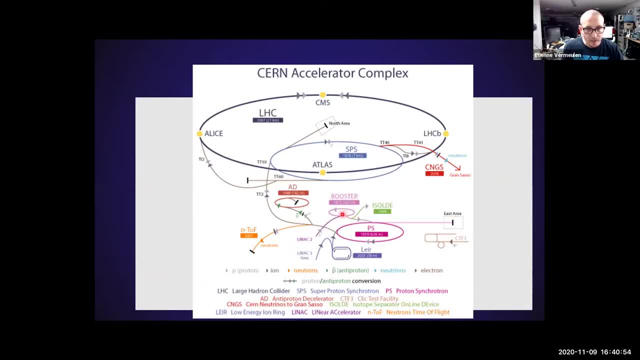 And this accelerator has a booster and it's got a LINAC that feeds that. And next to the LINAC is ISOLDE, which is used to make radioactive beams. ISOLDE stands for Isotope Online. I can't remember the other part of it. 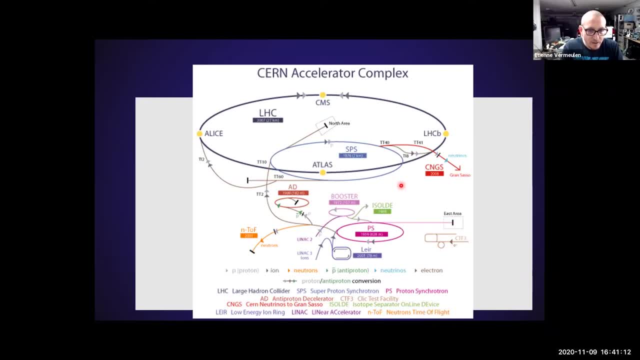 I can't remember the other part of it: Isotope, Online Separation And what happens there is? protons get accelerated up to 1.2 GeV And if you hit a high Z material with a proton that fast, it pretty much makes everything. 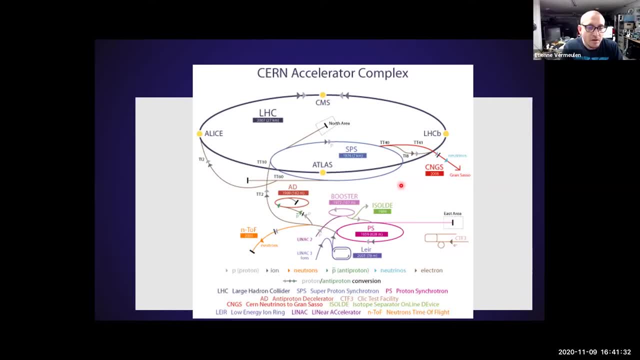 in the nuclei chart. So if you're pretty smart and you can pull those isotopes out of that target and into a mass separator and then post-accelerate that, you can actually isolate some of these isotopes and have beams of those. 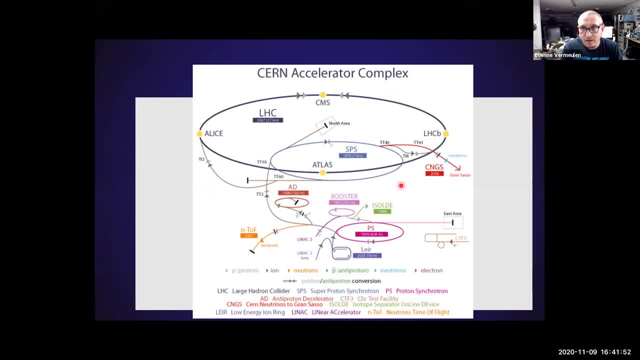 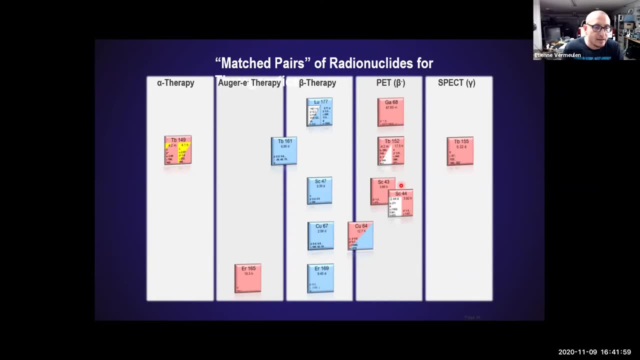 and then do all kinds of experiments with them. Of course, what we did- and we're back with the match pairs picture again- is we were looking for terbium-149.. So we were pulling mass-149 out of that target and embedding it into zinc. 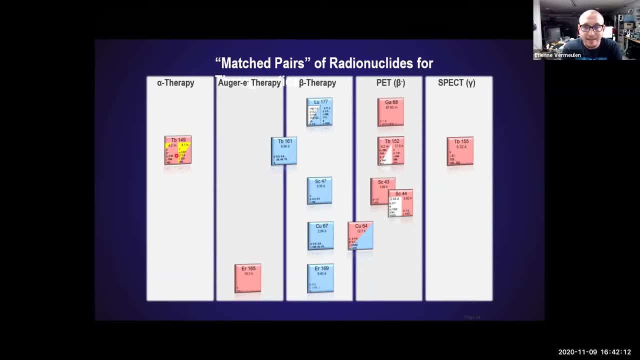 because zinc's a nice soft metal. It'll catch something and the chemistry of it is easy. If you know anything about lanthanides, lanthanides are incredibly difficult to separate because of the thing called the lanthanide contraction. The lanthanides are chemically very similar. 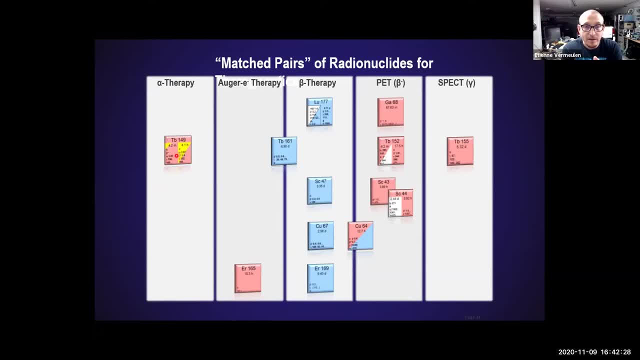 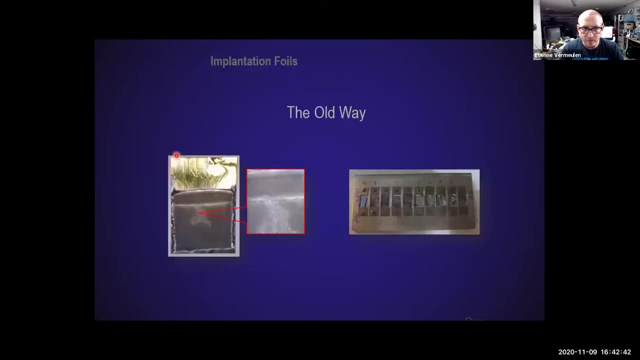 so it's really difficult to get them apart, And if you can purify them online and just drop them into zinc, zinc and terbium are easy to separate. So that's what we thought we would do, And first we tried some electroplated zinc. 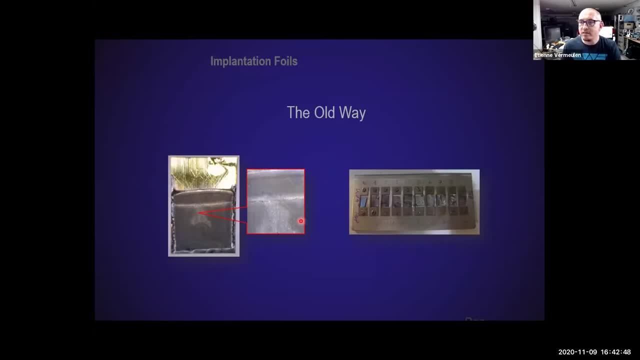 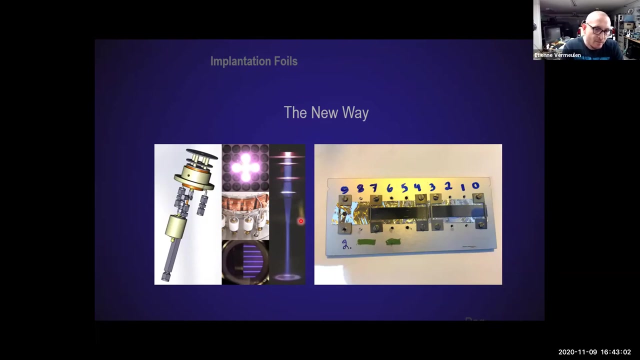 on gold, and this is using the cyanide method, so it's pretty dangerous as well, And we thought, no, this is really not the way to go. So there's a company in France, in Grenoble, that makes some incredible iron sources. 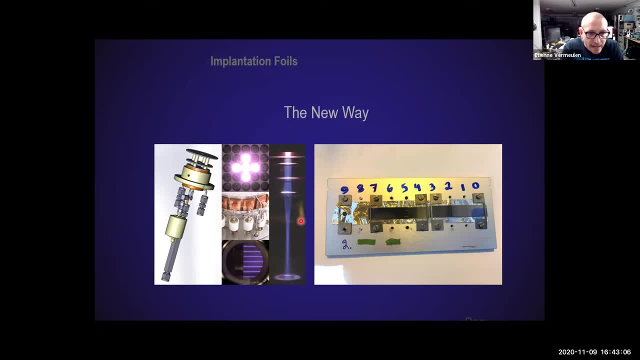 So we use an iron source that takes xenon gas and creates an iron beam of xenon particles and shot it onto zinc and put the gold foils next to it and made these wonderful, very nice gold-plated or zinc-plated gold foils. 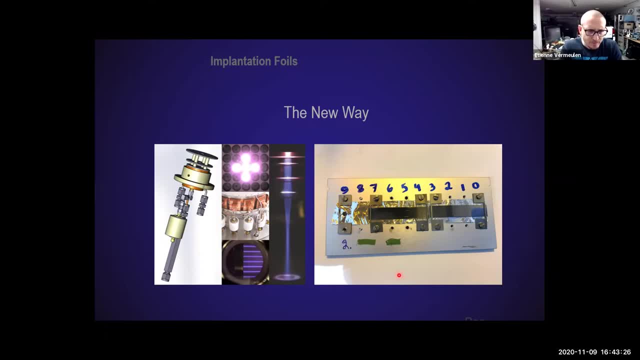 which supposedly were going to work very well. So we were shooting this in the middle of the night at CERN and for some reason we just didn't get any activity in the zinc. But when we counted the gold we had all of the radioactivity in the gold. 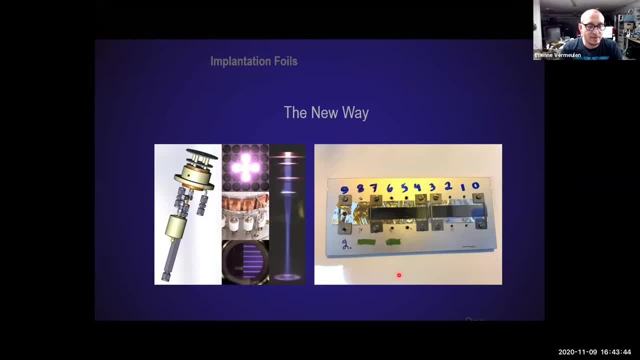 And you know you have an aha moment. in the middle of the night we were shooting terbium-149 at zinc, in the same way as we were shooting xenon at zinc to cause the sputtering, So we were sputtering the zinc away. 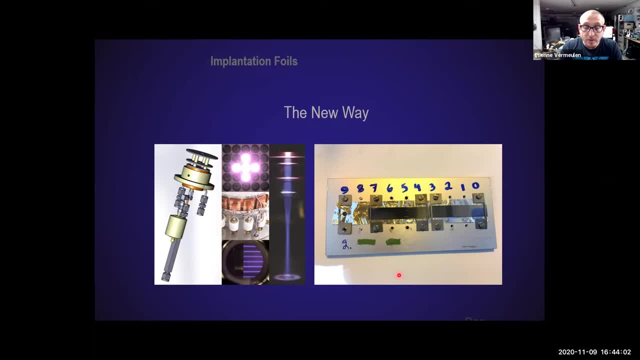 and embedding the terbium into the gold. Now all I can tell you is: aquaresia is your friend and you can dissolve gold, and if you have friends who are really good chemists, you can actually take those, those isotopes, out of the gold. 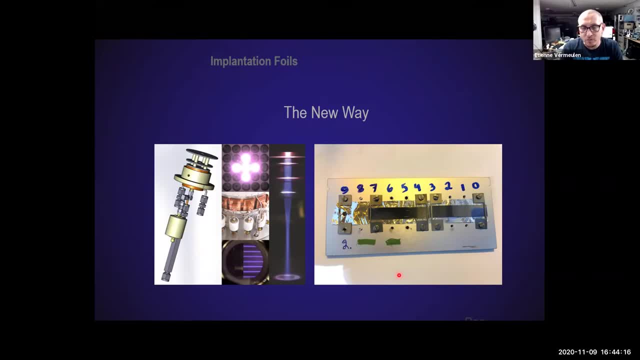 It's not ideal, and the answer to this was to move the beam up and down over this foil using grad students, because grad students make very good automated machines. So fair warning: every now and again you're going to be asked to sit through the night. 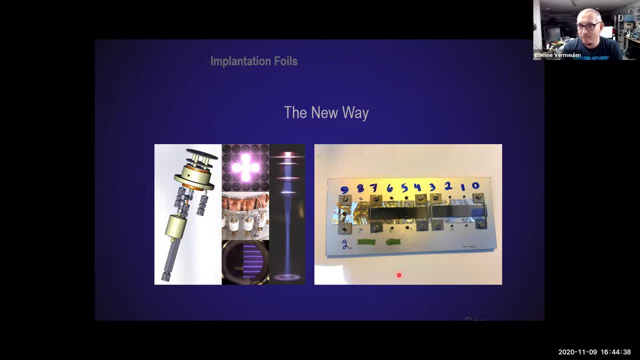 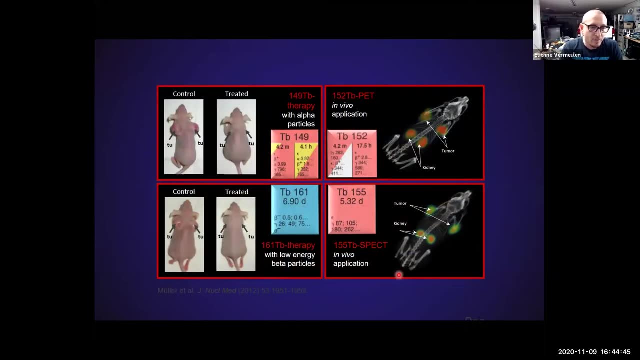 moving the beam left, right, left, right, But it means you get to do really cool things like this. So this is what we managed to do. We made terbium-149, and on the top left here you see a mouse that has. 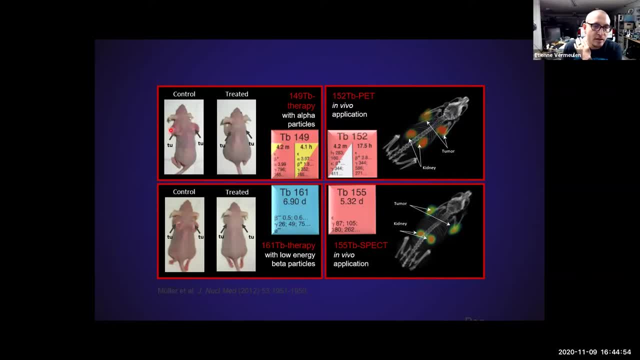 cancer on its shoulders and after treatment you can see the tumors have shrunk almost to nothing. So terbium-149 is a really good candidate for therapy. The problem is it's really difficult to make, So that's why you need a place like CERN. 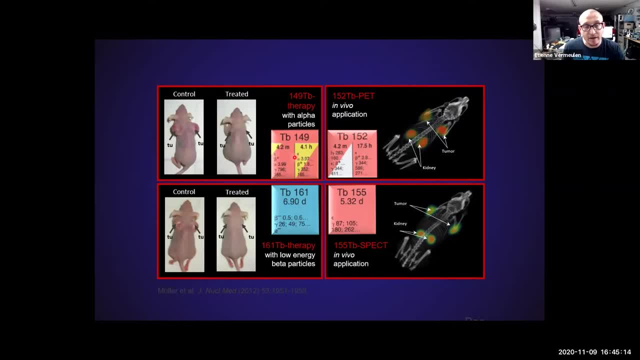 and we have to think about other candidates to do that. Now, in the terbium family there's actually four isotopes that allow you to do a multitude of things. So terbium-161,, which you make at a nuclear reactor, also has. 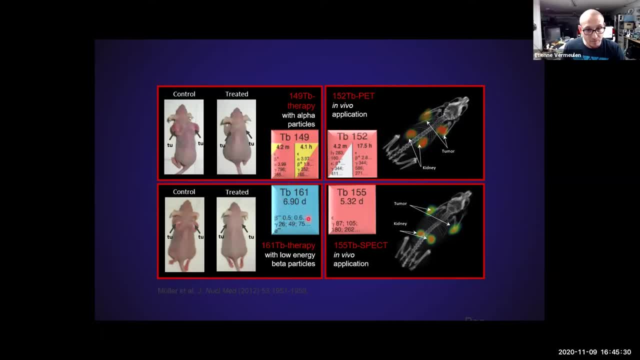 good results, and this is something that may be more easily accessible. And then there's two other ones that you can use for PET and SPECT imaging, so you can make these very nice images showing where the tumors are, how much there is. 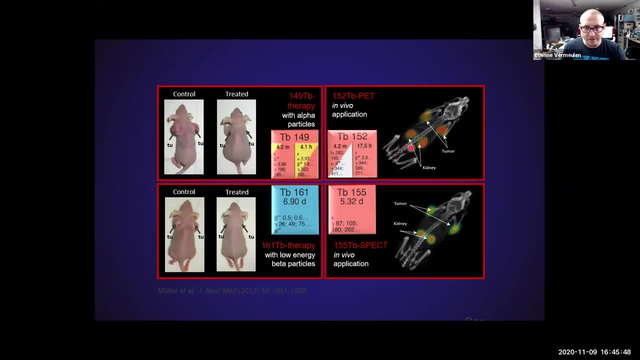 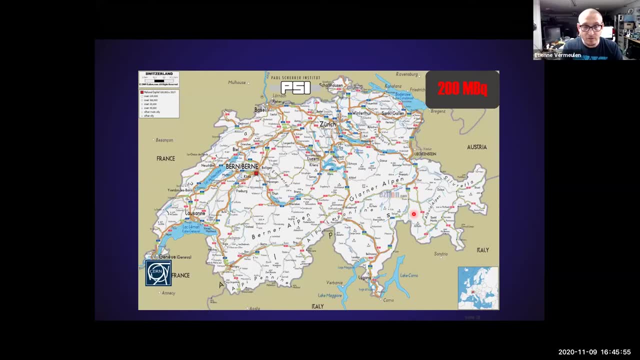 This is just in the kidneys, because everything has to go through your kidney to get filtered. So when we were doing these, of course, this is the other thing you have to keep in mind When you're working with short-lived radioactivity- you have to get it to. 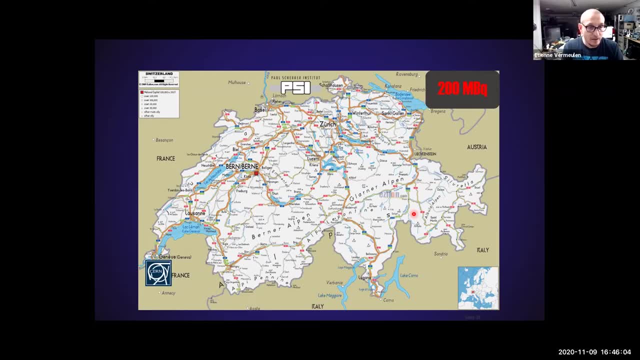 where it's getting used in an expedient fashion. So we were making the stuff down here in Geneva at CERN- and CERN is that circle you saw about there- And we were transporting it to PSI, which is up here close to Zurich. 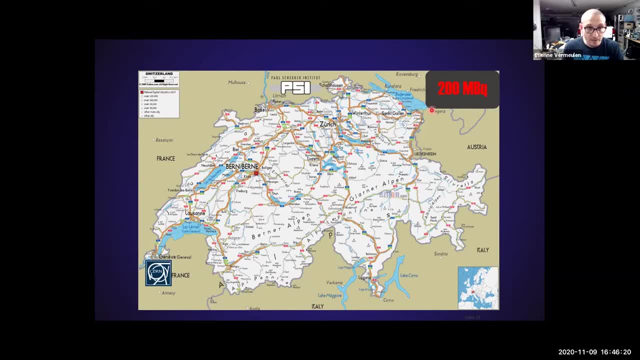 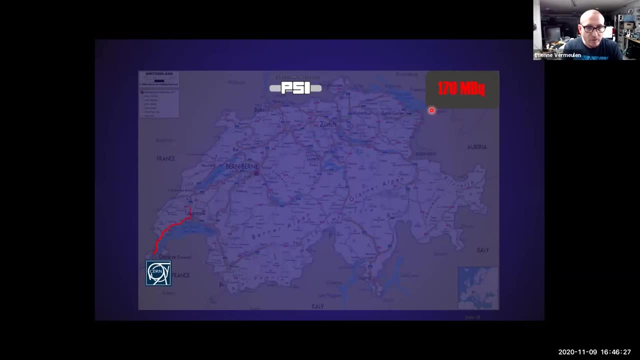 This is Switzerland, if you do not recognize it, because I don't think it says- And what we had to do is drive it by road and track the radioactivity in the top right corner there, all the way to PSI. do the chemical separation. 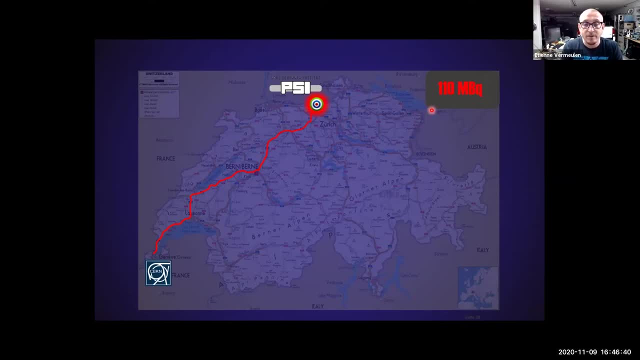 and get it into the mice with enough time and enough activity to be able to do this. So again, relatively short-lived. it shows the challenge of making enough of this stuff to get it into people. And remember that when we talk about Actinium a little bit later, But this 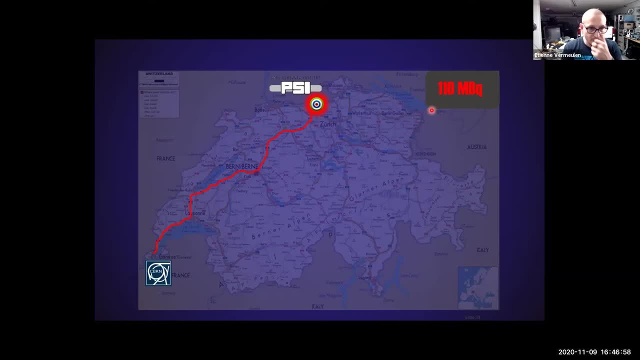 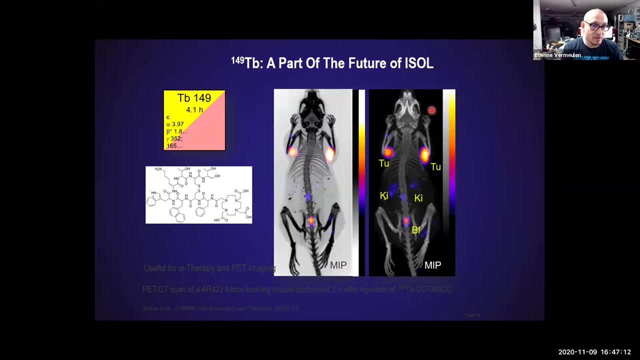 was a pretty exciting experiment. It was nice to do. We learned a lot. We figured out how to make radioactivity at CERN and actually get it offsite in such a way that we could do these experiments, And this was the result of it. So 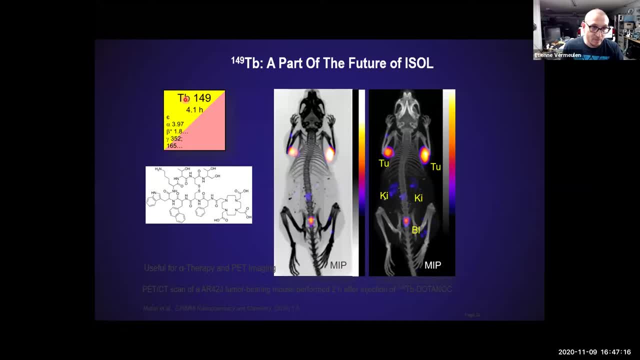 with Tobium 149,. as you can see, it's got a yellow piece and a pink piece, So you can image it and use it for therapy. And this is the very first PET image obtained with Tobium 149,, which we thought was pretty cool. 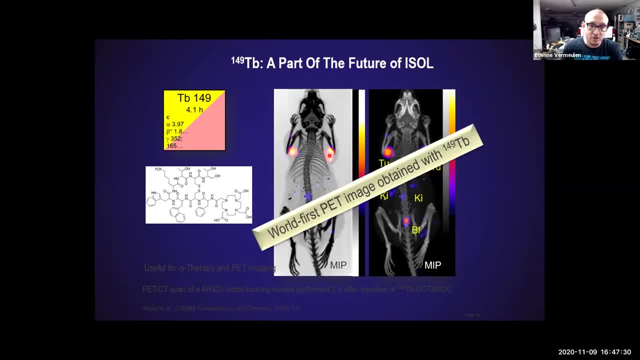 And you can see the tumors over there. You can see where the injection was done. There's a little bit of kidney showing up there And then these little spots is pretty interesting. So these are immunosuppressed mice, As you saw. they. 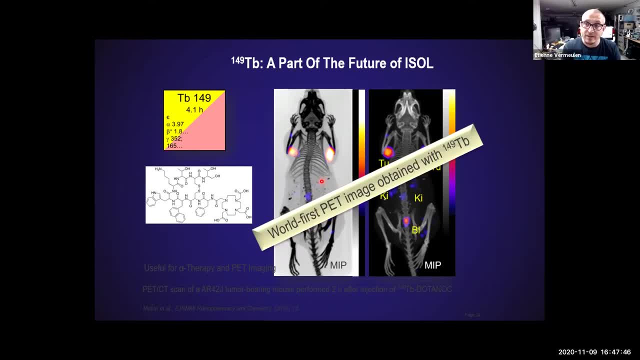 don't have hair on them, So they don't have immune systems so that they reject the cancer. because we put human cancer in these mice? But because they're immunosuppressed, they're also short on some minerals, So they eat their cages And these. 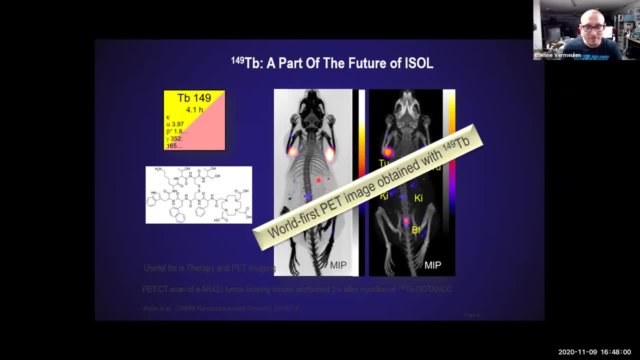 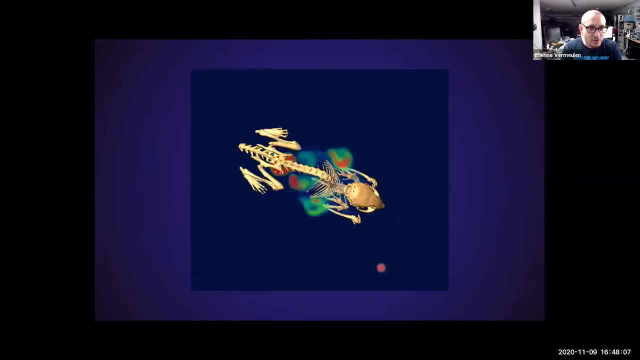 spots on the X-ray are. what you see are pieces of the cage that they actually chew off the sides, And if you have people who are really good at making these images, they can make something like this, And let's see if we can get this to play. 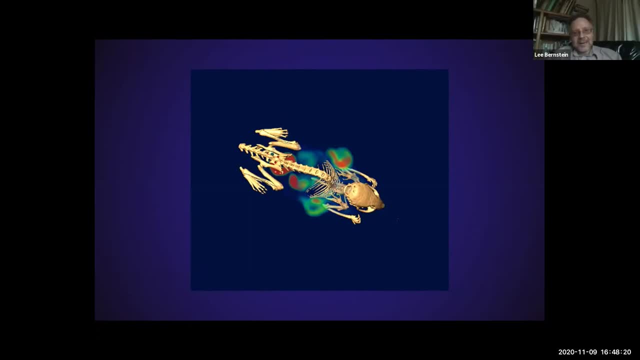 Maybe I have to change that. I think you have to turn off the laser. Yeah, There we go. How cool is that? So this is the type of thing we can actually do. So the skeleton is created with the computer tomography, the CT. 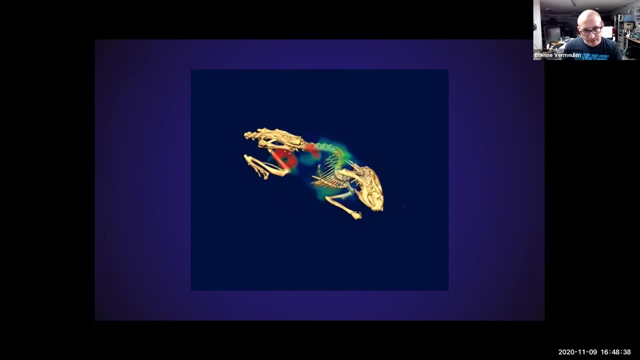 And then these ghost images that you see here are actually the PET images. So there's a kidney in there And then there's a mouse over the mouse's shoulders And that's the bladder, I believe, at the bottom there. So that's pretty cool. 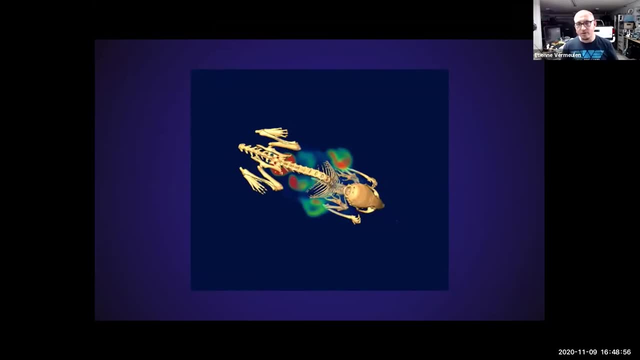 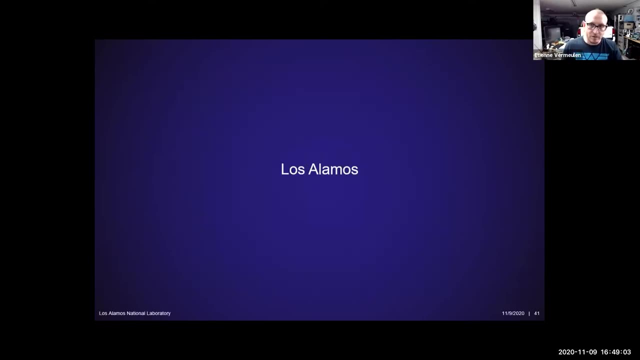 Okay, So we've sort of gone from Africa to Europe, And now I went to Los Alamos, And let's see if I can get my pointer back again. Los Alamos is another fascinating place. Here we do not have a cyclotron. 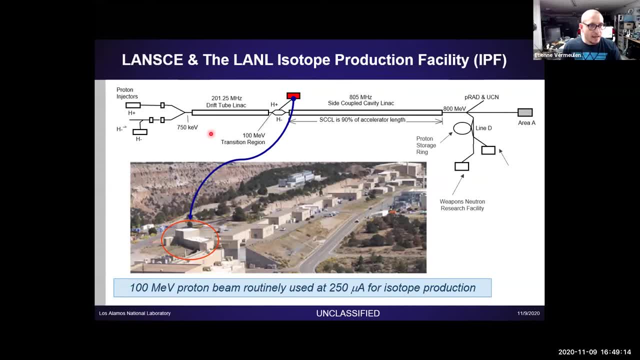 but we do have a linear accelerator And this linear accelerator is a kilometer long. So there's a corridor that runs from here to there And if you stand in here you can look down a one kilometer corridor and get vertigo. So if you're 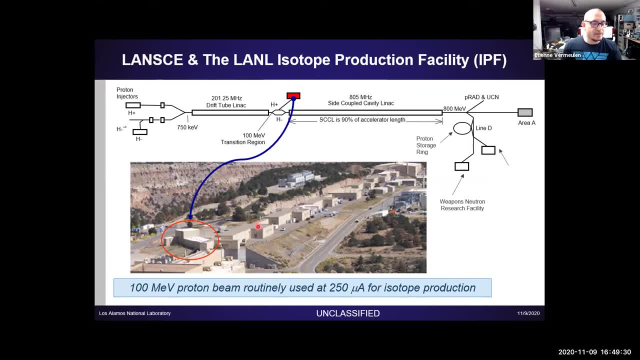 ever around at Los Alamos remind me to show you that It's pretty spectacular. The business end of what we do uses H plus ions, So this is a very interesting accelerator in that it accelerates both H plus and H minus ions at the same. 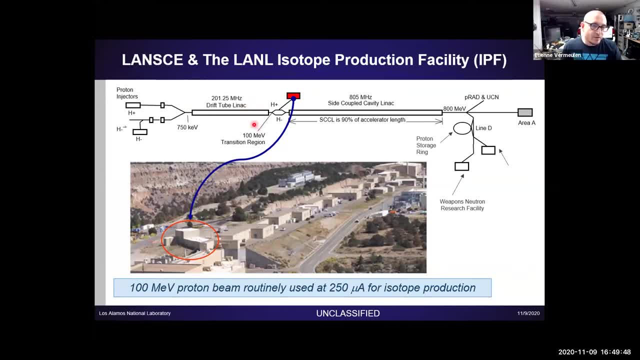 time in the same accelerator. Now, if you're pretty smart and you choose your magnets correctly, you can peel off the H plus at some point and the H minus goes along down here to all the other experimental facilities, And that's exactly what we do. 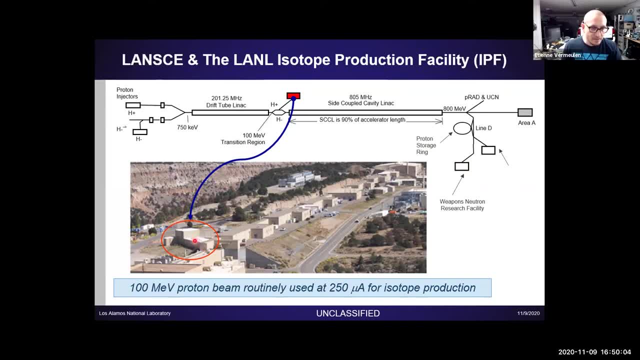 So at the IPF, the Isotope Production Facility, we can get 100 MeV protons, which are what this piece of the accelerator produces, And we can make pretty nice isotopes with that Down. here there's two spallation. 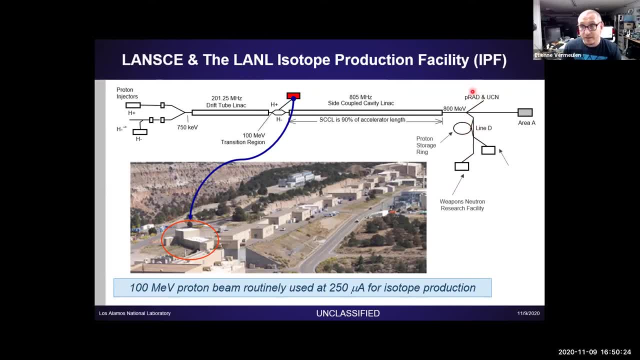 targets. There's also a proton radiography facility so they can do pictures of explosives and they can do pictures of T-Rex skulls. There was a fascinating study they did where they could look inside pretty much a rock that had a T-Rex skull inside it. 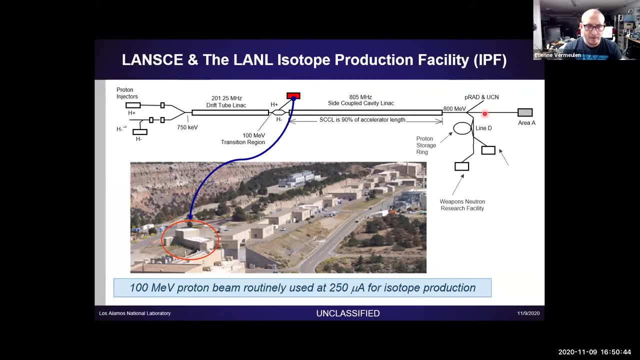 and they could tell by the size of the cavities in its brow how well it could smell. Those are really smart people. I'm not that smart. And then down here there's spallation targets that give off neutrons. They do all kinds of interesting neutron research. 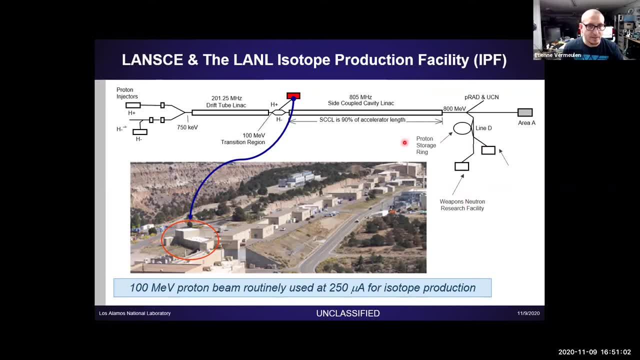 down here at the Luan Center or at the Weapons Neutron Research Facility. This accelerator is as old as I am- not as old as Lee, but as old as I am. So it was built in the 70s. Some of these pieces, 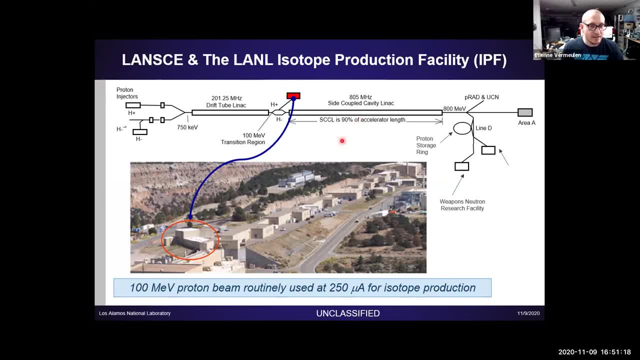 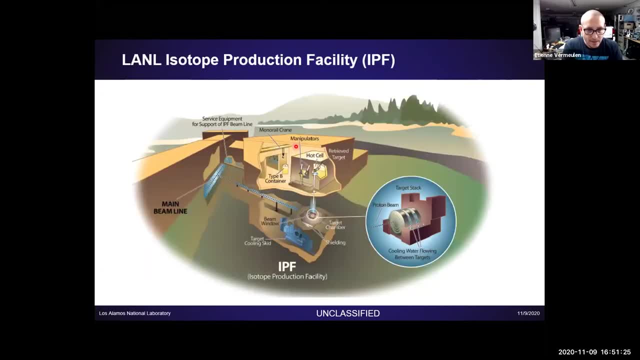 of this accelerator has been under vacuum since the 70s, So that's pretty cool too. But at IPF we have these hockey puck-sized targets, and now they're really the size of hockey pucks. They're about that big. We put three of them. 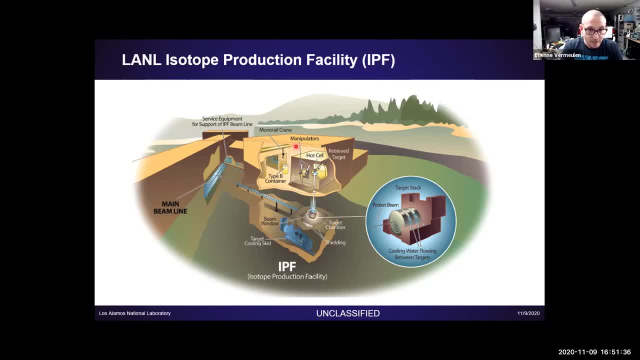 in a row because we have enough energy to make it through all three And we put them in a hole 40 feet down and very well shielded. So this is all concrete shielding down here, And then we peel off the protons and we shoot it. 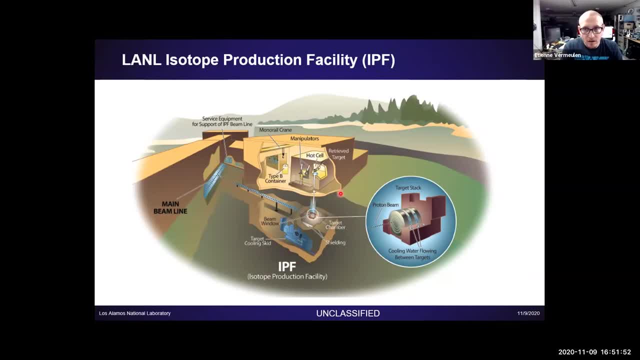 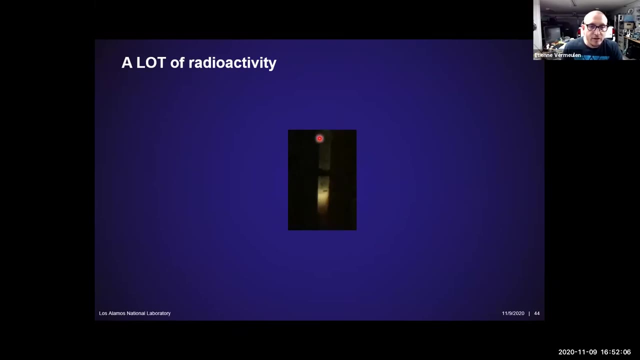 at these targets. Here we make very large amounts of radioactivity. So in the tens of queries, to the point where, if you turn off the lights in the hot cell and you take a picture, what you see here is an ion exchange column with about 12 queries. 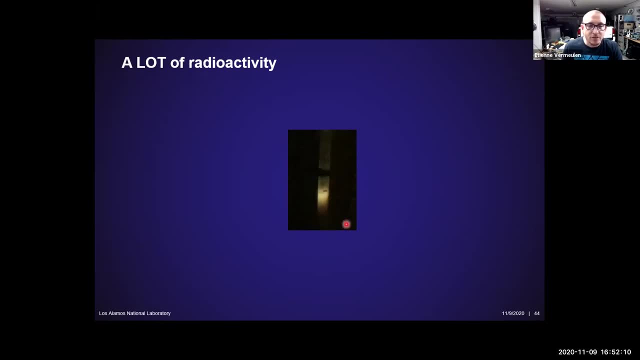 of strontium-82 that gives enough Cherenkov radiation to actually light up the hot cell. That's pretty cool. That's a lot of radioactivity, But the most important thing we're working on right now is Actinium-225.. 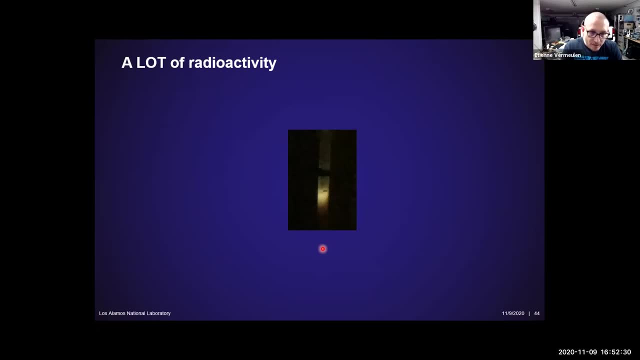 Actinium-225 is an alpha particle emitter that is probably going to be one of the most important therapy isotopes in the world, And the reason I say that is there's already been studies done with this isotope that shows it's very effective in. 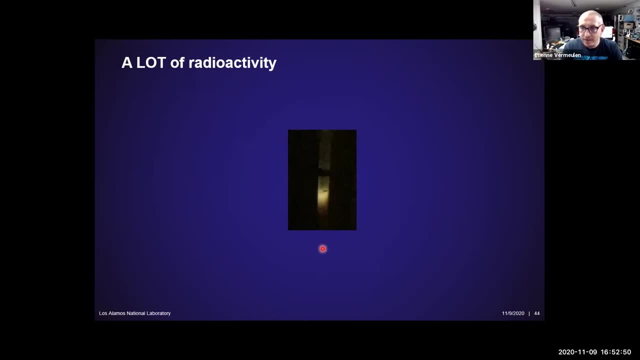 treating cancer And that's where I started. I'm pretty excited because one of the targets we built to make lots of this Actinium like this much we tested today and it actually worked. So that went really well. We didn't get that catastrophic. 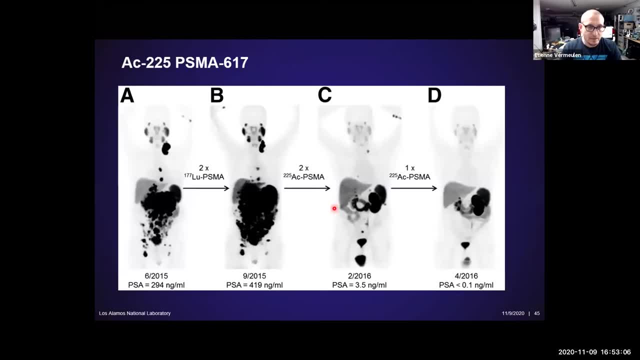 failure. But this is the reason Actinium is pretty important. Actinium, coupled to a molecule called prostate specific membrane antigen, seeks out prostate cancer and it will seek it out anywhere in the body. So this person you see on here is pretty much full of cancer everywhere. 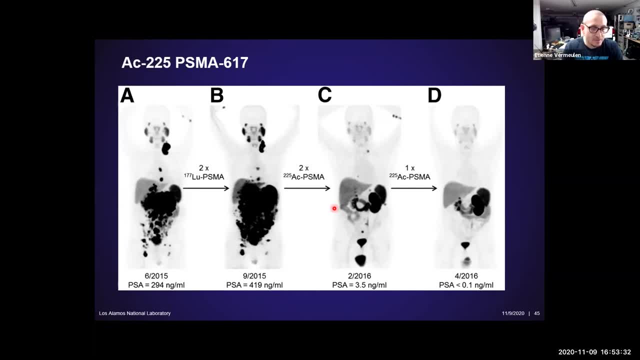 All those dark spots are cancer, And this person was treated first with Lutetium-177 that we met earlier, And it didn't really make a difference, As you can see. in fact, the cancer spread more. Then they had two treatments of. 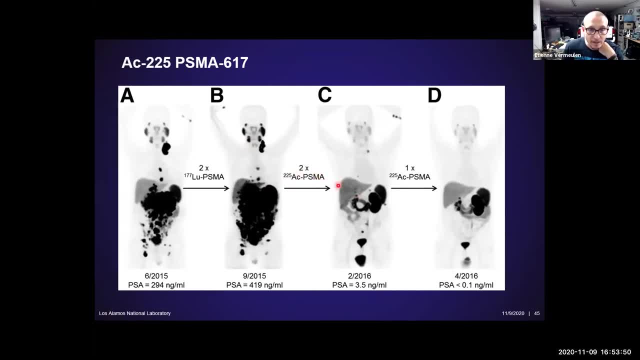 Actinium-225 with this molecule And, as you can see, it cleared up. There's a couple of lesions in the arm here, There's some in the neck, There's one in the bowel And then with another treatment, most of that cancer was cleared up. 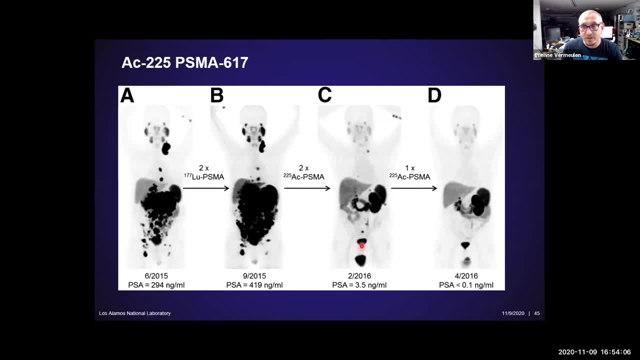 Now you'll see a number of these pictures as these studies come out. This is absolutely incredible And of course, there are side effects to these therapies, So the salivary glands, your tear ducts, things like that, get affected by this. 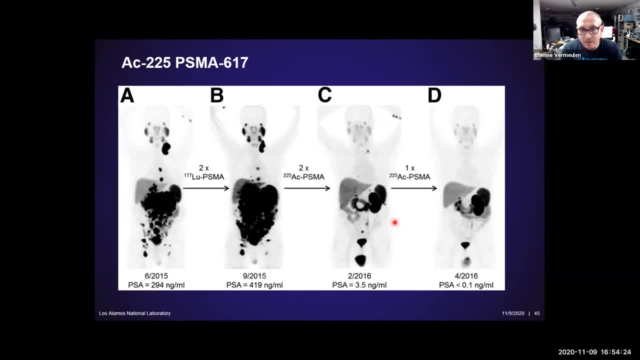 But the doctors are working on a way to manage that so that if you do have terminal cancer- and this person really was terminal- There was no hope to save this person And doing this, they probably bought them in the hospital. If you boil down what we do, 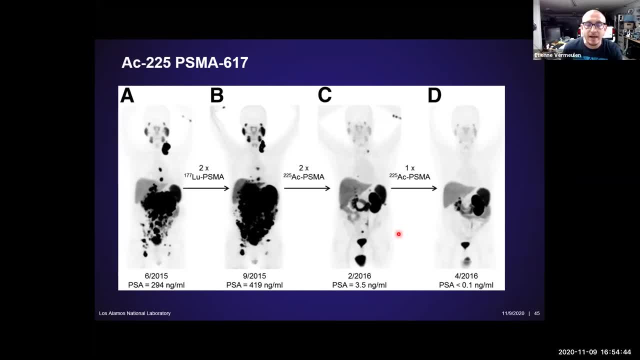 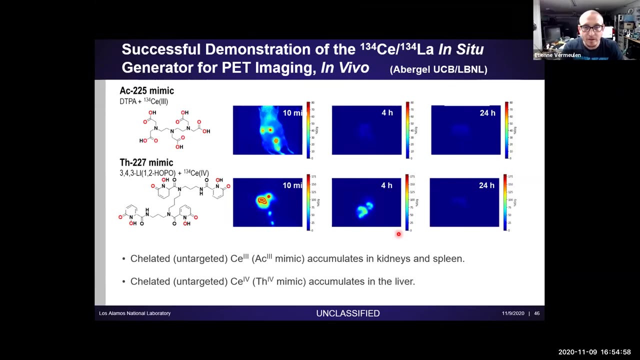 to what's the most important. this is the most important reason we make isotopes. Isotopes can really make a difference in the fight against cancer. So one of the things we did to bring the Berkeley's perspective in here is we collaborate with Professor Abagel. 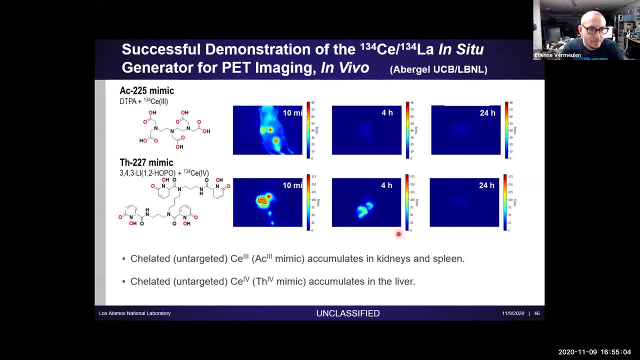 and this is a very interesting um application of chemistry. So cerium-134 is a very good mimic for both actinium and thorium, And the reason it's a good mimic is because cerium's got very interesting chemistry. Cerium is the only one of the lanthanides. 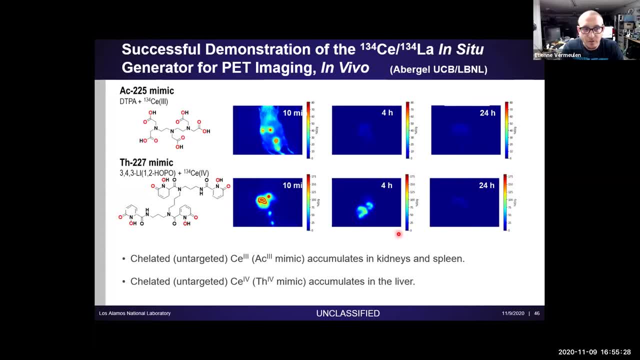 where you can easily create a plus four oxidation state, And by selectively changing the oxidation state we actually change the size of the cerium ion, so that in the three plus state it mimics actinium and in the four plus state it mimics thorium. 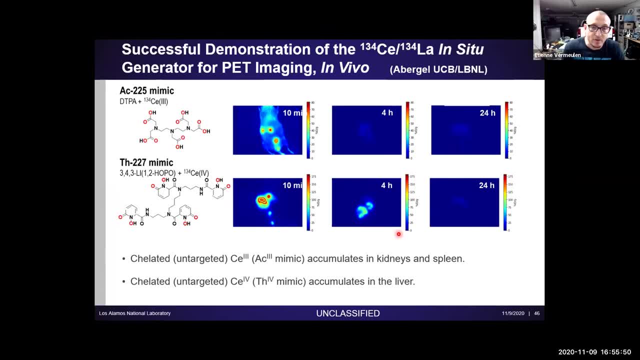 And you can do different work with it, And you can do these wonderful images, and I'm pretty happy that we managed to get this published in Nature. So again, congratulations, Rebecca. We're really happy about this. Um, so this is pretty cool, But we said we do. 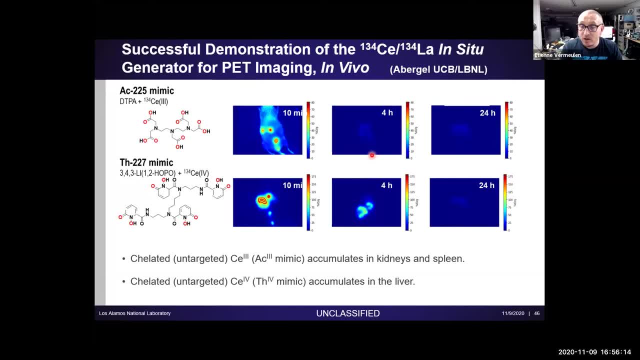 a lot more than chemistry and physics and biology. We also do a lot of engineering. So the most important engineering that we do is keeping these targets cool. Our targets get proton beams of the order of about a kilowatt per square centimeter. 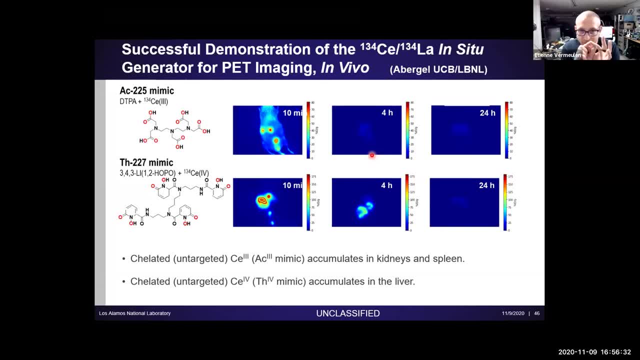 So just let that sink in a little bit. You have that much space and you're putting a kilowatt of heat on there, You're putting a torch to it and hoping it survives, And the way we do this and we keep this intact. 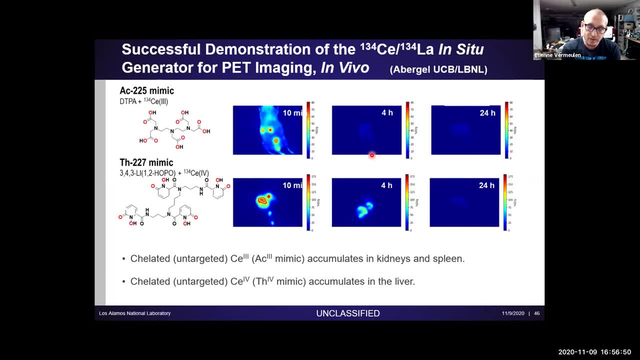 is by simple water cooling. And the reason we use water is because water doesn't activate, It doesn't become as radioactive as other materials, And you also don't break it apart. So you can say: well, why don't you use Freon? 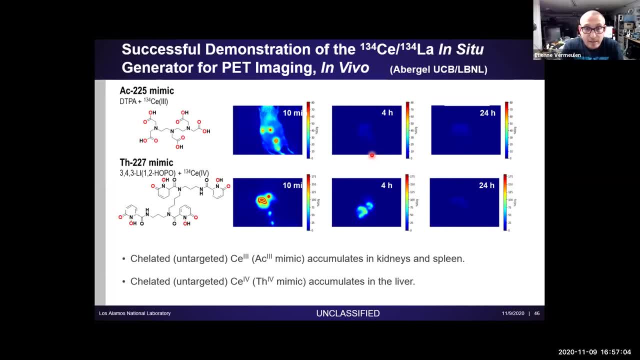 Freon is a much better coolant. Well, you're only going to shoot it Freon once and then it's going to fall apart, So we use helium. Helium is a really good coolant. Well, helium is really difficult to keep in a big system. 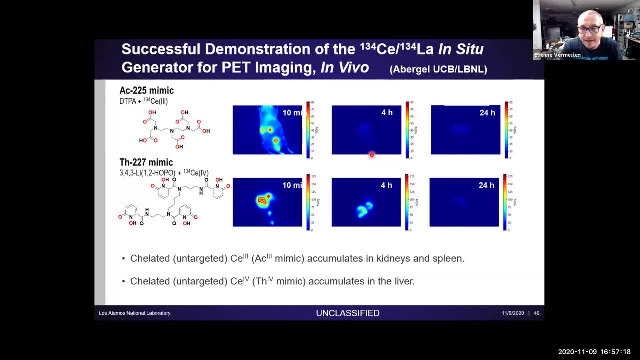 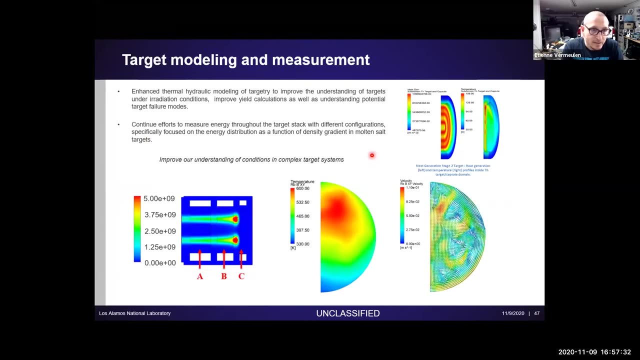 like I just showed you. It's a very tiny molecule and it's difficult to contain. And people do use helium, but they use it typically to cool the windows of isotope production facilities, not the targets. So we're stuck with water. So what we do is: 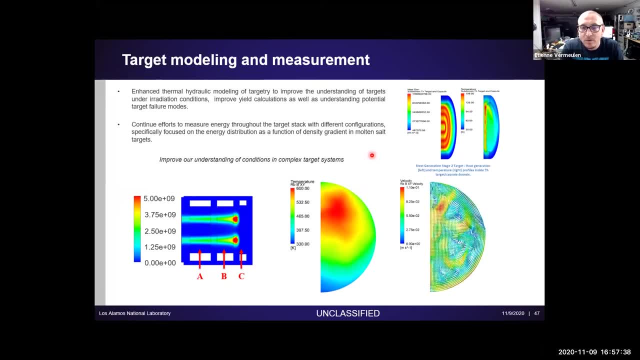 we model these targets extensively and how we can optimize the use of water. The biggest problem we have is boiling on the surface of our targets, because if you have enough boiling, it dries out and then you burn a hole and you're stuck with 16 slides ago. 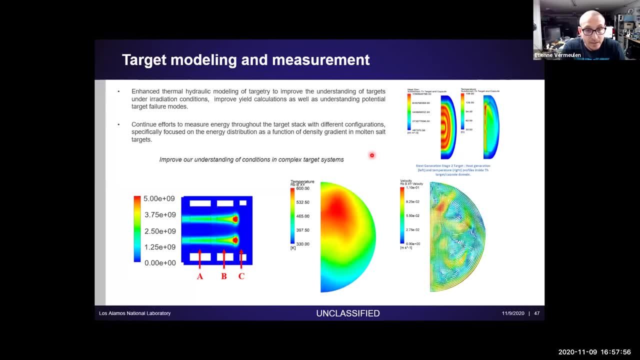 And this is one of the things we do at Los Alamos is we use ANSYS and we use thermal hydraulic simulations to create this type of simulation so that we better understand our targets. So, on the bottom right, what you see is molten rubidium chloride salt. 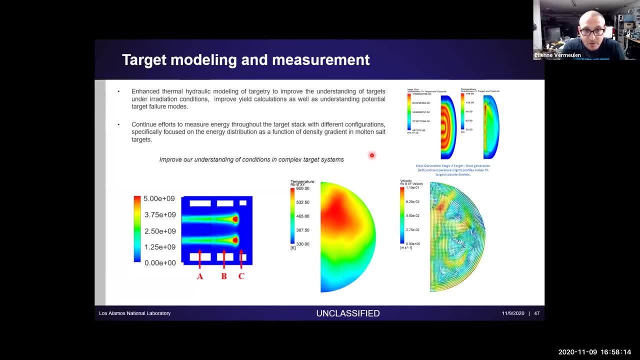 and you see the velocity and the temperature maps there On the right hand side. this is what the simulation says, how the molten salt moves around, and then on the left hand side. this is where we think the hardest part is. If you look at the target physically, 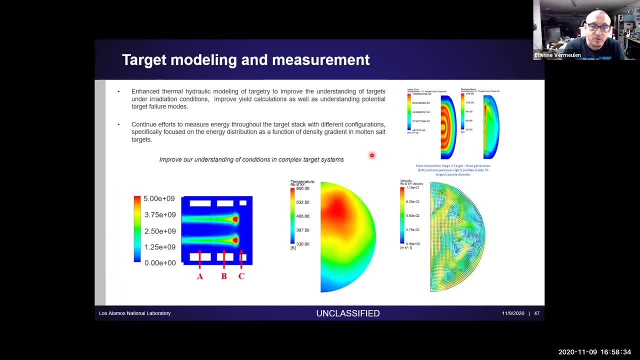 you can see these, what looks like burn marks on the target, and it correlates with the hot that is the hottest. The reason we see that is because hotter material is more buoyant, so it's going to move up and it's going to sit there rather than down at the bottom here. 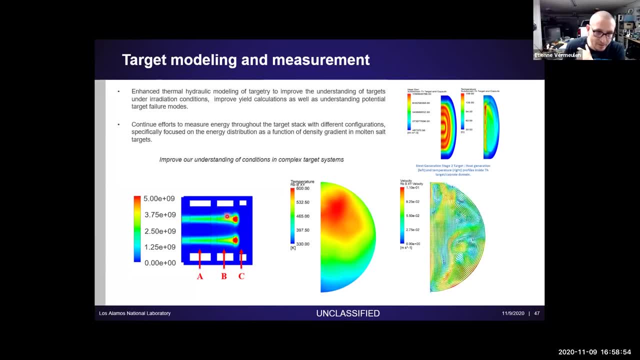 On the left hand side is a 2D model where you see the beam hitting the target and you can imagine this is a circle because, remember I said, we make our beam into circles. so that's the circle: going through and getting less and less. So in this simulation, 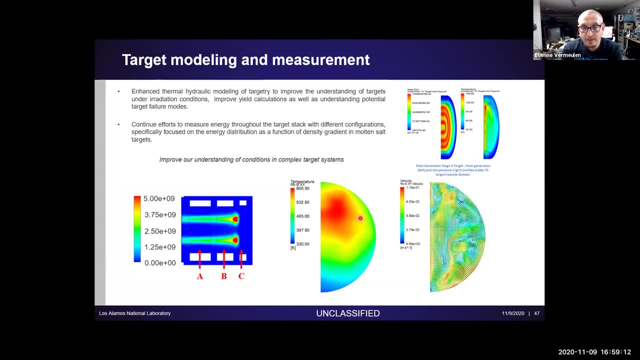 we have to do a complicated coupling of thermal hydraulics and proton transport. So we first run an MCMP calculation to say where the protons stop and what the source term is going to be, and we translate that back into ANSYS and we run a little bit of ANSYS. 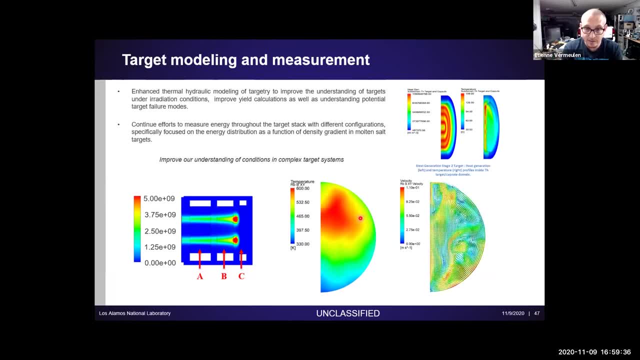 and we have a new picture of what this looks like. We put it back into MCMP and we iterate between the two to get this really interesting: dynamic simulations. At the top here is a solid target and that's three circles of beam so we can paint our beam. 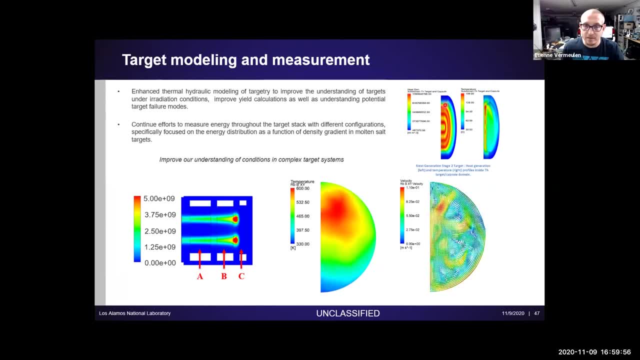 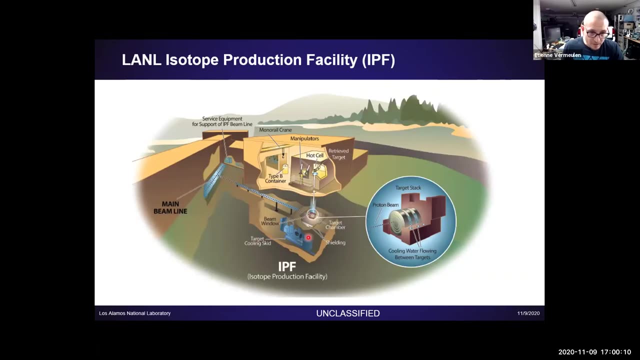 in many different circles, and this is the targets that we were actually shooting today. Beyond that, we also build experiments. Now, if you remember what IPF looked like, you can see that this target sits down here in a 40 square foot concrete block, and it's so radioactive. 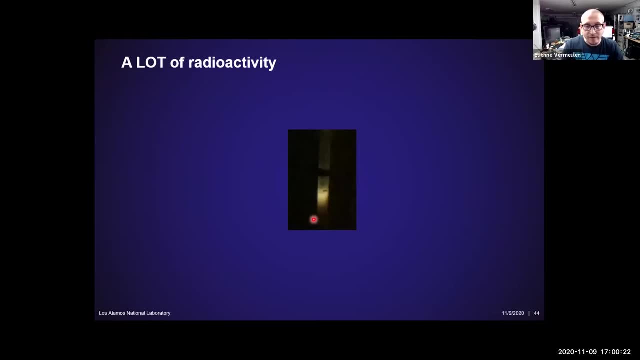 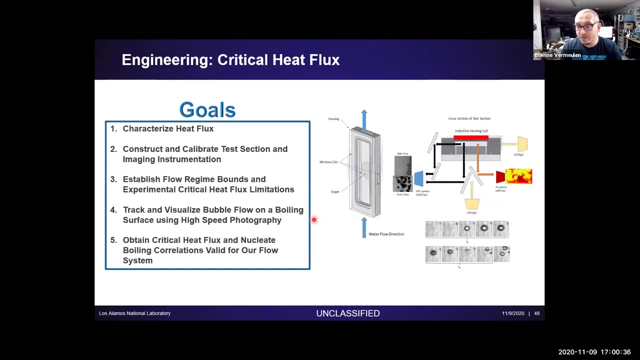 as you can see by that, that we cannot put a camera anywhere near that. Besides that, the people who built it built it such that it's impossible to get a camera down there, or any other diagnostics, to see what's going on. so we have to build experiments. 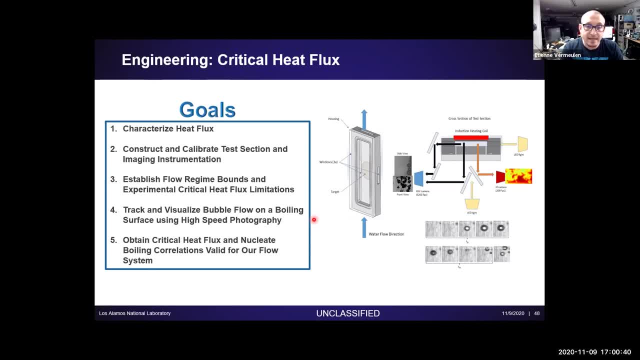 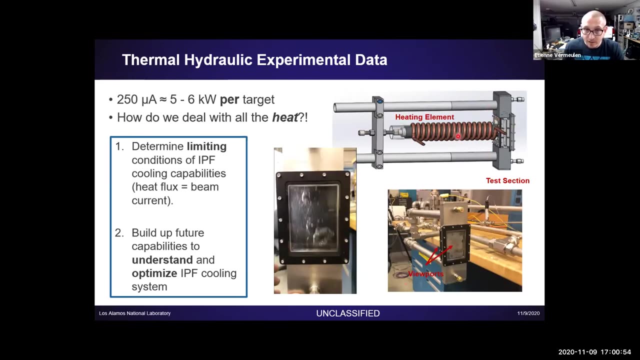 and what we're going to do right now- that's pretty exciting- is we're going to investigate how bubbles and boiling form in these cooling channels. So we've built a mockup of a cooling channel and that's what it looks like, and we have an induction heater. 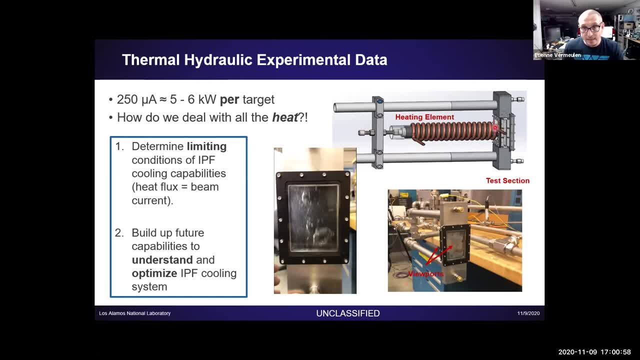 and we have a susceptor and we can heat this guy up to as hot as this window is going to get. when we heat it with protons That means this guy gets white hot. It literally makes stuff around it start to smoke, but it gives us the boiling. 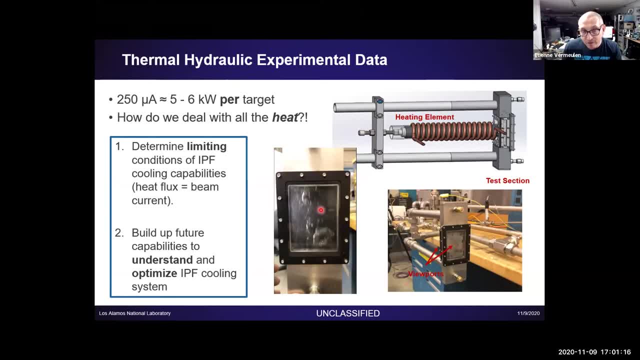 that we're looking at, and then we're using high speed cameras to very carefully look at how these bubbles are being made, how they grow, how they get broken up, and hopefully through that we can understand how to better cool these targets, because we've exhausted just using boiling. 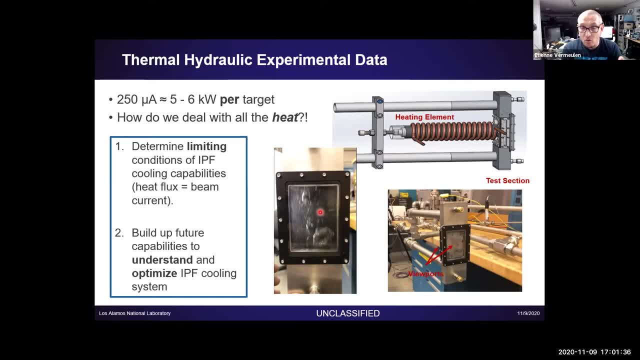 we now have to start moving the water around. so this may mean changing the surface. it may mean changing the way the water flows, maybe introduce more turbulence and remove those bubbles from the face of the target much quicker. and this is a very narrow range. it's either you blow a hole in the target. 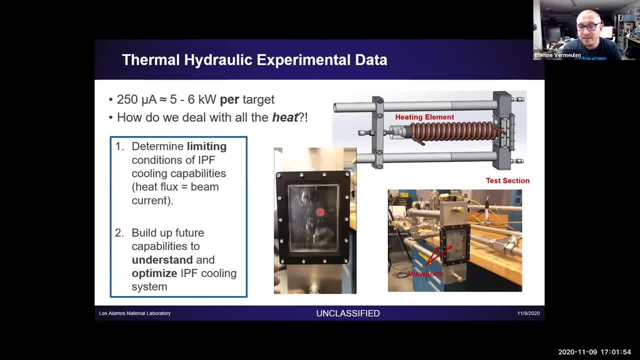 or you cool it efficiently. so this is really fascinating work and we get to do all of this engineering, we get to do the physics, we get to do that chemistry and separating all of those, and we get to touch the biology as well and we get to work with the. 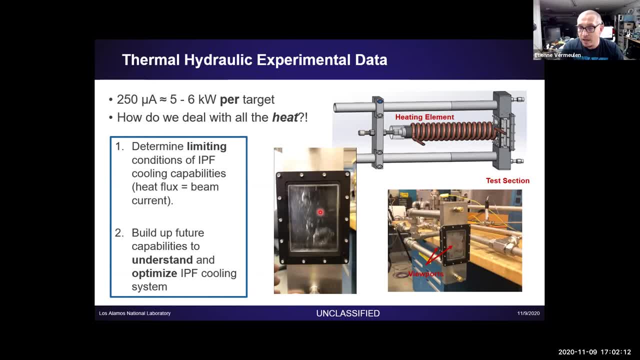 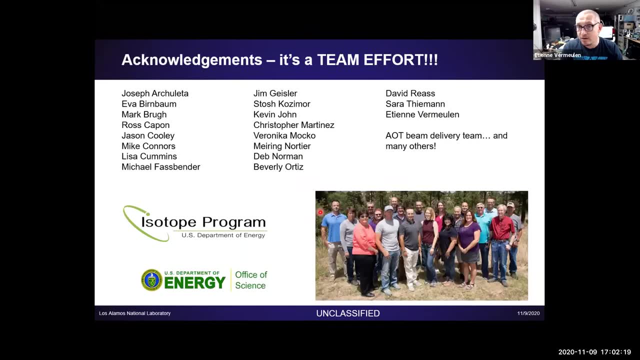 preclinical folks on these mouse studies. so I think with that I'm probably through all my slides. and, like always, these things are a team effort and we couldn't do it without our team and we couldn't do it without the support of the US Department of Energy. 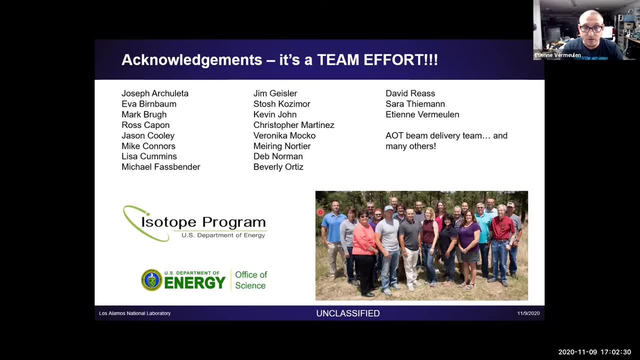 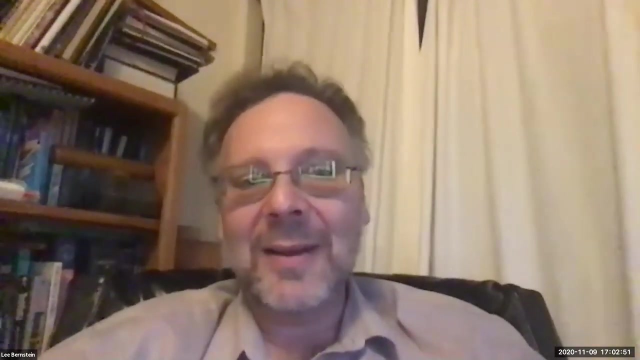 Office of Science and the ISO production program. so I think that's it. I will probably open it up for questions. Thank you very much, Etienne. that is excellent, really super exciting. so let's go ahead and ask questions. we've got lots of clapping hands in virtual space here. 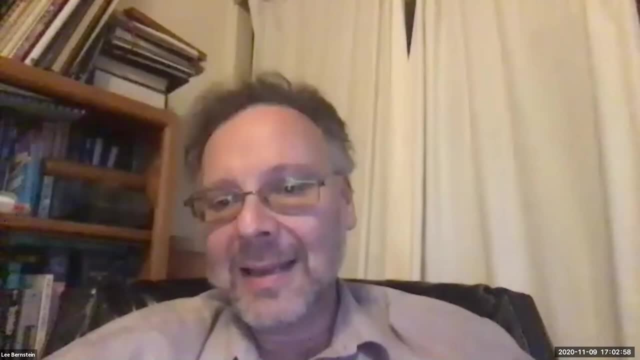 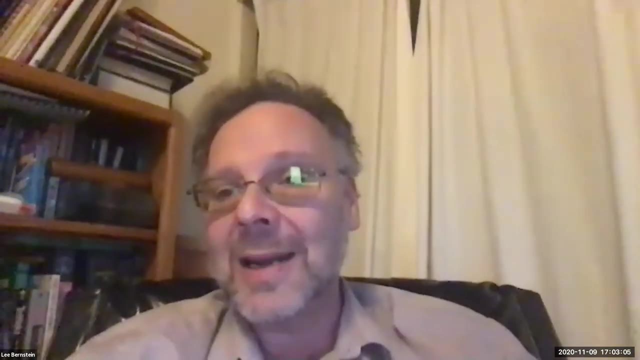 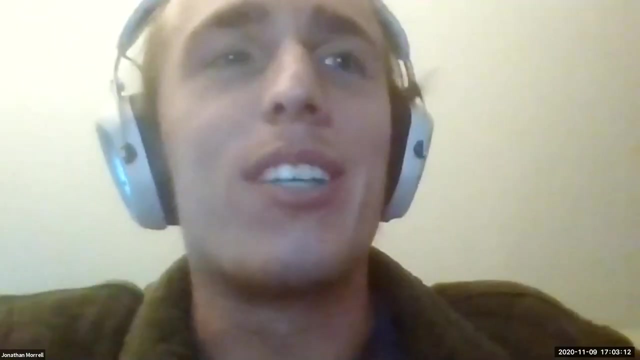 let me open up my participants window and let's take questions from people. please just raise your hand, or actually I think you can just unmute and speak on your own if you want. yeah, I've got questions, by the way. thank you so much, Etienne. this was really cool to listen to. 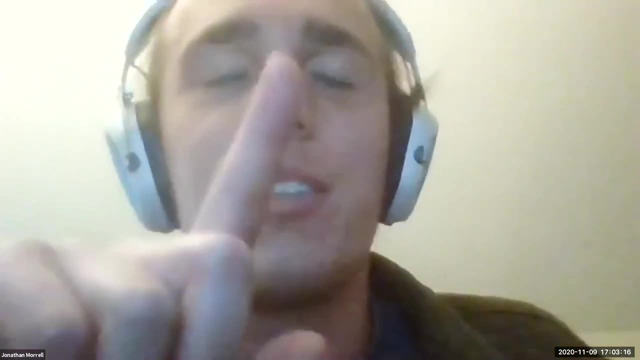 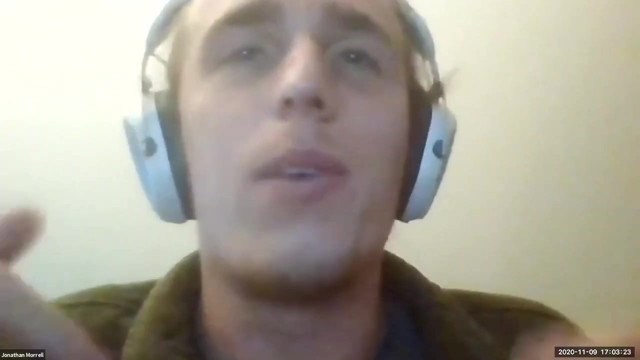 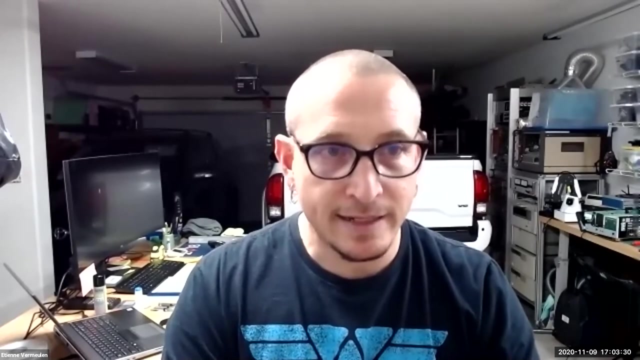 so I'll keep it to two questions. so one: you started at Atemba, but what, I guess, got you to Atemba Labs like, why did you start with isotope production? so I started my career as an analytical chemist. we involved, we just quickly changed. 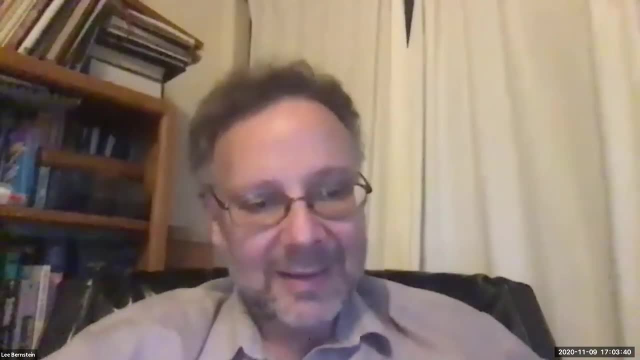 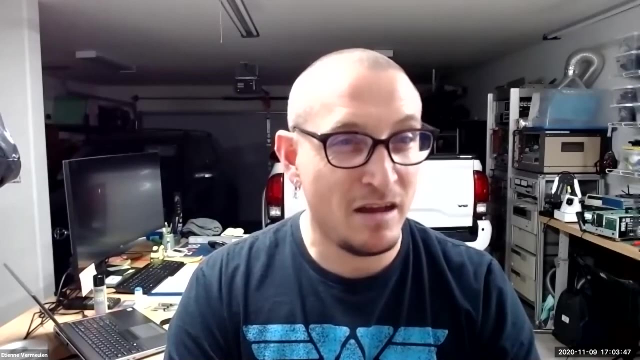 somebody's not muted. so one of the things analytical chemistry involves is chromatography, typically in HPLC, high performance liquid chromatography. so you learn about chromatography a lot, and one of the places we could go and work at was Atemba Labs doing quality control. 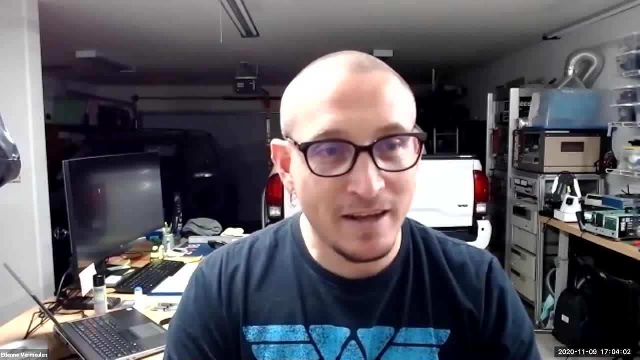 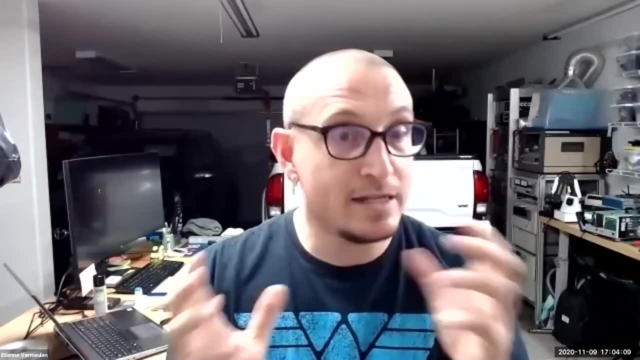 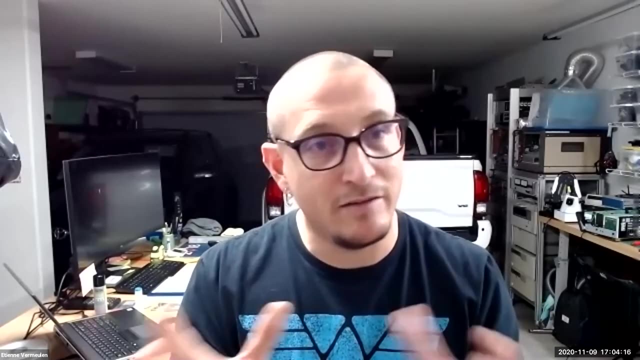 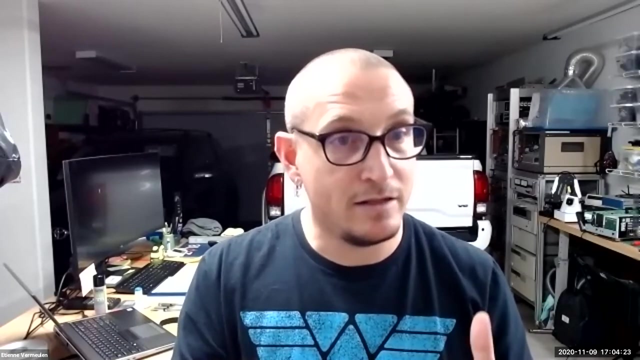 turns out that separating isotopes from targets also uses column chromatography, and that was the connection. so I started doing radioactive separations and one thing led to another and started getting involved in first the chemistry and the radiochemistry of separations, then becoming interested in the targets and then sort of 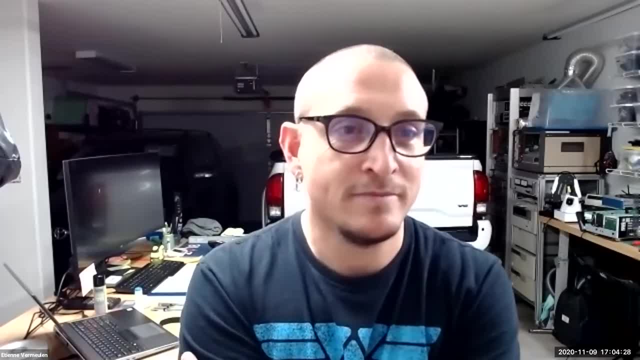 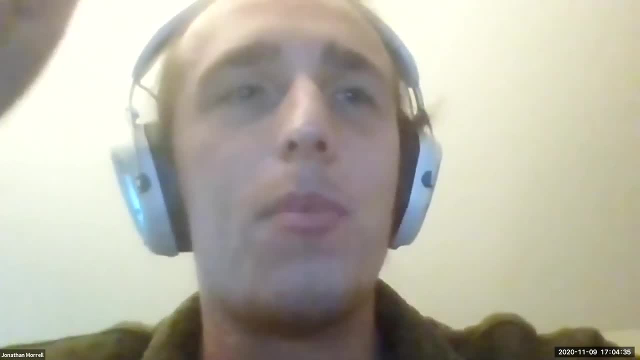 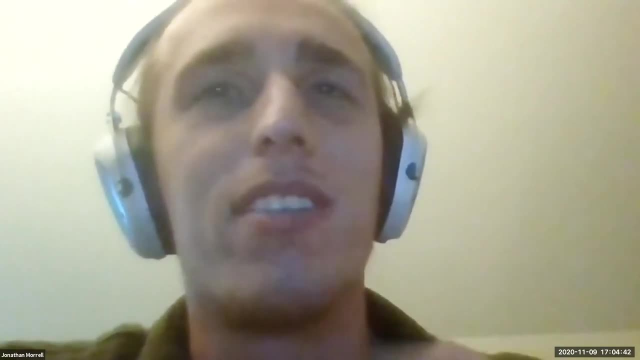 pivoting to physics after that. that's very interesting. and then my other question is: I guess how much beam could Lance give you guys? so I take it you're limited by your targets more than the beam we're targeted. target limited at the moment or cooling limited. 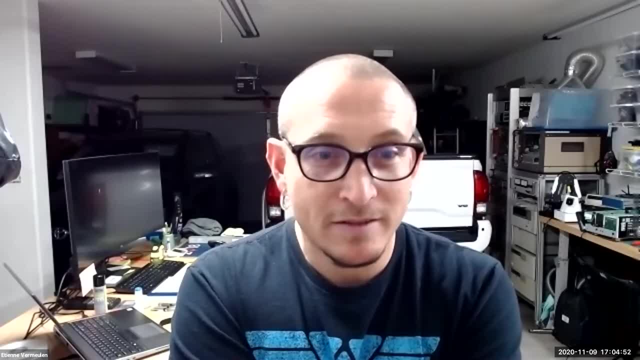 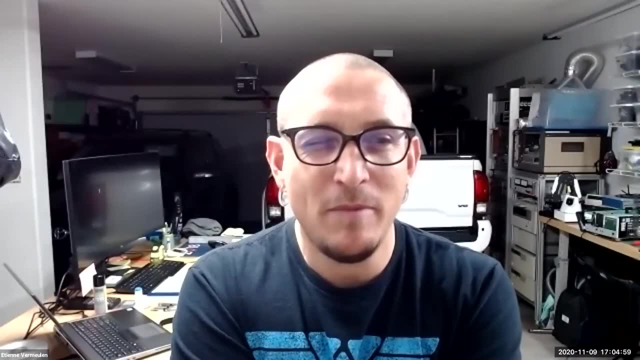 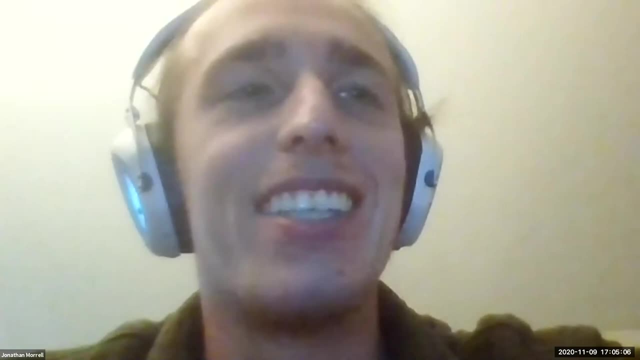 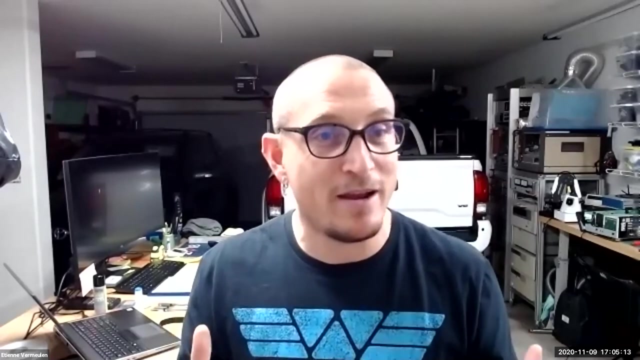 in principle, Lance can give us a milliamp of beam, let's do. that's probably about 10 kilowatts per square centimeter, so ridiculous, 10 megawatts per square meter, if you want to put it in that. so right now, if we run 300 microamps, 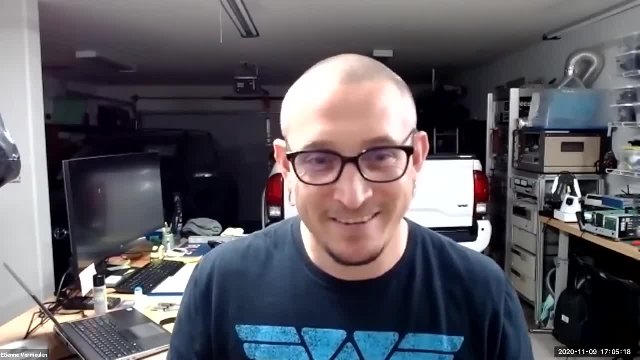 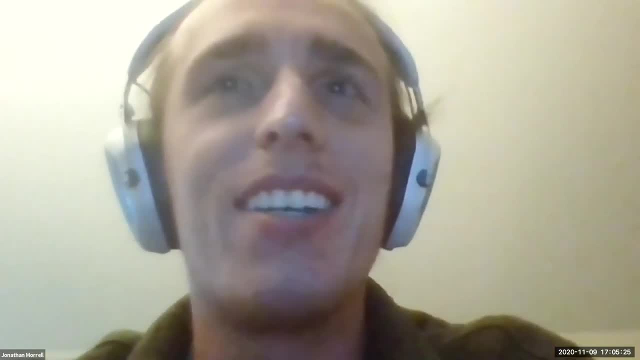 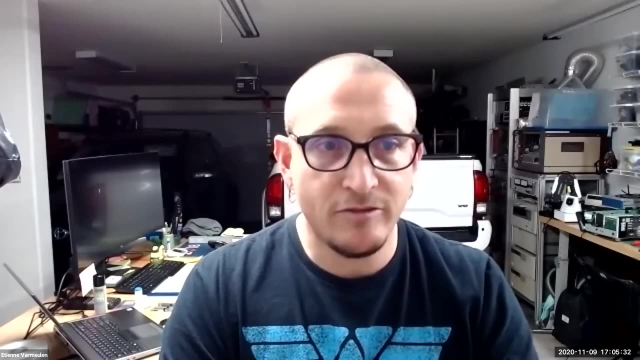 we're running 1 megawatt per square meter. that's like, I think, in fusion power plants. the limits they're operating at are like 5, so you're very close. so we deal with very much the same heat fluxes as fusion plants do they. 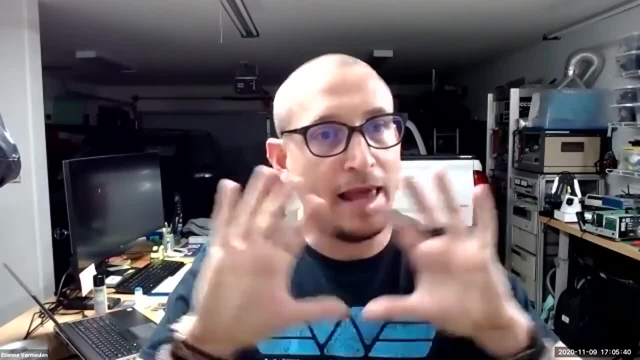 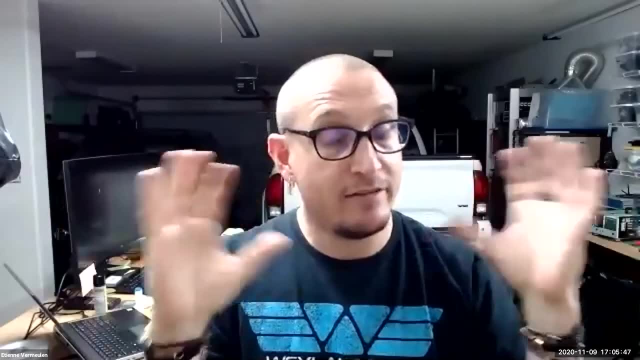 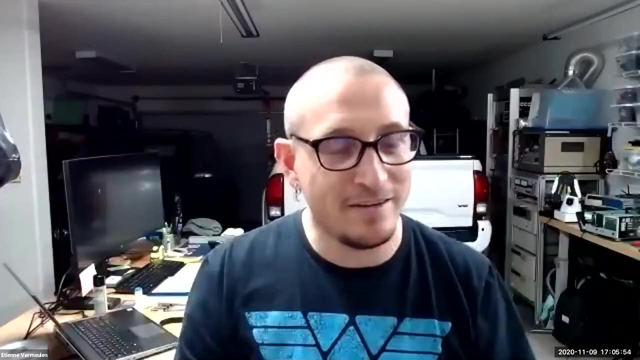 have a little bit more luxury than the blankets that are around the tokamak, for instance. if you look at ITER and the way it's built, what they're worried about is that first layer, and those are bigger than our targets so they can put more cooling channels in there. 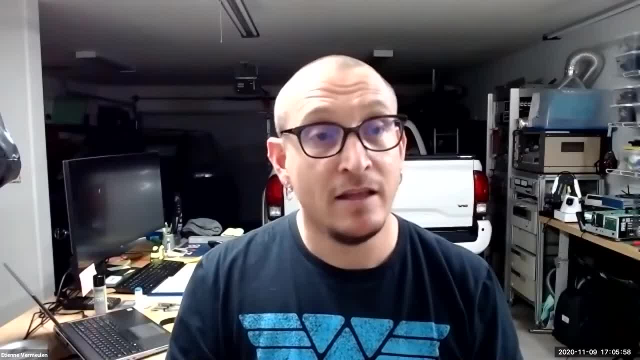 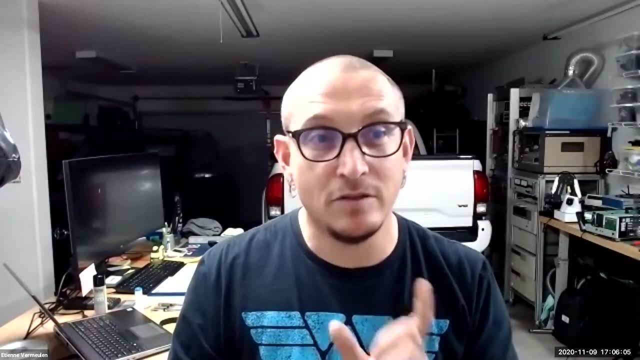 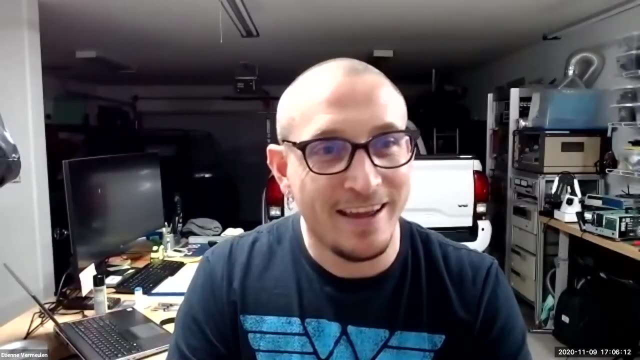 but it's similar sorts of heat fluxes. they do interesting things like hypervaportrons, and there's fascinating research being done to keep those connectors cool. but it's the same problem as we have: they have to use water and they have to make it fast. 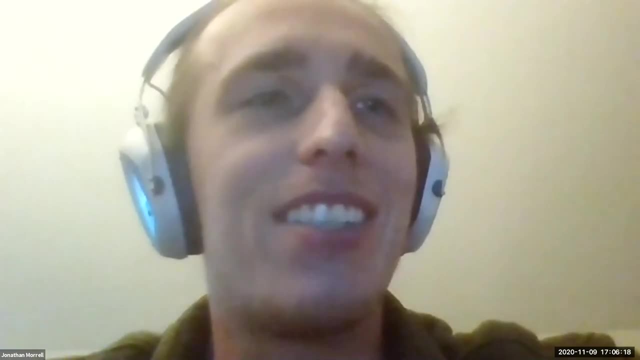 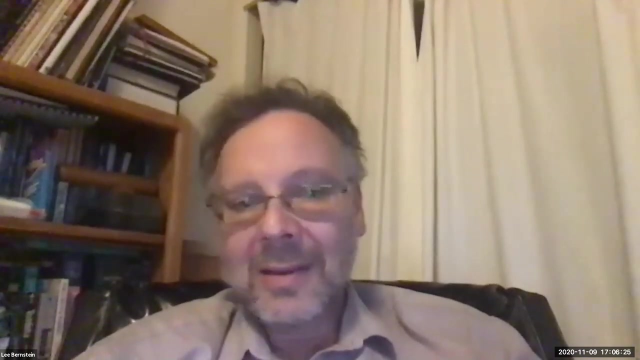 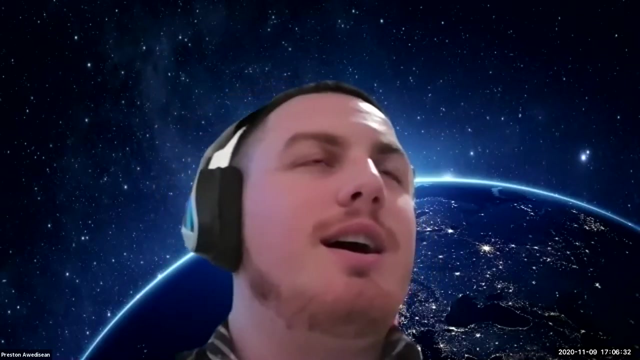 that's the way you do it: interesting stuff. thank you, cool. do we have other questions? I got a question. sure, go for it, Preston. hey, thank you again. in your opinion, what do you see as the future of cancer therapy with respect to the nuclear engineers in this call? 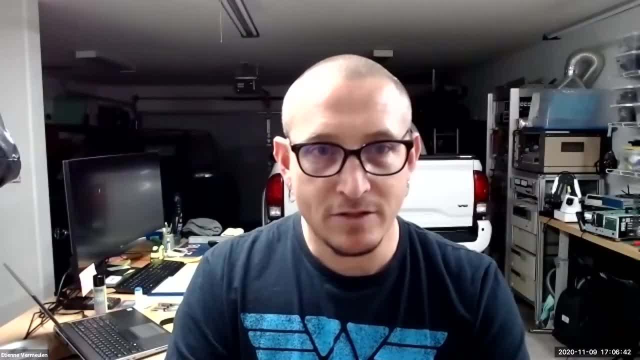 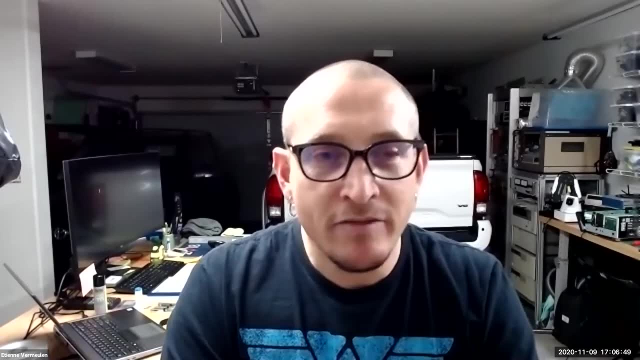 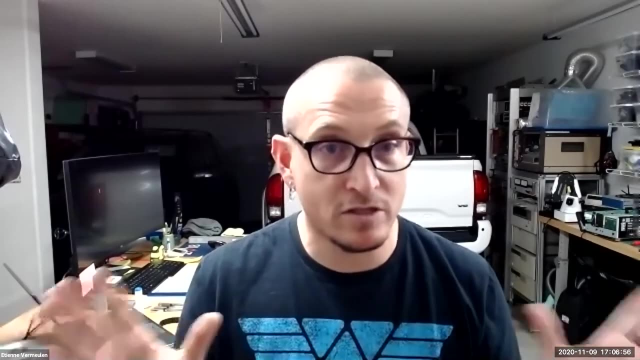 so one thing that's really important- and this is why I brought it back to you- 225- is there is not nearly enough of that in the world right now. the other important thing is, while there are a lot of small cyclotrons around the world, you can really only make actinium. at these higher energies. so higher energy, higher intensity, more heat, more engineering needed, and we do a lot of engineering in isotope production. most of it is done by nuclear physicists, so it's not the natural bent of the physicist to be doing engineering all the time. you really want nuclear engineers? 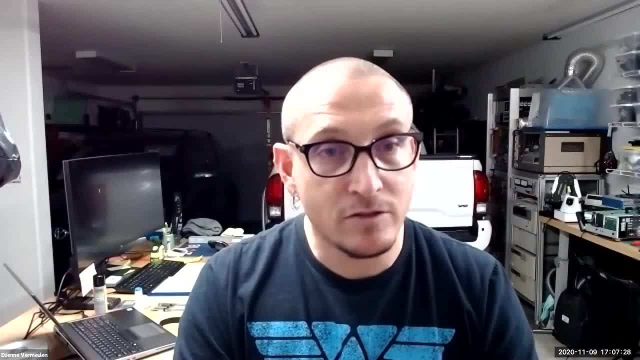 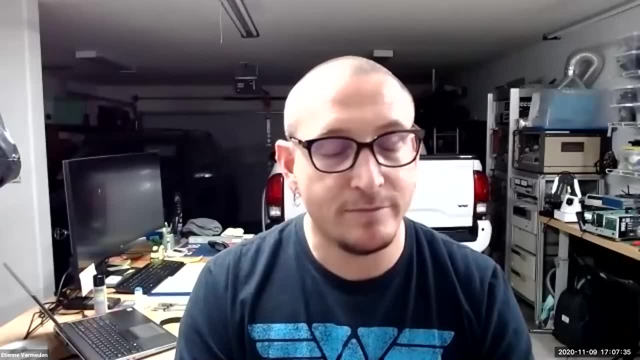 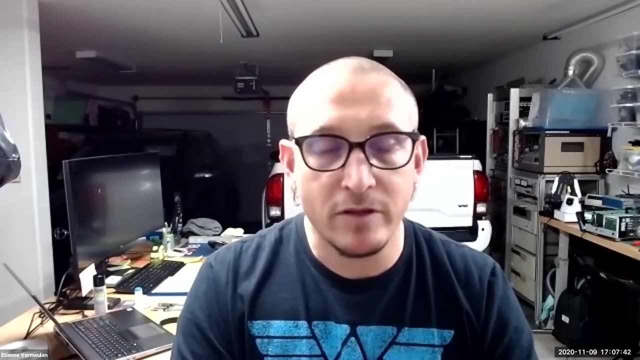 who understand this thing and who can do the thermal, hydraulic type of calculations and even the physics, so the neutron or the particle transport. I think there's going to be much more of a growth of nuclear engineers getting involved in isotope production, as we have to now push the frontiers. 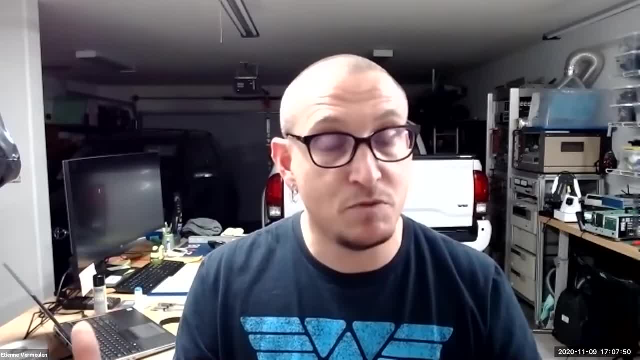 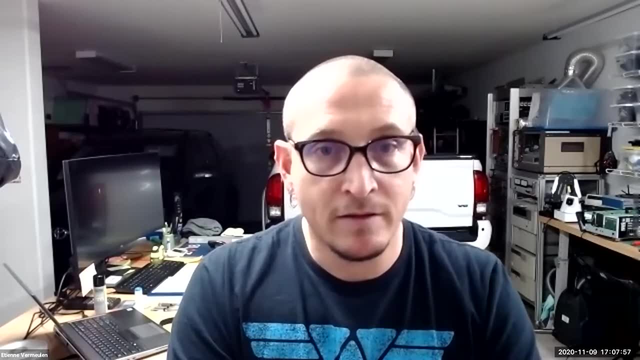 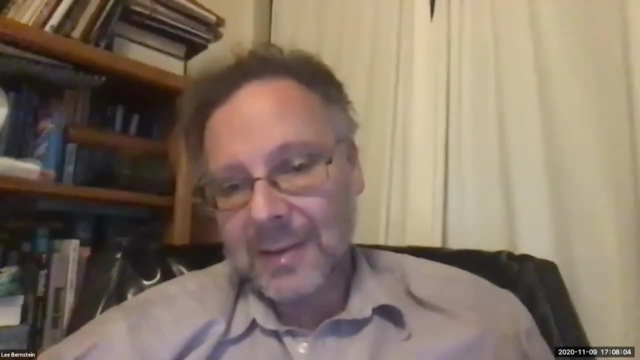 and push the limits of what these machines can do to make enough of the isotopes that are needed for the world supply. that's really cool and exciting. Saleem has a question. Saleem, can you go ahead and unmute yourself? yes, so I wanted to ask. 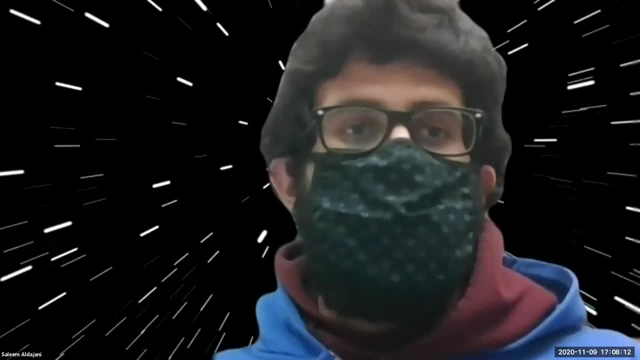 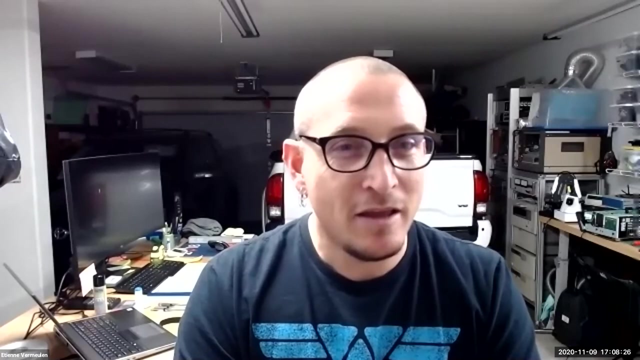 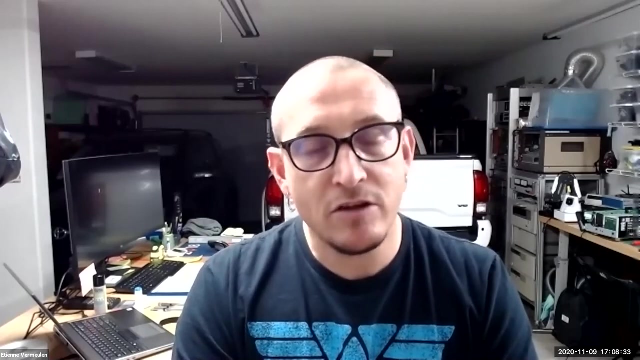 about the challenges. so why is making TB161 so challenging and why is CERN the only place where you can do so? ok, so it's TB149. so 161 is challenging, but you can make that at a nuclear reactor. 149 because it's so far from. the line of stability and there's such a mix of isotopes that you start off with. the only way you can do it is by having mass separation, and CERN is the only place where the energy is high enough to make enough of it to be able to separate it online. 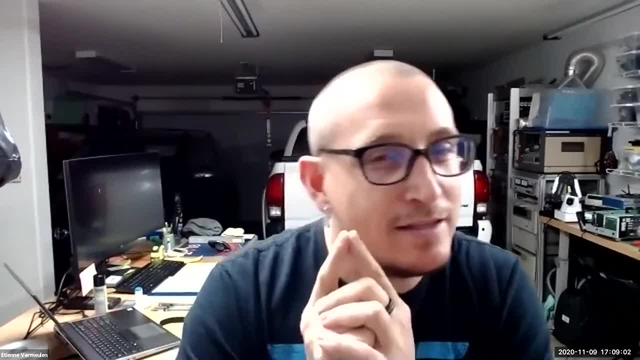 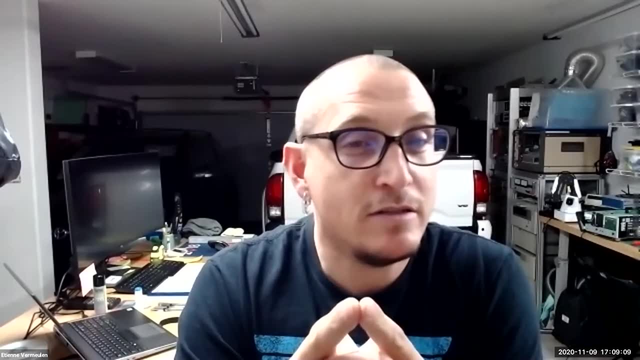 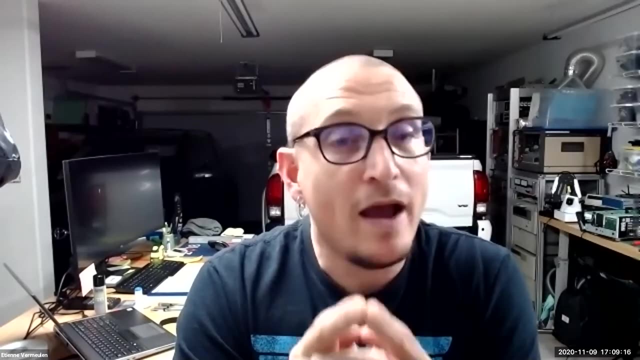 now there is another way that may work and this is for you guys to go and figure out. maybe if you have a lithium 7 beam and you shoot it at europium, you may be able to make TB149, and I think there's been a couple of experiments. 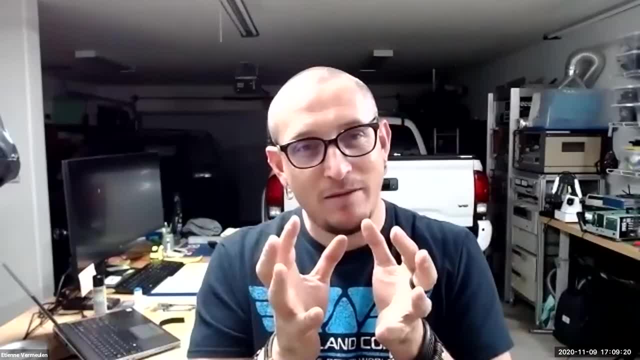 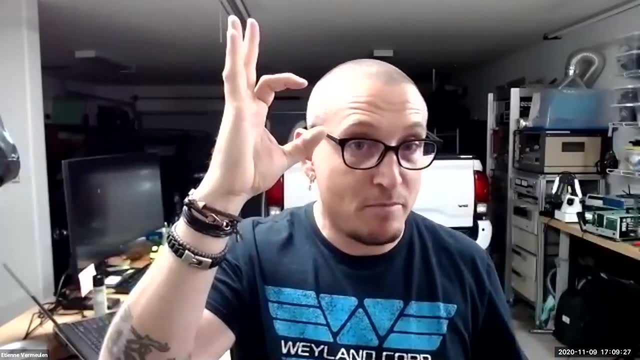 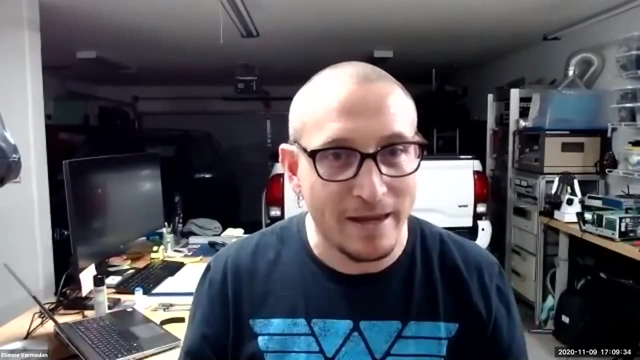 why hasn't it taken over? well, the problem with the lithium 7 beam is, if you get, if you want to get- high intensity, the beam starts blowing up. so you start getting a beam that's that big on a target that's that big. so that's the challenge with heavy iron beams. 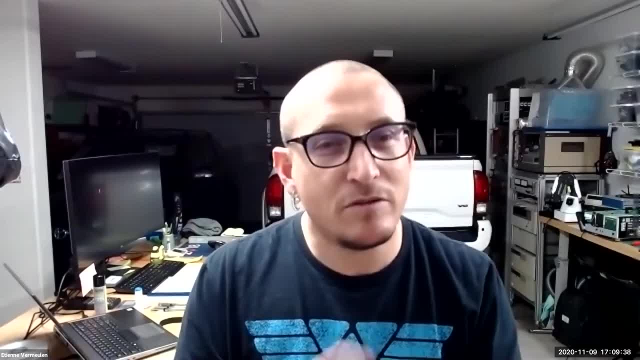 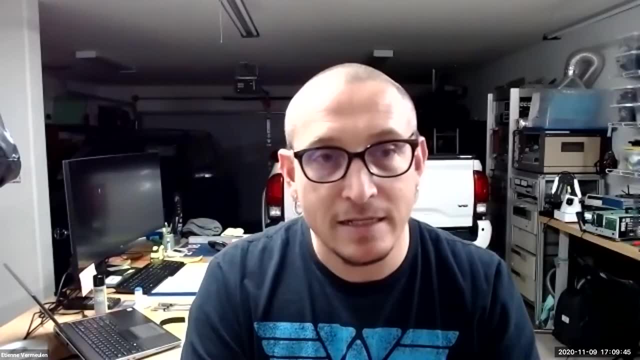 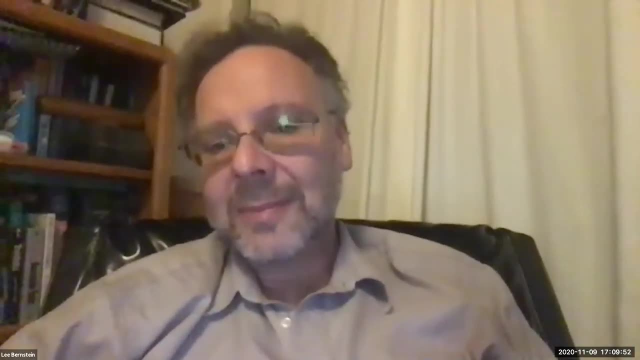 they tend to get too big, and it's something to think about for the future. maybe somebody can get a way to bunch those lithium 7s together in a better way, but the big reason is, the energy is just not there. thank you, Tyler, you have a question? 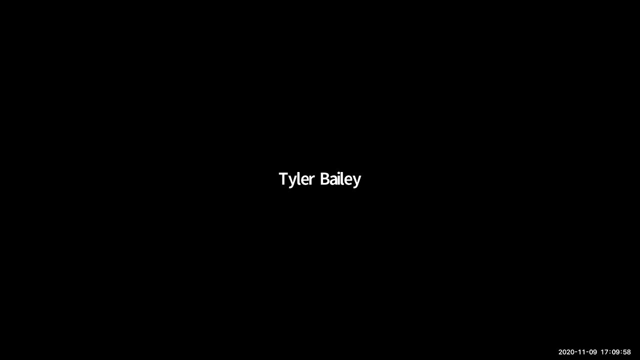 yeah, hi, Etienne, you had a very interesting slide on matched pairs. my particular focus has shifted on the Turbium 155 in particular. I was wondering: have you considered using it for Auger electron therapy? probably because there's a good chance it has some Augers as well? 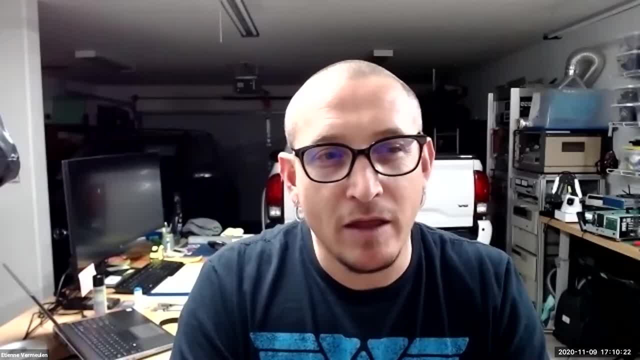 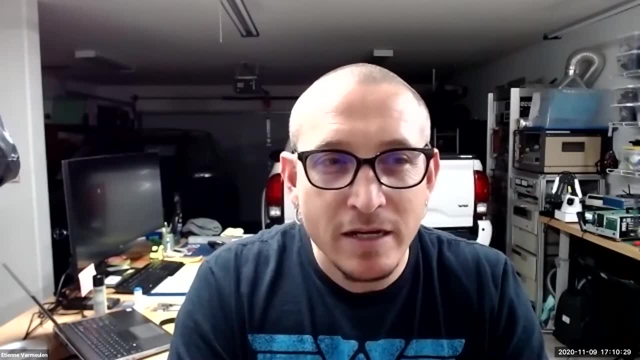 um, I think. I mean, we haven't measured it, so one has to go and figure out if there's enough Augers there. the one downside of Turbium 155, though, is it's got a lot of gammas, so you're going to get a lot of gamma dose. 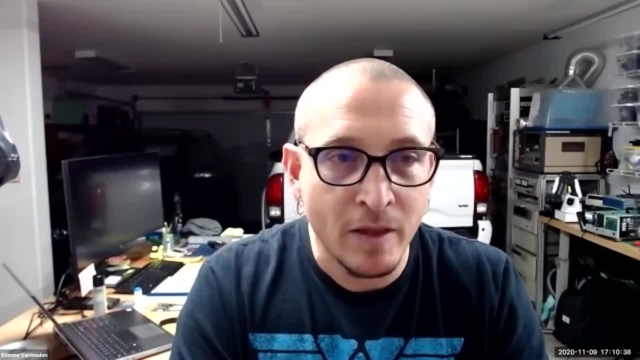 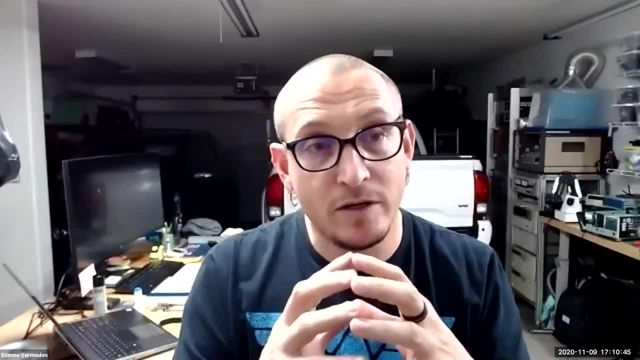 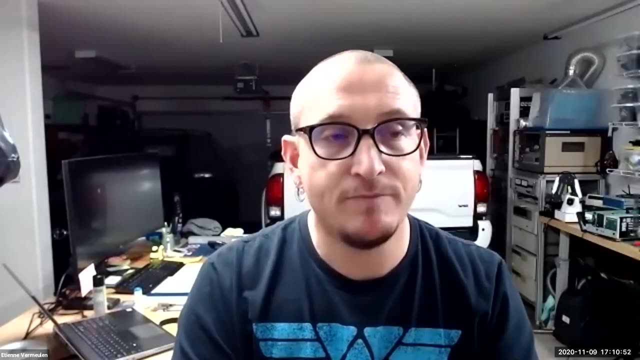 at the same time as you get the Auger dose and of course, that's going to irradiate the rest of the body. now think about it: when you do therapy, you want to use more radioisotope than you typically use for a diagnostic dose, so there may be issues. 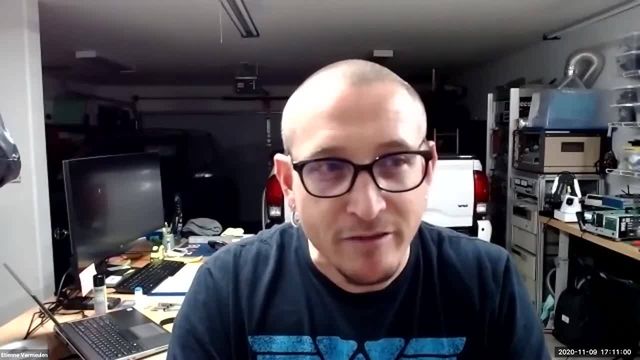 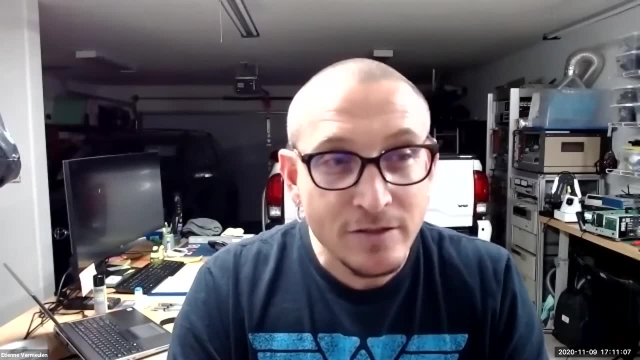 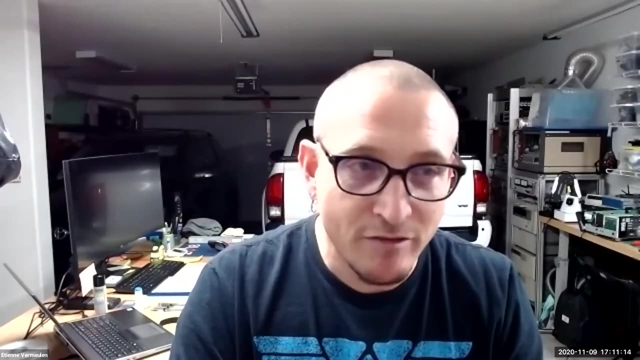 with the residual dose you get from the Turbium 155. if you recall, on that picture I showed you there was Urbium 165 as well, which is really interesting. Urbium 165 is a pure Auger emitter. it's got no gammas so you cannot track it. 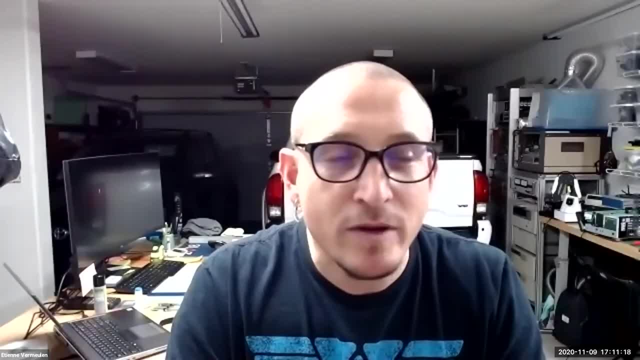 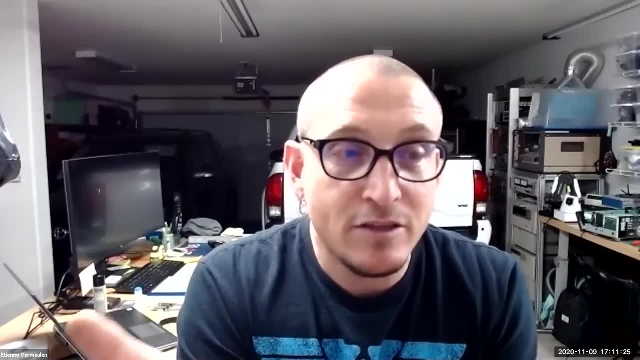 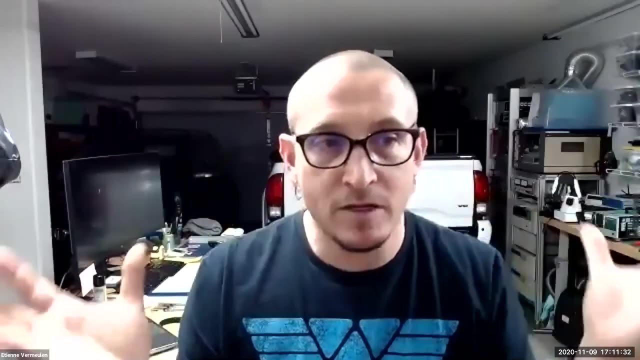 but you have only the dose from the Augers. but I wouldn't discount 155. it may be that turns out that it has such a beneficial Auger effect that you can tolerate the extra dose of the gammas. it's always that balance between how much damage are you doing? 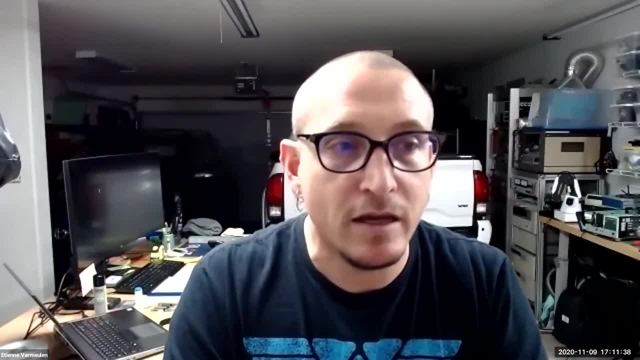 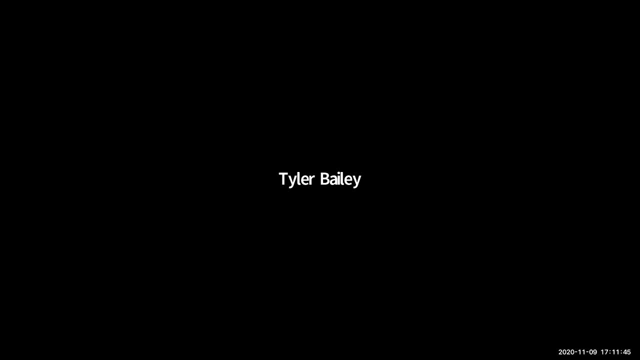 on the outside or the rest of the body and what you need to kill the cancer. I hope that answers your question. well, it's interesting you bring that up because Lutetium 177 is similar. it's a theranostic isotope. you have the beta and the gammas as well. 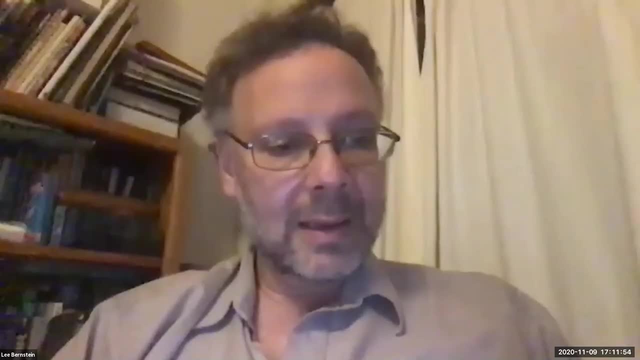 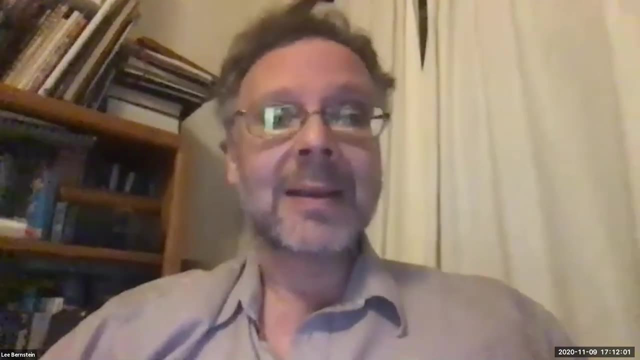 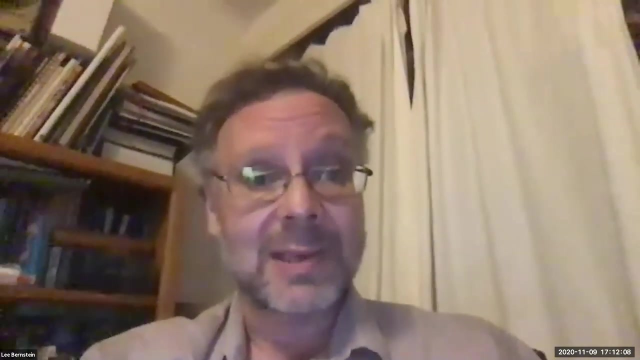 so very interesting. thank you so, Etienne. I wanted to mention that we have also considered the possibility of trying to make 149 by alphas on Europium. but, same as you, there are just also a shortage of facilities that run this sort of higher in energy. than most places would run that have alphas. I should say if you have alphas, acetine is maybe more lower hanging fruit. I think Davis is gearing up to try to do that in some sort of production and Texas A&M are making acetine on purpose. 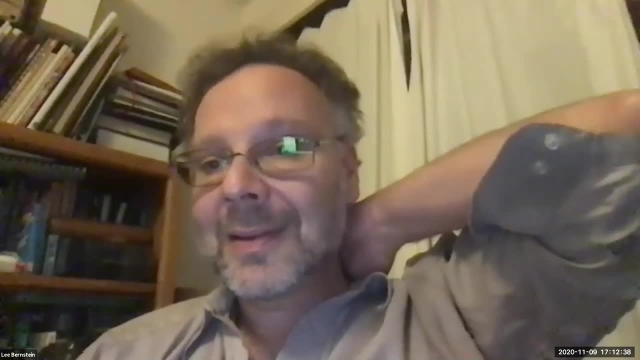 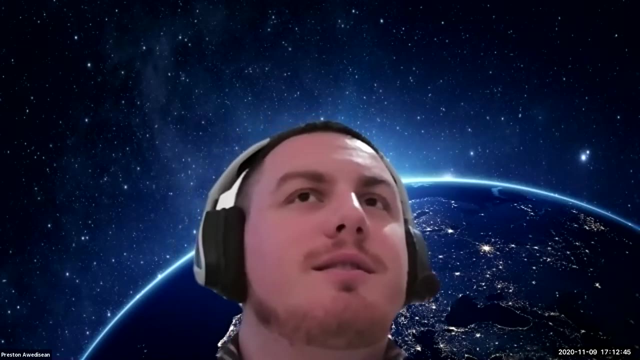 do we have other questions? how much would it cost to make a facility that can handle the necessary energies in the United States for alphas, for the higher energies, like at CERN? do we just keep building bigger and bigger cyclotrons and just see what we can do with it? 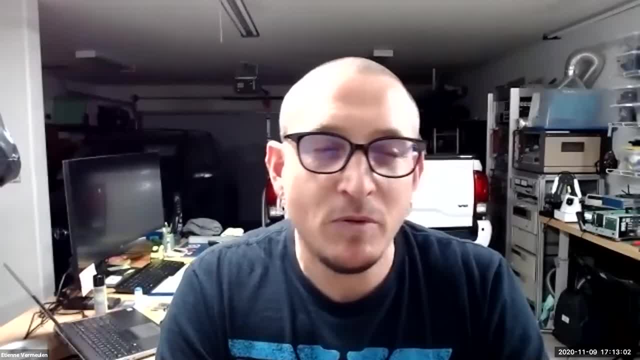 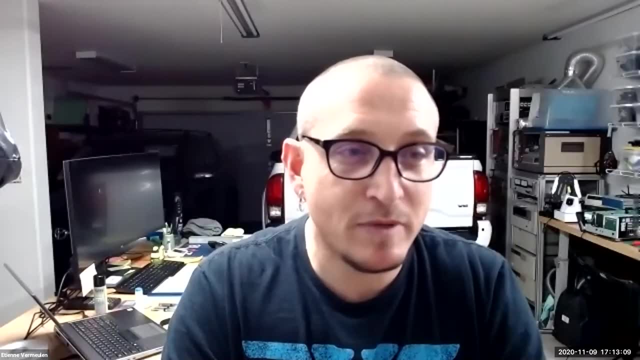 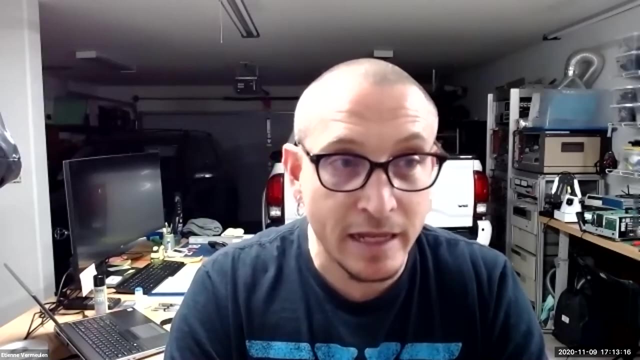 how to check out. I don't think people will build accelerators specifically to make terbium 149. it will always be an ancillary facility. so at LANS, in principle we could make terbium 149 if we change the end of the accelerator. 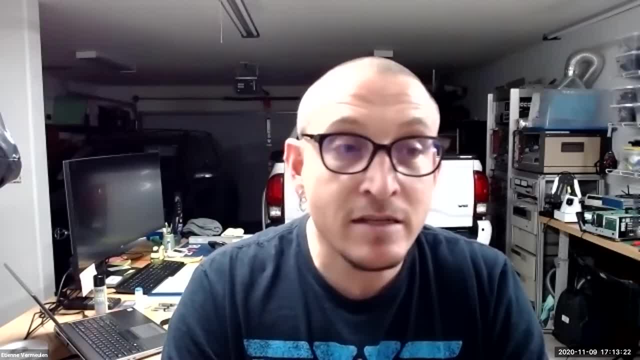 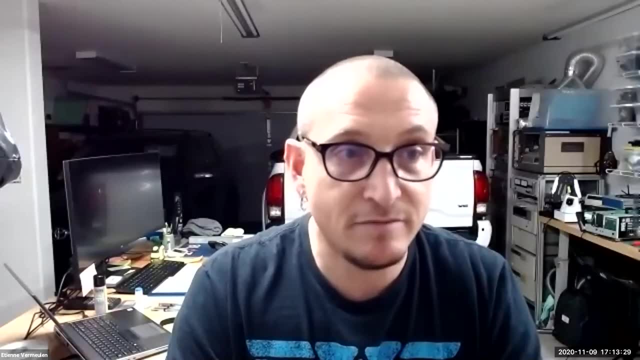 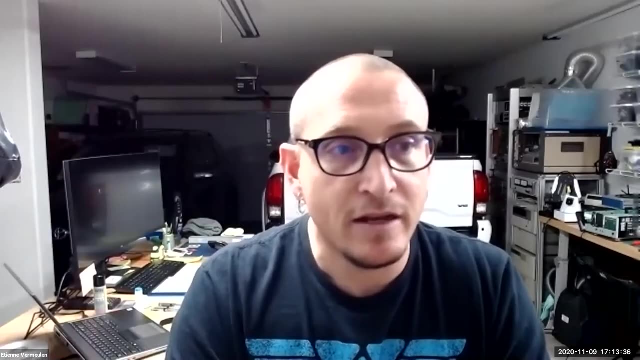 so our accelerator goes up to 800 MeV. that is enough to make terbium 149. right now there is no facility at the end that allows us to do that. we actually used to have a facility down there and one of the plans that they are thinking of. 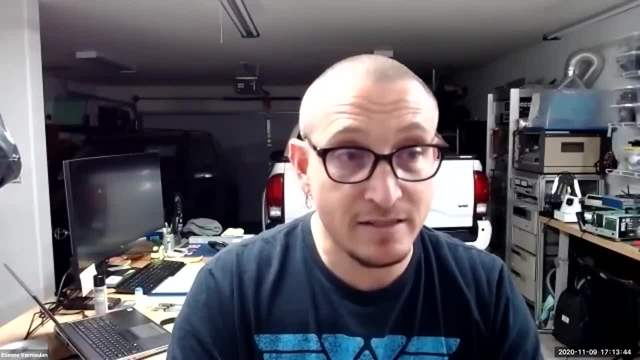 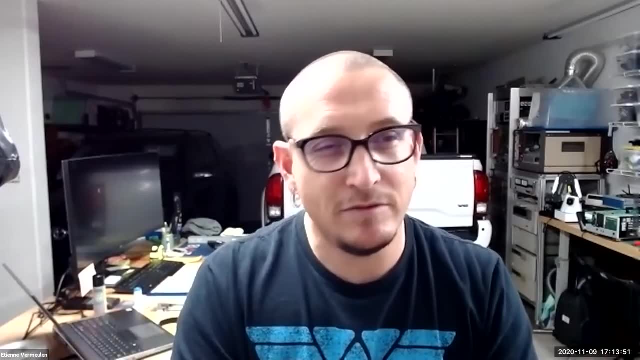 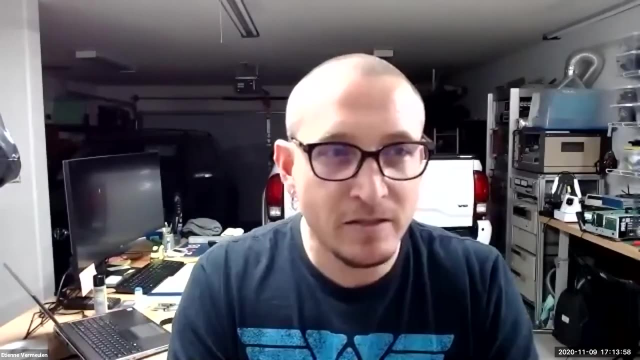 at LANS, because people are always trying to think about new things- is to make a spallation facility like that that will create a bunch of these isotopes, so essentially an isole facility, and then you could possibly do terbium 149 there. what that is going to cost. 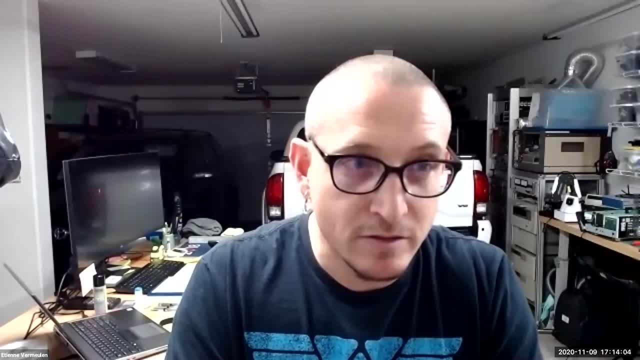 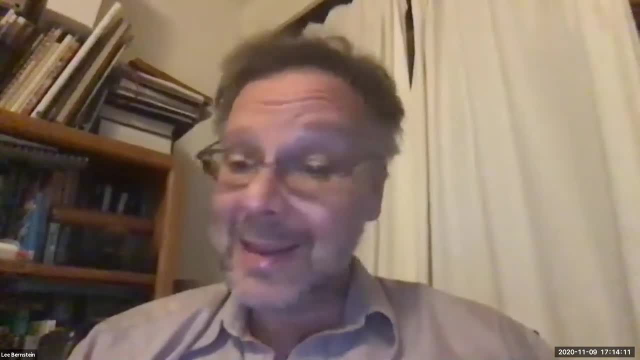 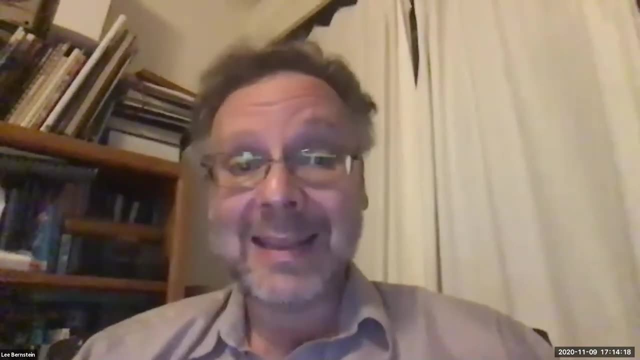 in the tens of millions of dollars if you had to build a facility from scratch. you are probably looking for something, but then again, this is an extremely worthwhile and inspiring activity. I think you can find terbium 149 is even more interesting when we made it. 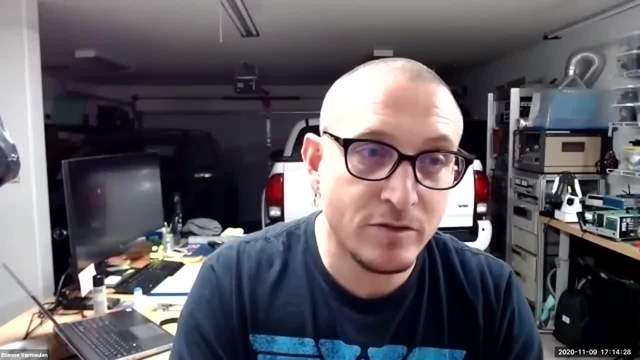 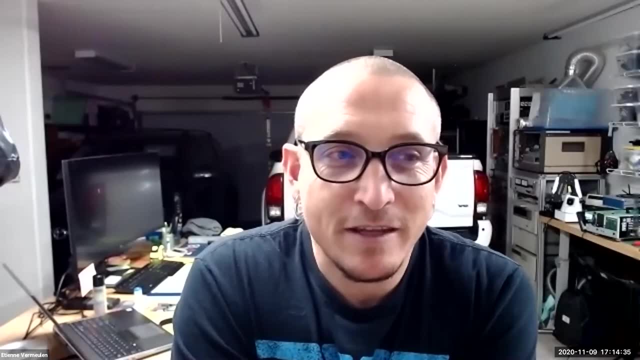 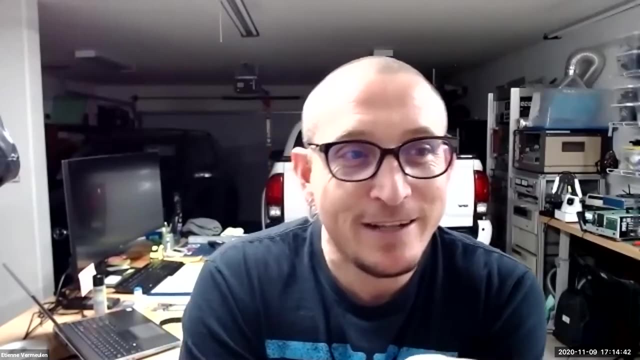 we used it for therapy tests. we used it to image with PET. in principle you could also image it with SPECT. there are emissions of 149. that may just work, and we tried and unfortunately our SPECT camera failed halfway through the experiment. so we did see a little. 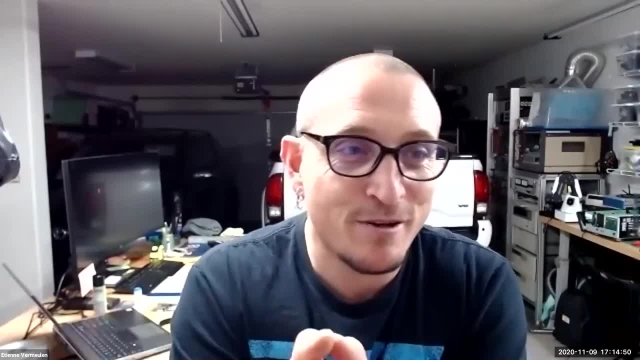 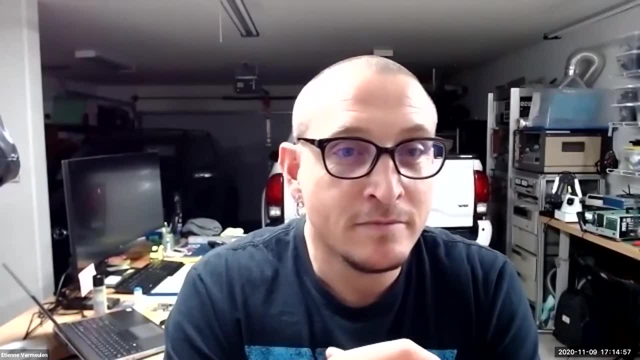 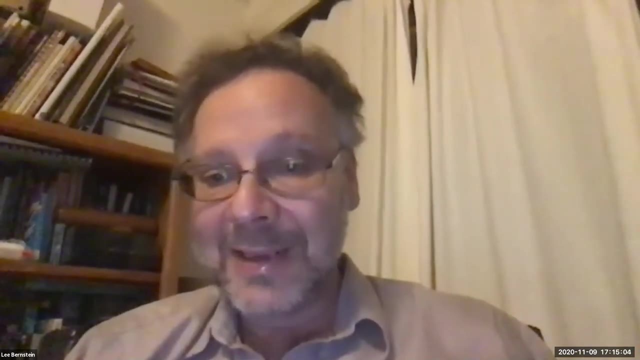 interesting emission. we thought we saw an image and then we just couldn't confirm it, but it may be the one isotope that can do everything. So, Etienne, I just want to share a couple of the comments from the chat. Sasha said this was an absolutely amazing presentation. 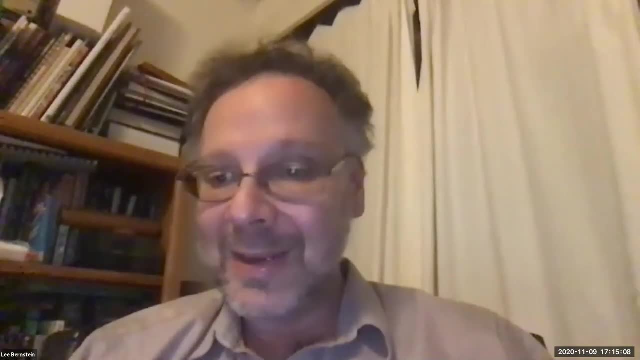 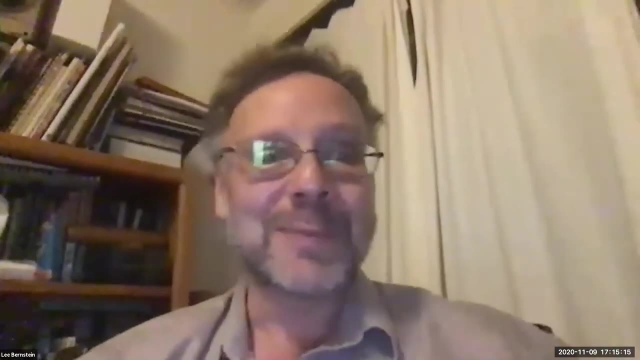 thank you. I think we are going to have more like this. so many people really appreciated this. I just want to let you know that I don't know if you are looking at the chat- you probably shouldn't be, since you are answering questions, but really, people have been very 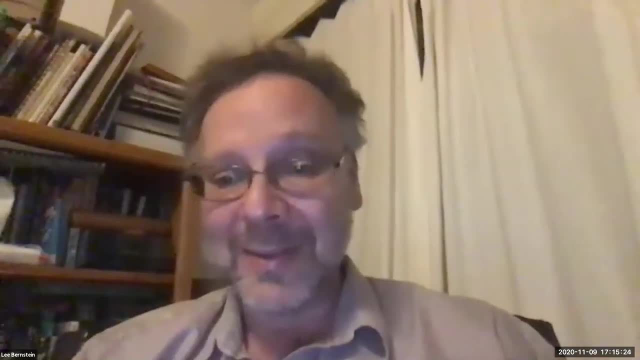 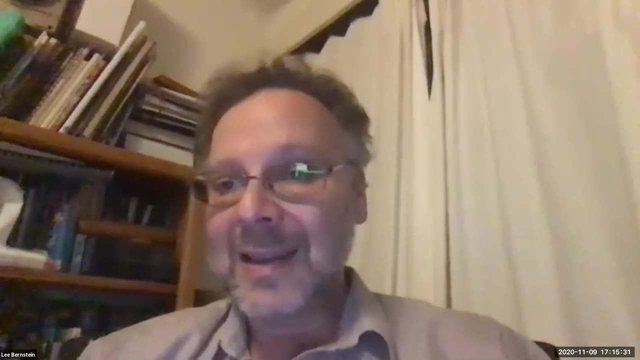 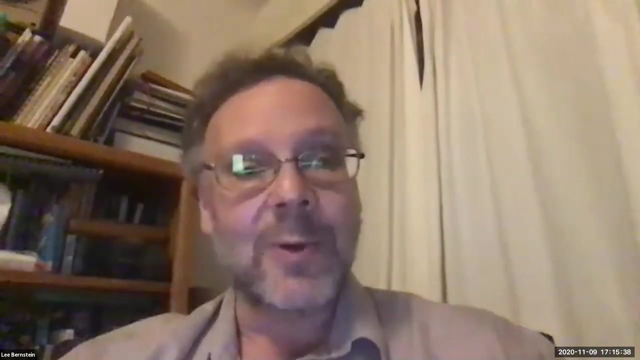 enthusiastic about this. Carla said the same thing also. by the way, she works with Rebecca's group. are there other questions? there is one other request, and I am going to add my name to this as well. you said that you had an LAUR number. are you willing to share the presentation? 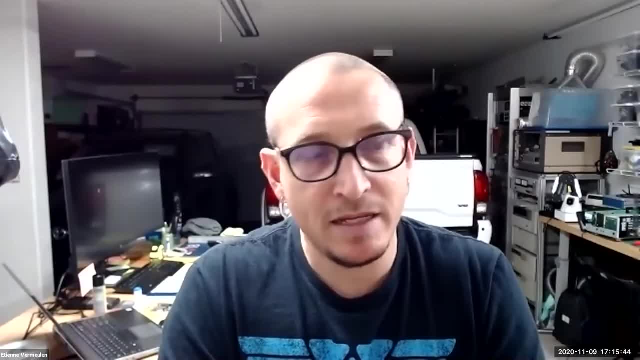 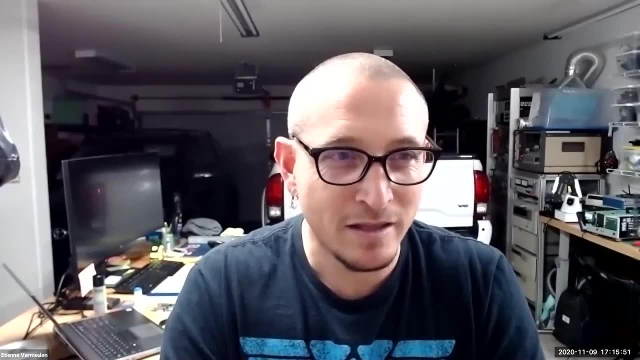 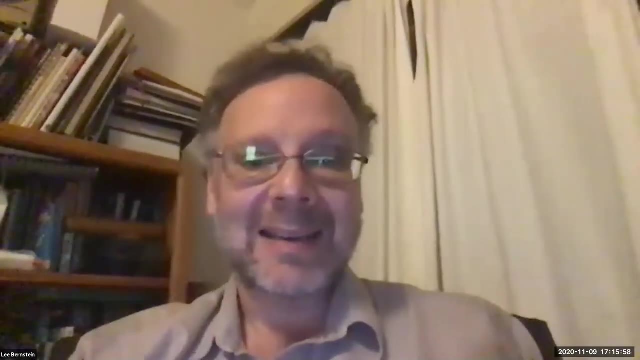 Etienne, Yes, I can share this presentation. it is difficult with the videos, so I am happy to share them separately because they are huge. the presentation is 172 MB, but I can make a PDF for you. that would be fantastic. I think that everyone would love to see it. 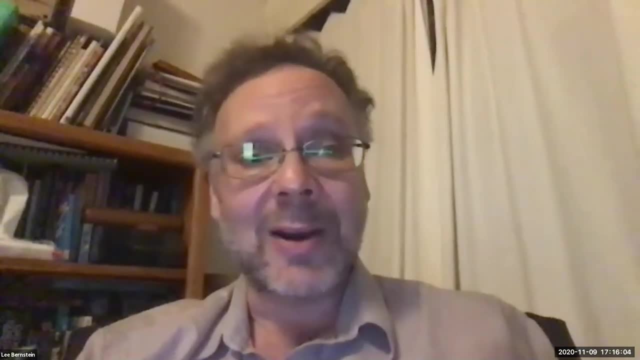 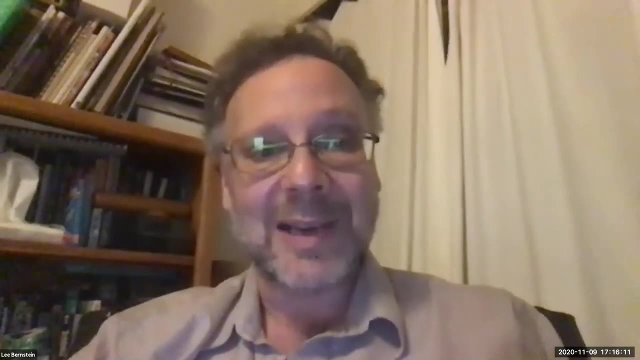 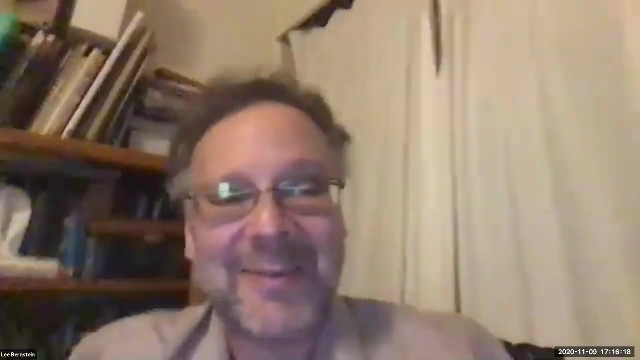 and I am going to do a little bit of gratuitous advertisement here. we are always looking for good students. we have a number of them already with us, but if you do have questions about isotope production and you get to work with really cool people like this, 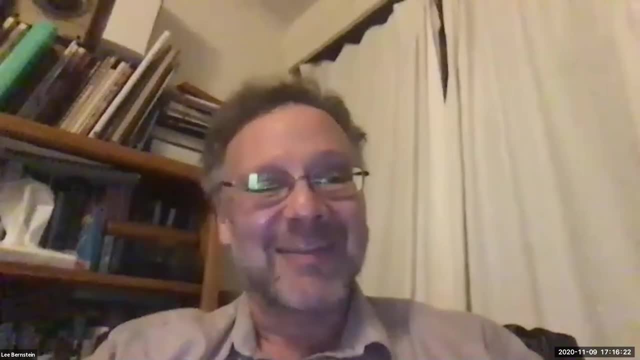 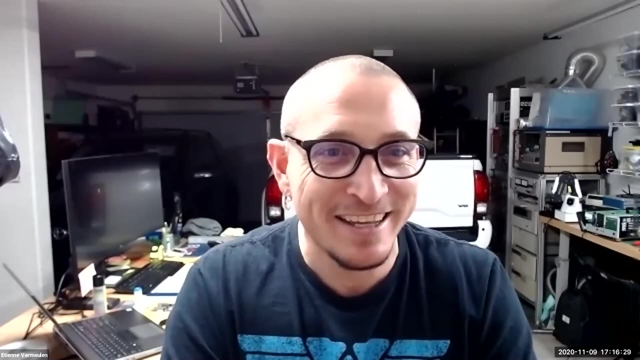 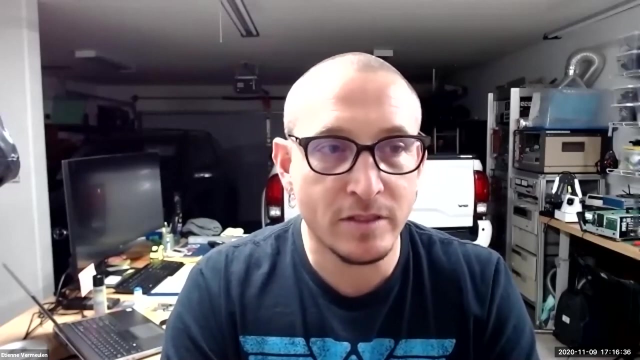 who also have got interesting garages with things in there. I am making Rebecca laugh. I am happy to share stories ten times because John has probably heard my stories ten times already. so I do believe we have a call tomorrow to talk more about career opportunities, so I will be there.